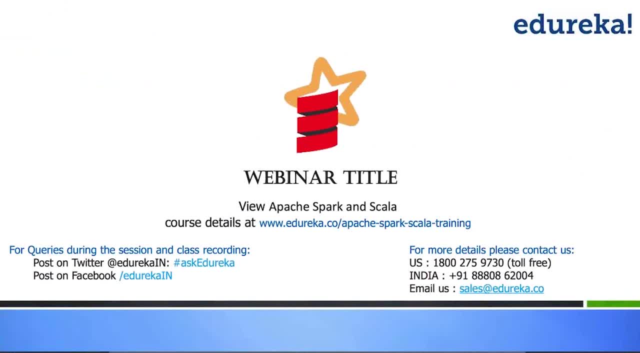 Guys, my name is Vishal, as you know by now. I'm having overall industry experience of almost like 9 years now, and since last 5 and a half years I'm working in this big data domain. By accident, that was how I started in this domain. 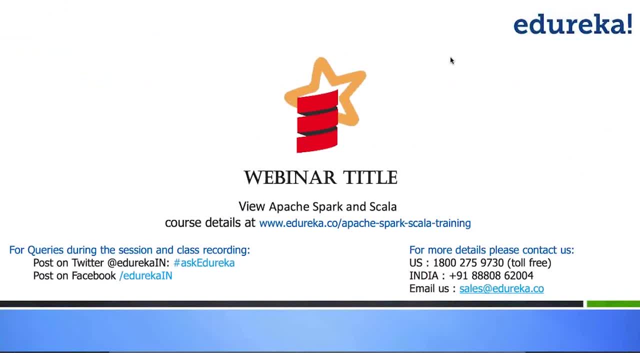 I was a part of a startup. we started doing the things and it just went forward And, just like you, many of the other guys who are just starting in Big Data Domain, I started my journey in Hadoop world. I have spent quite a lot of time into that and then eventually now, if you say, what are you doing right now? 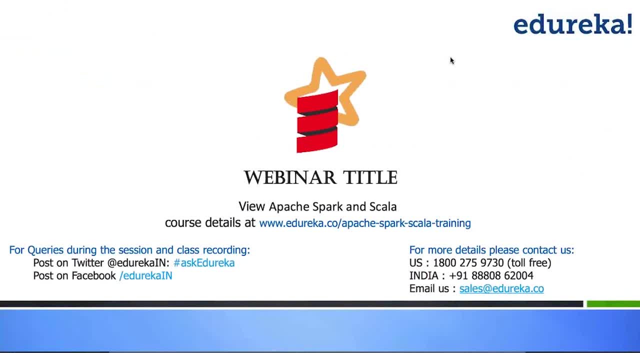 So my specialization at this point of time is the integration of the enterprise systems with the Big Data Analytics systems, Typically, or so called, near real time processing of the systems, And sometimes we even refer it as lambda architectures. So I find myself doing those kind of implementations more often than not. 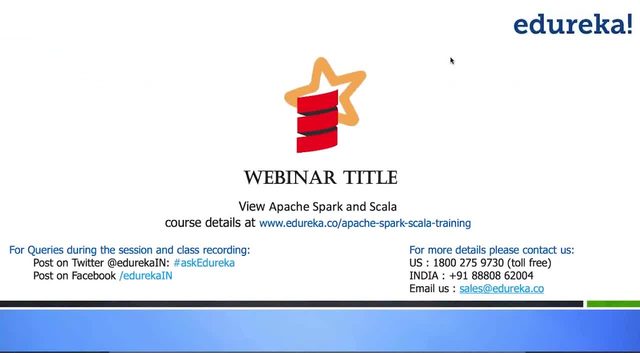 That's pretty much from the technical side, I would say, And from the domain's perspective, it has primarily been into the area of, you know, completely into the area of banking and a bit into the, you know that retailing thing. 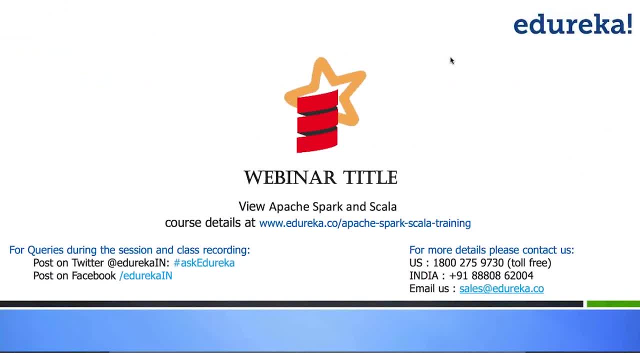 So they are the main areas. And then there were a few projects for telecom and banking- sorry, telecom and healthcare, and all which are like very much negligible as compared to these two domains, banking and retail. So well, I think that's. let me just keep it that short. 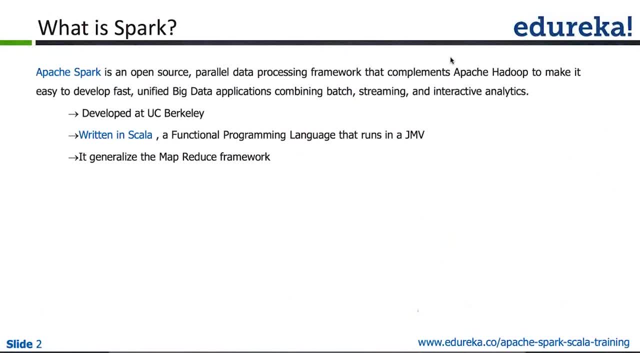 You know more about the experiences and all. we'll always keep exploring, as in when you know, we decide to meet in course and other stuff. So let me just tell you the objective which we have. So let me just tell you the objective which we have. 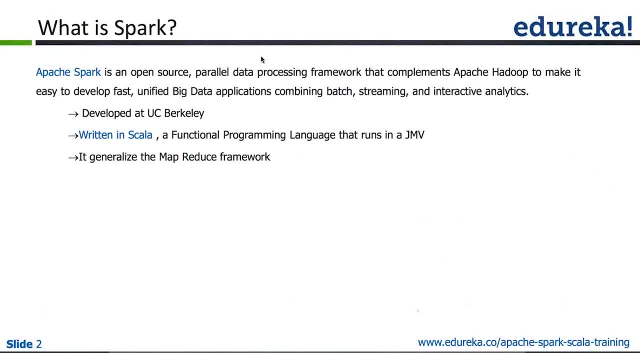 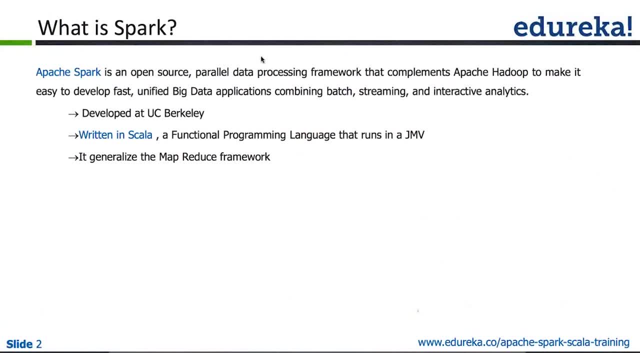 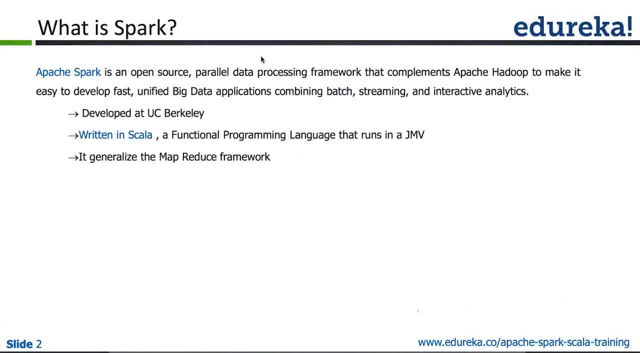 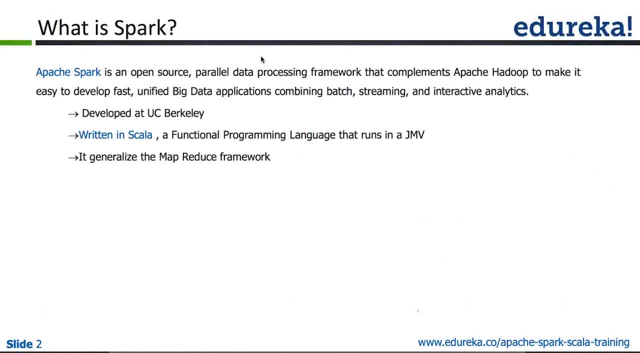 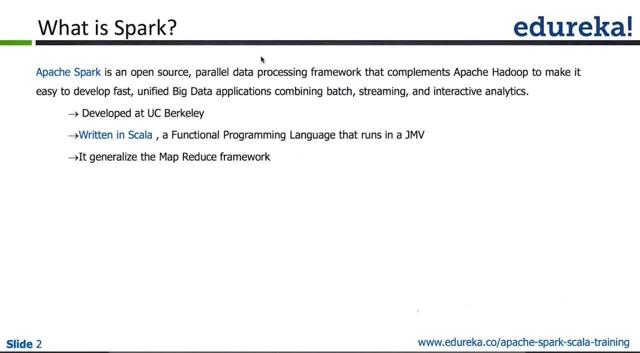 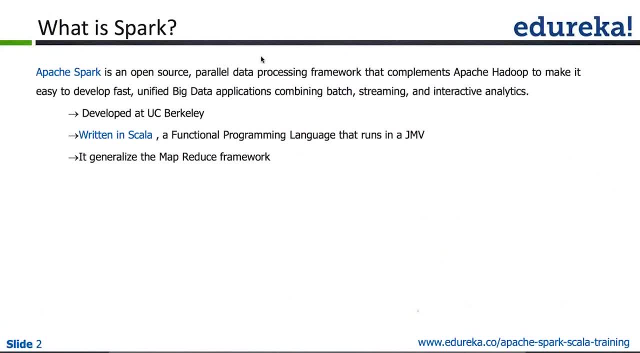 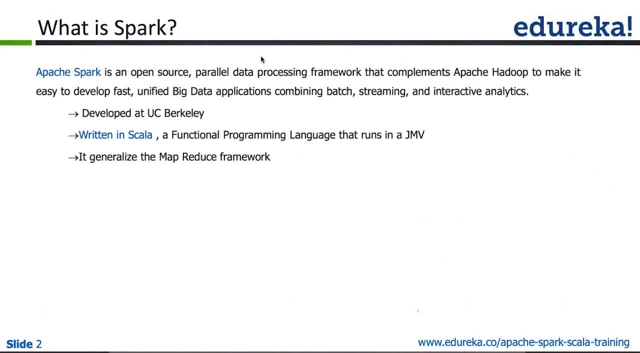 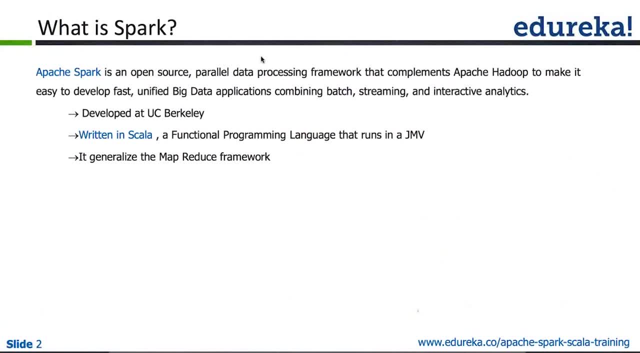 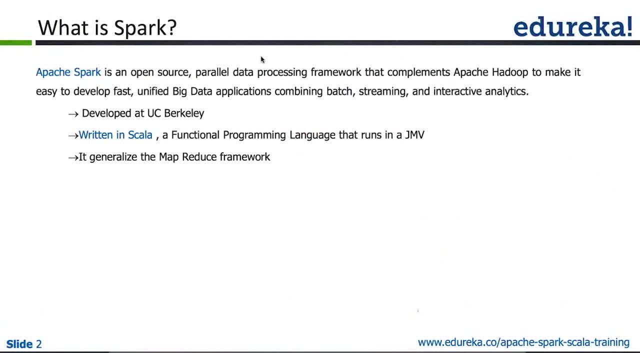 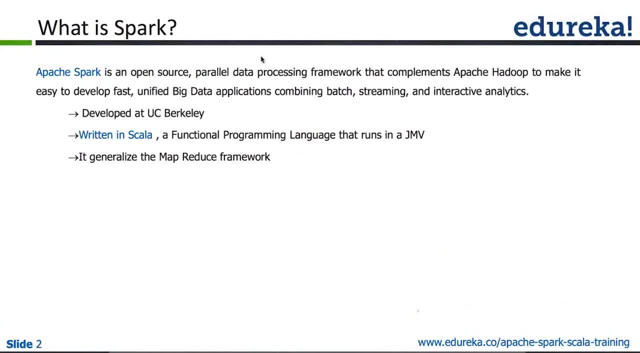 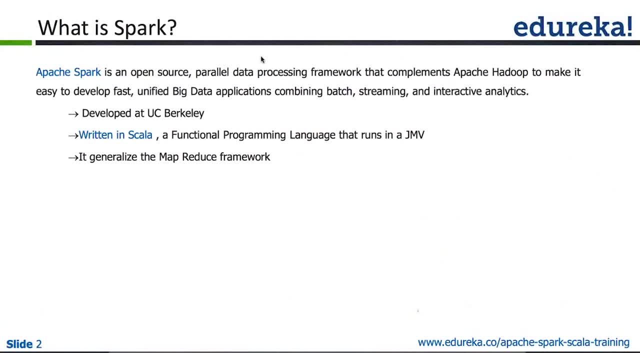 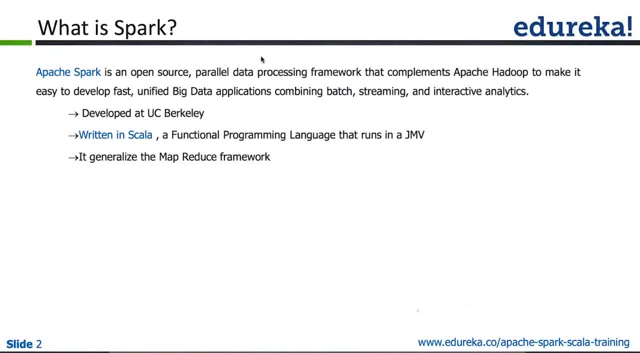 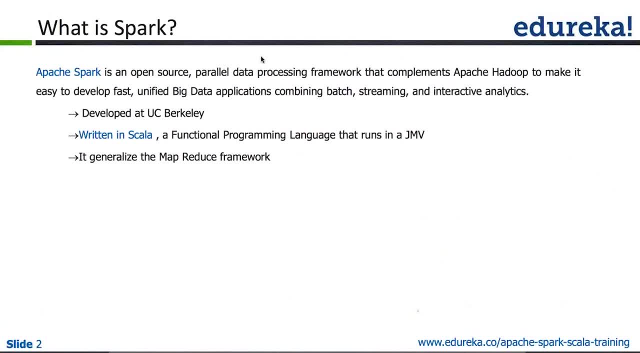 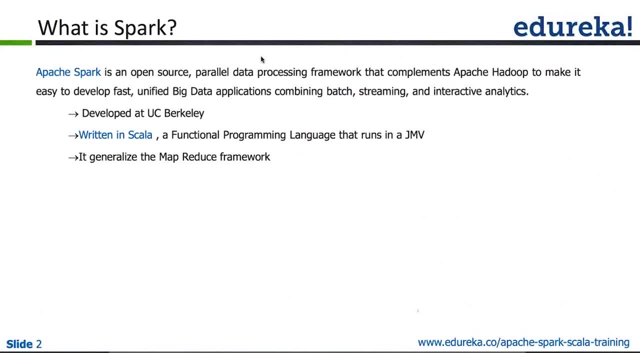 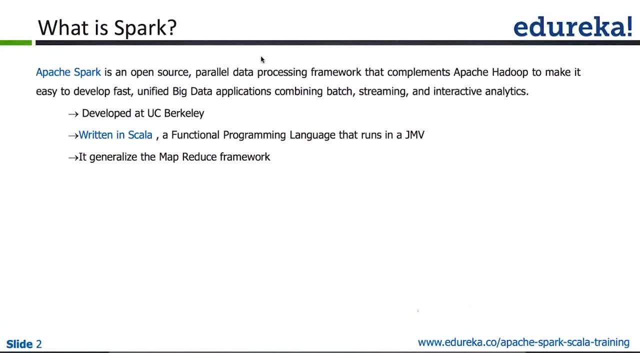 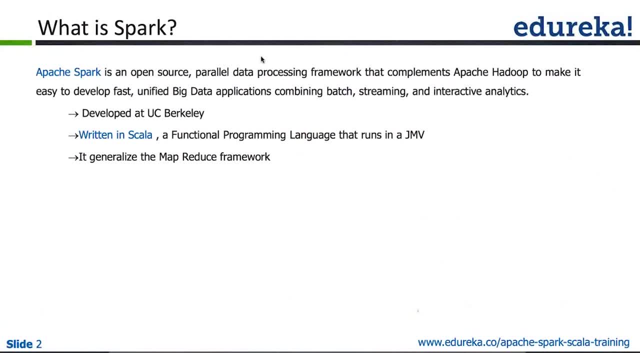 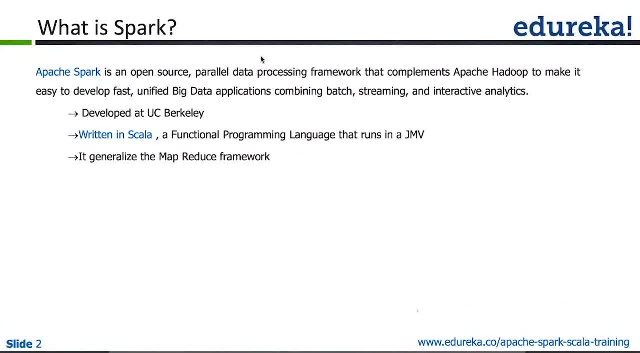 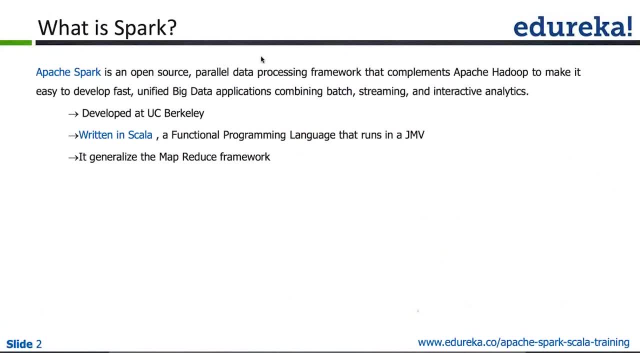 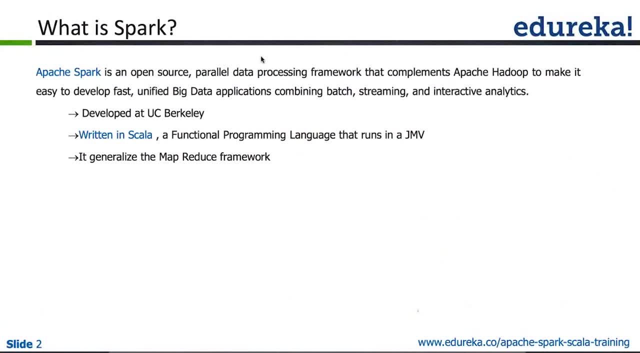 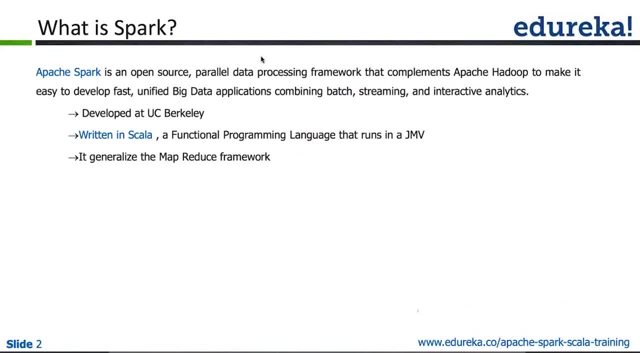 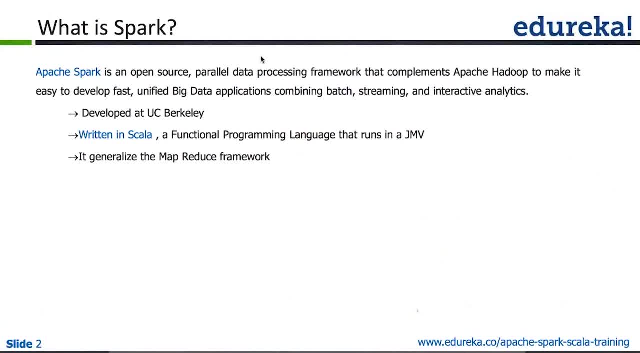 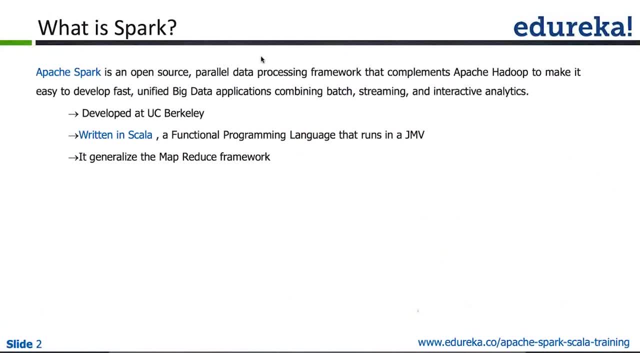 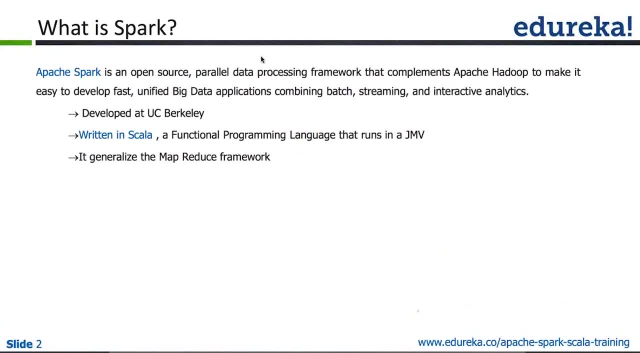 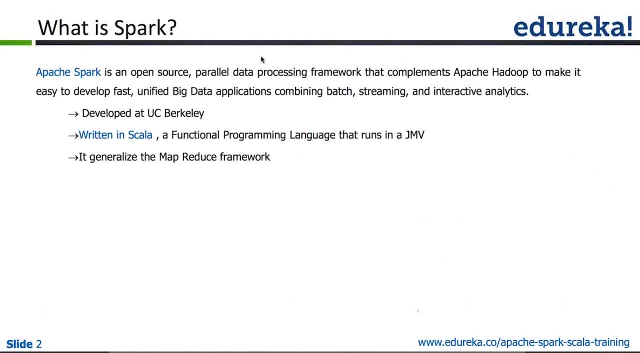 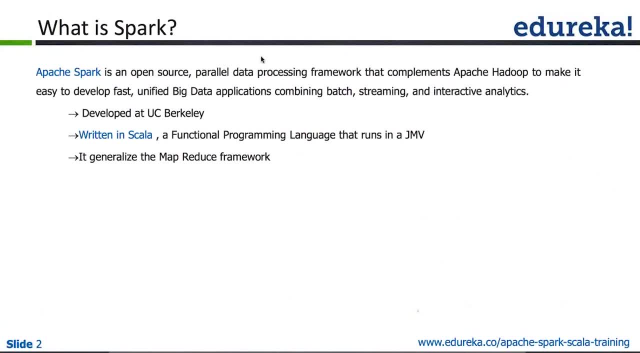 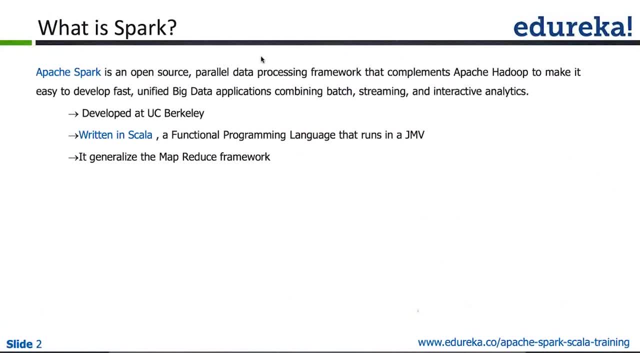 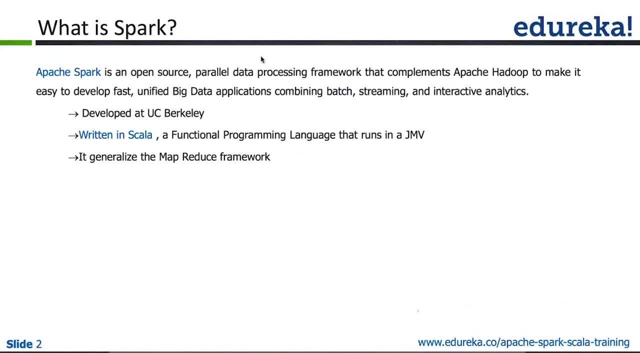 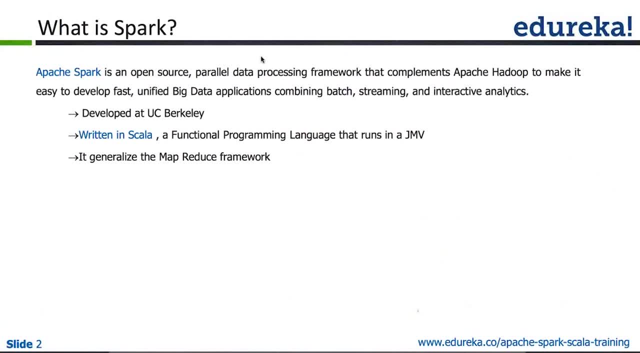 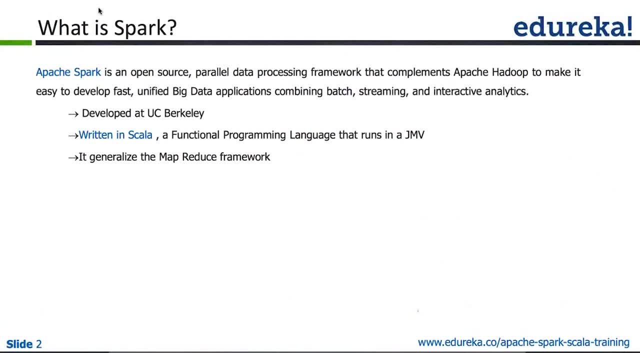 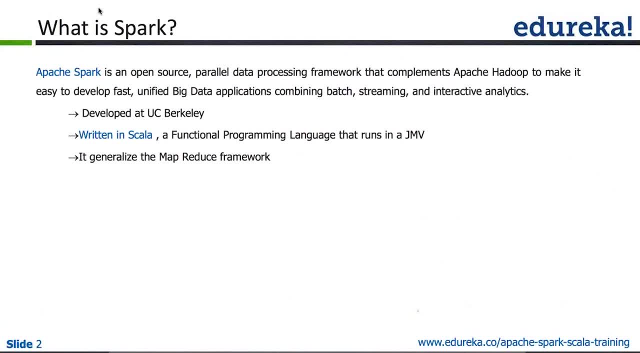 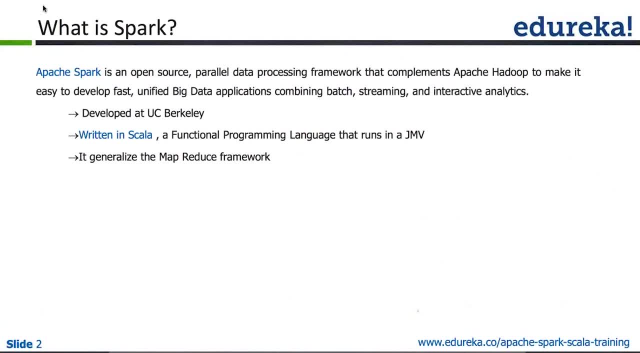 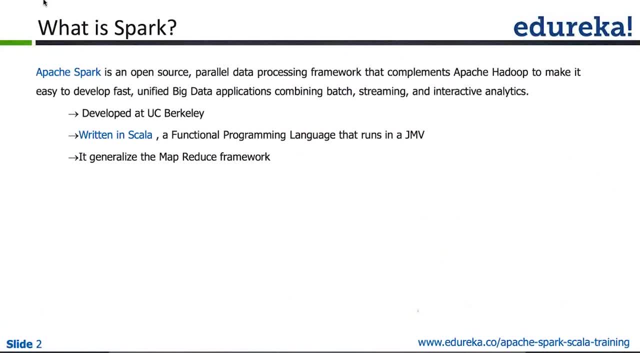 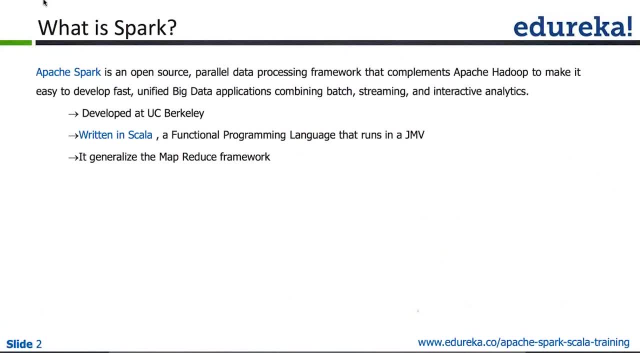 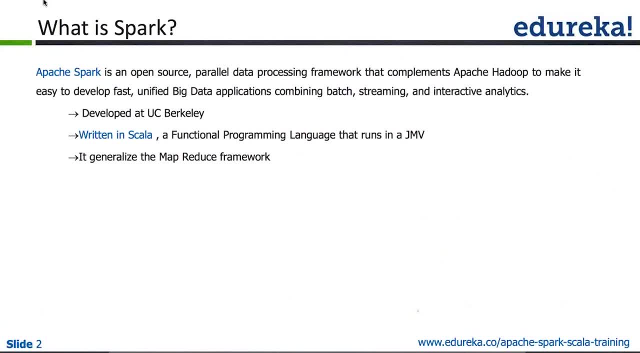 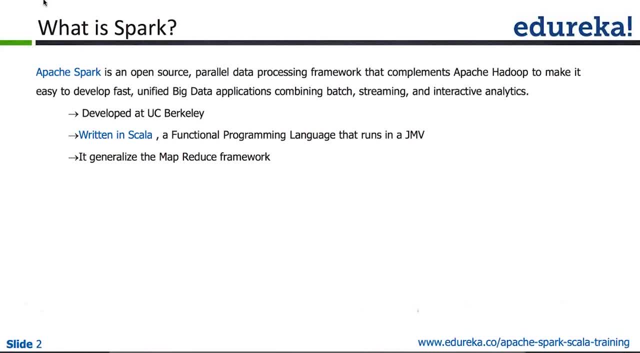 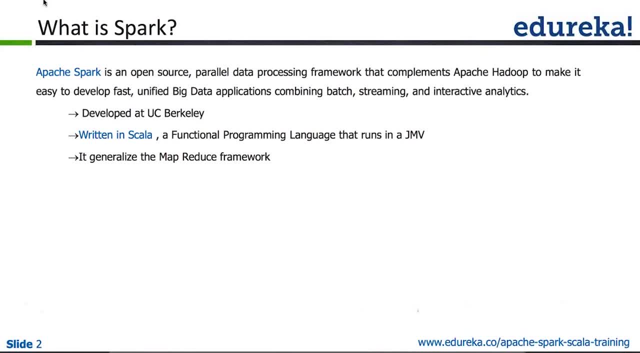 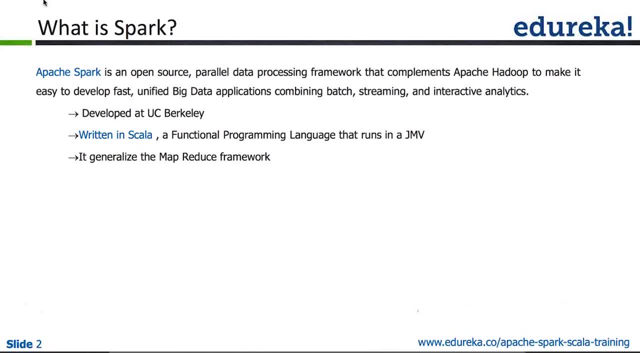 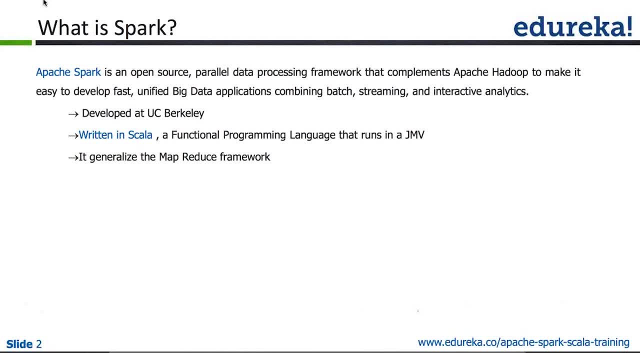 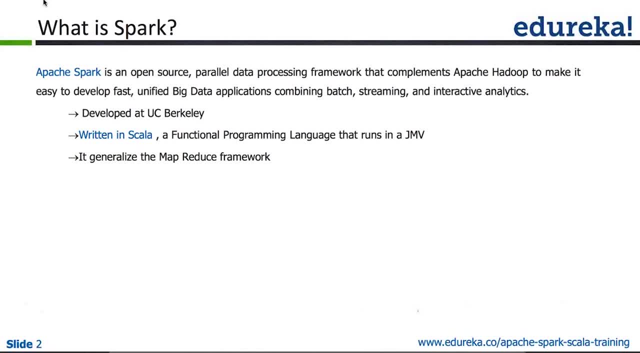 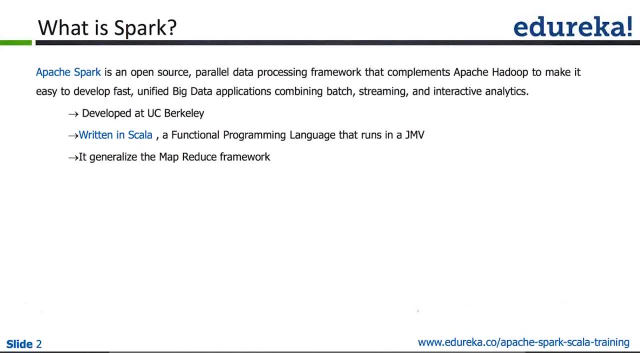 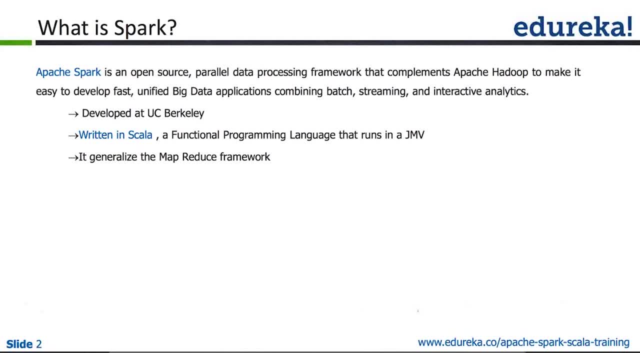 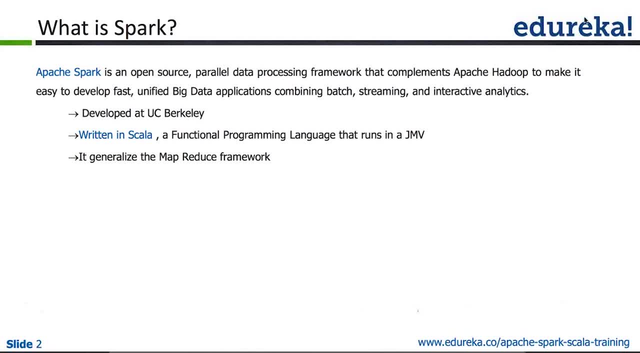 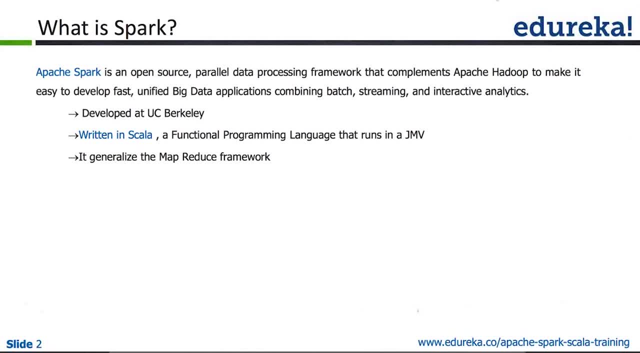 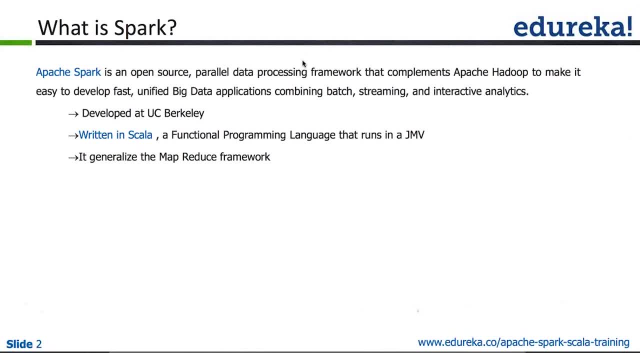 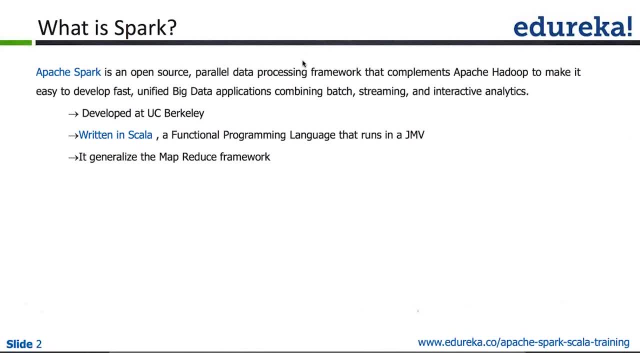 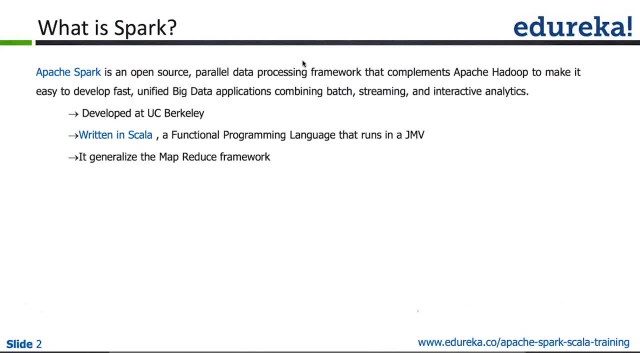 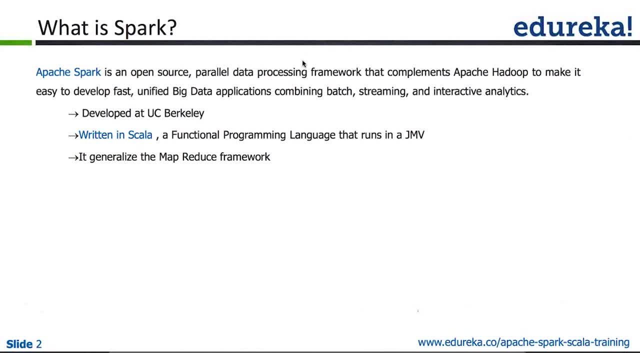 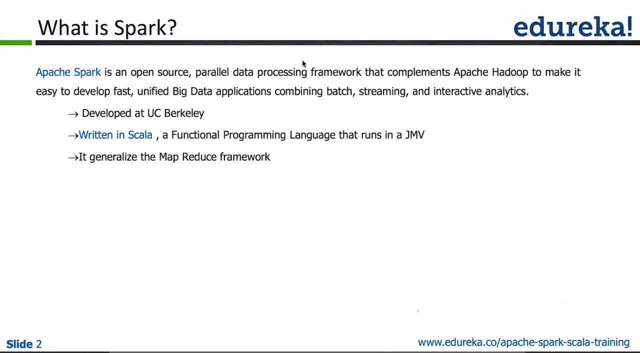 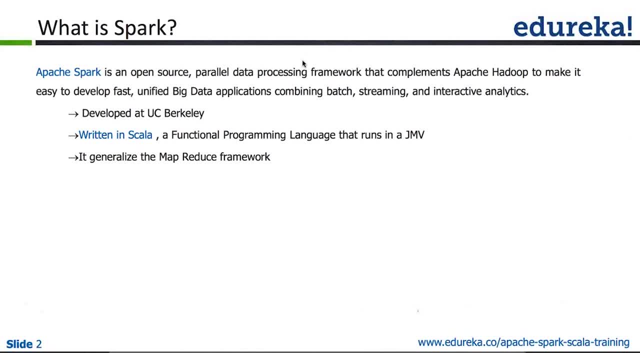 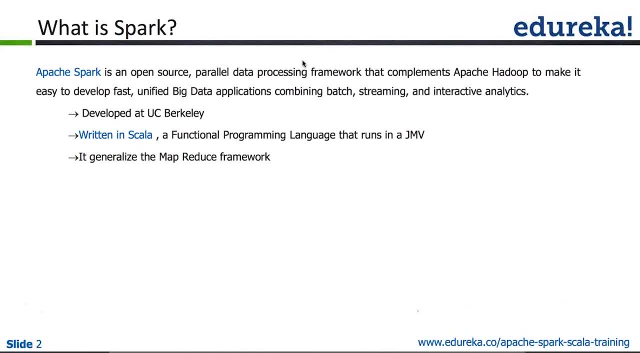 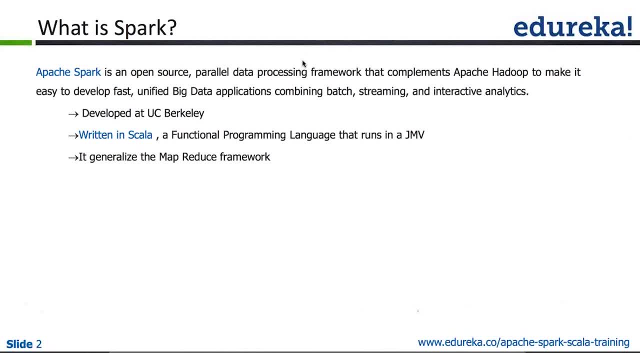 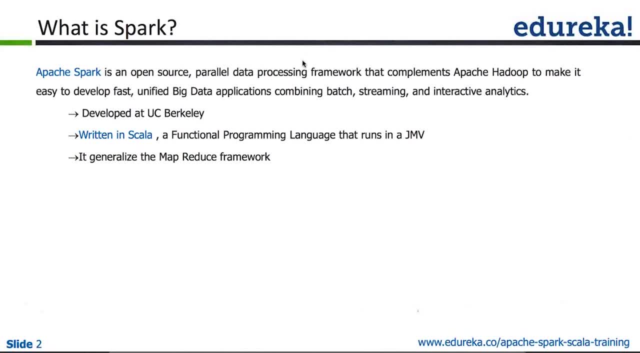 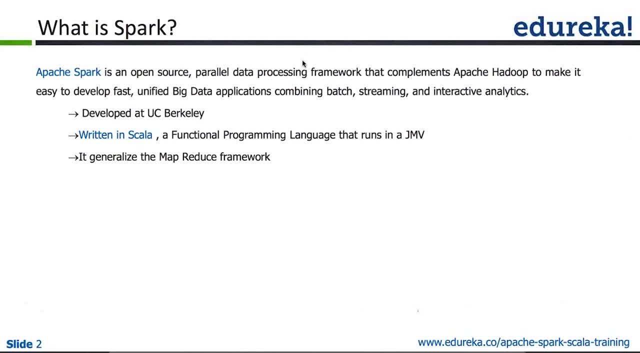 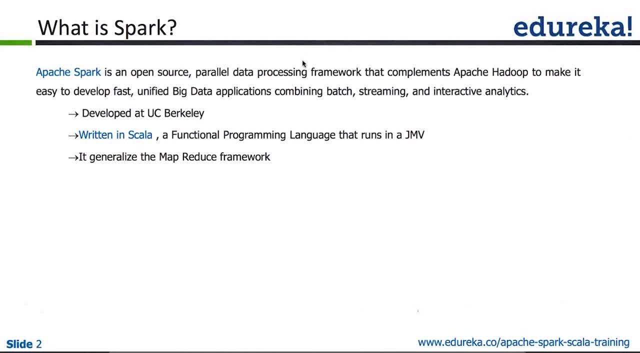 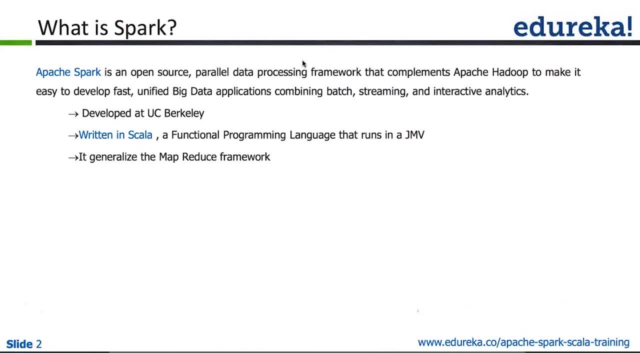 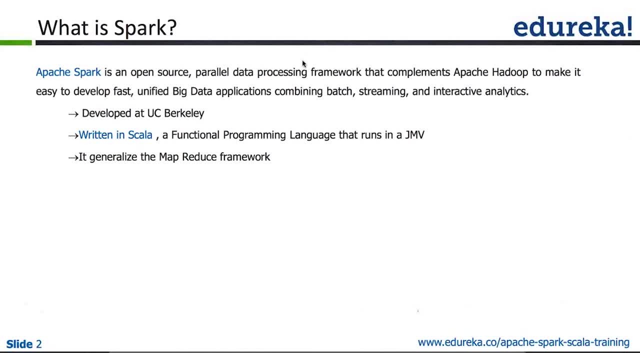 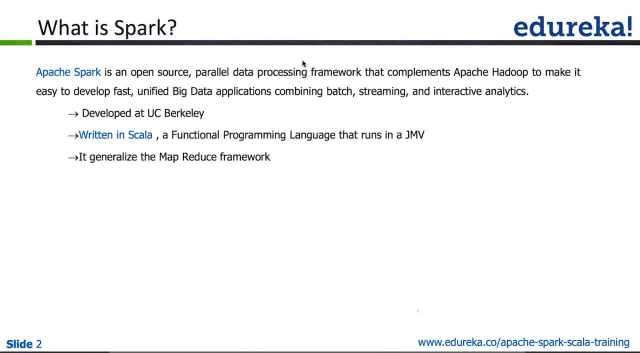 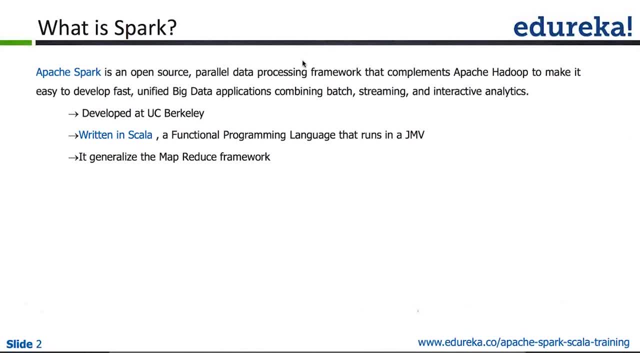 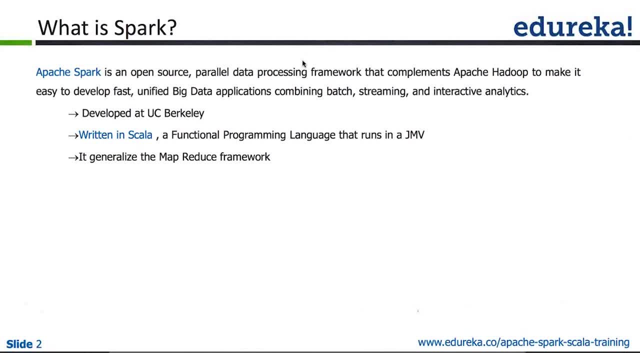 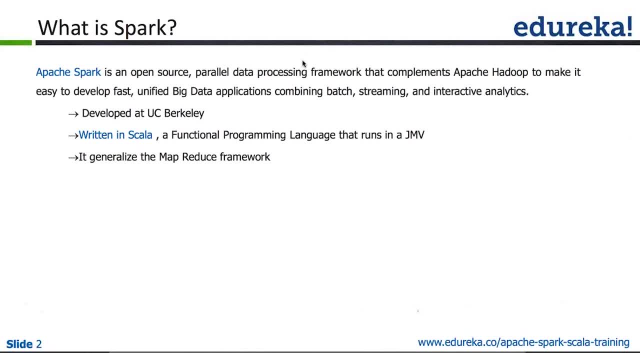 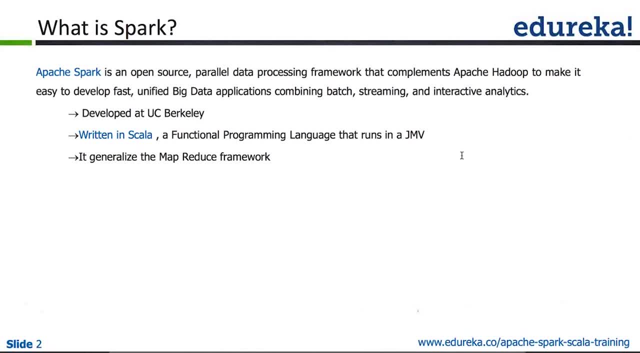 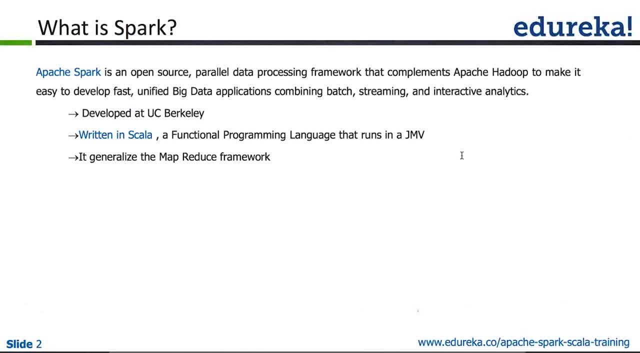 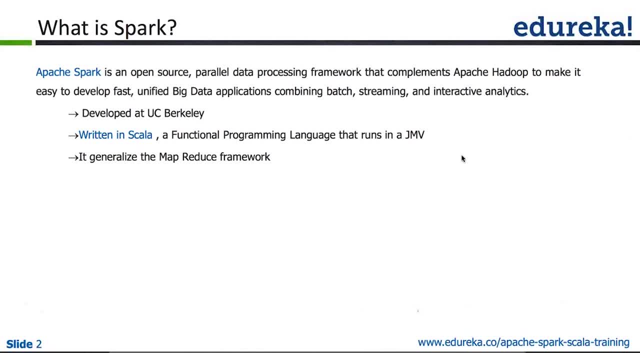 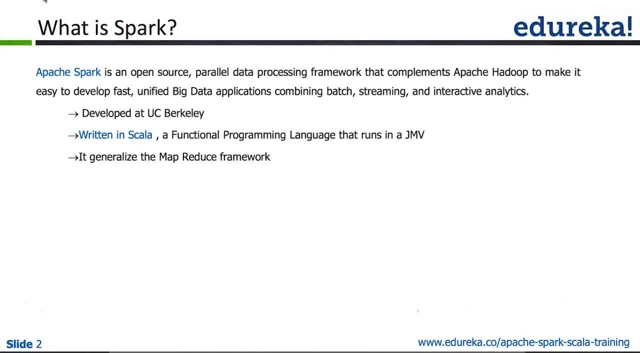 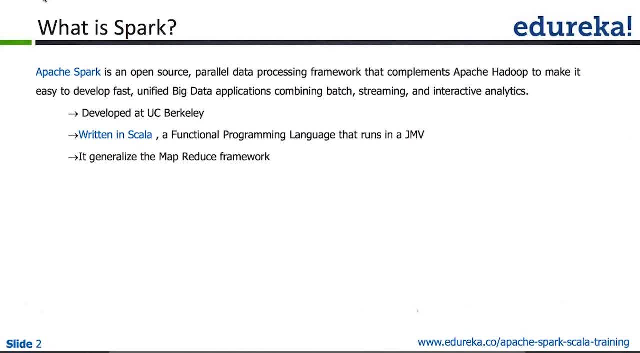 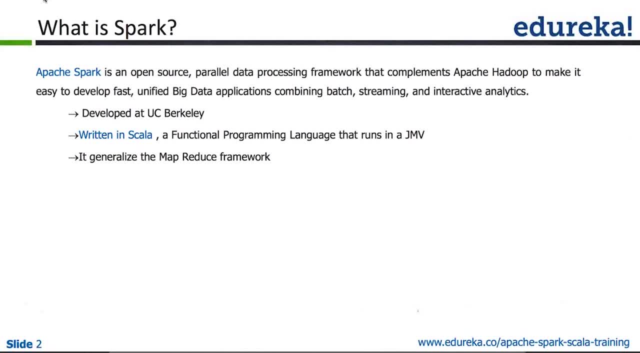 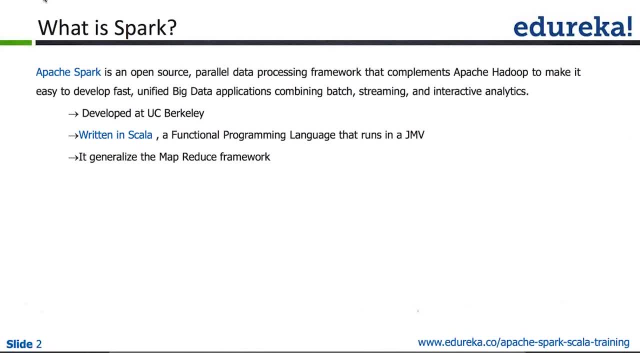 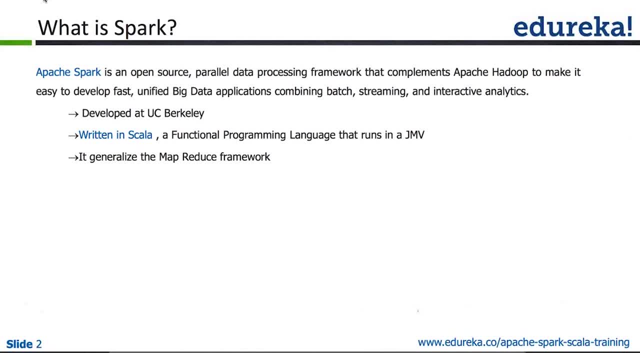 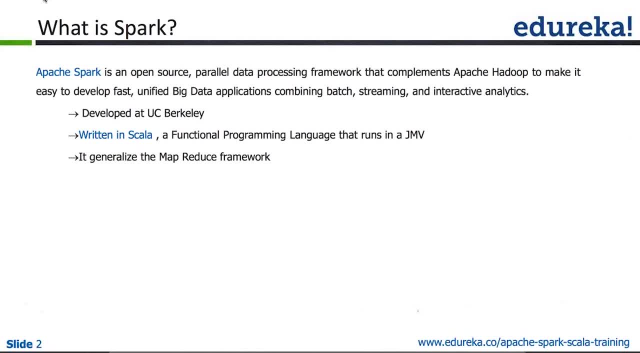 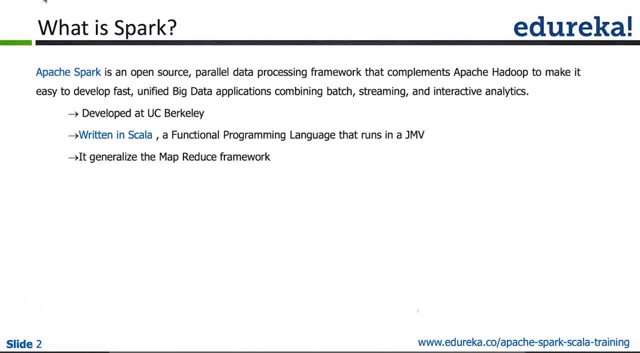 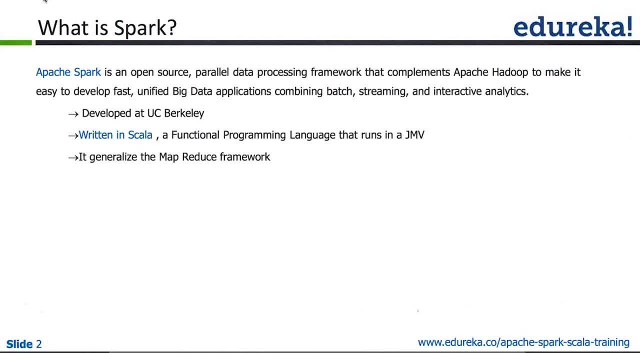 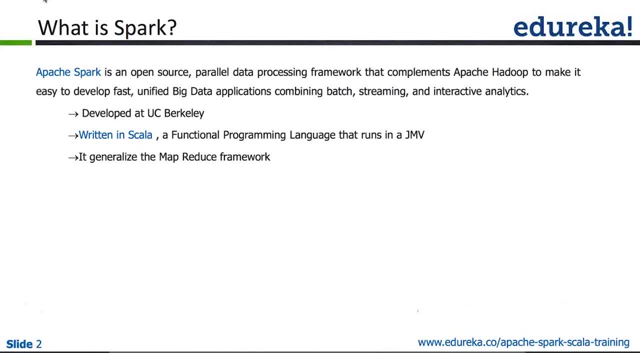 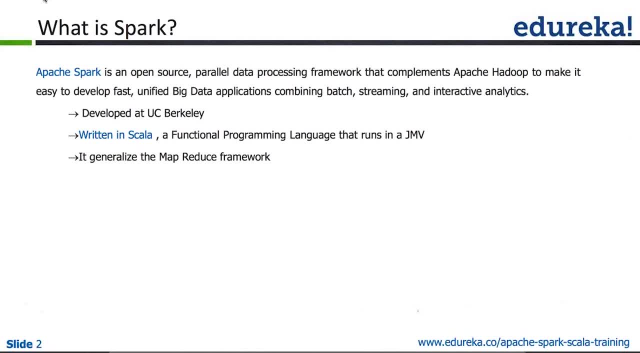 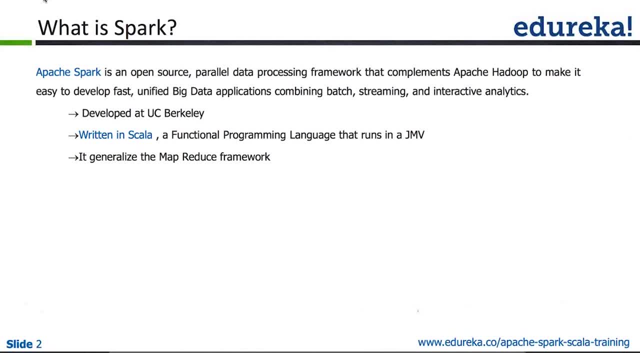 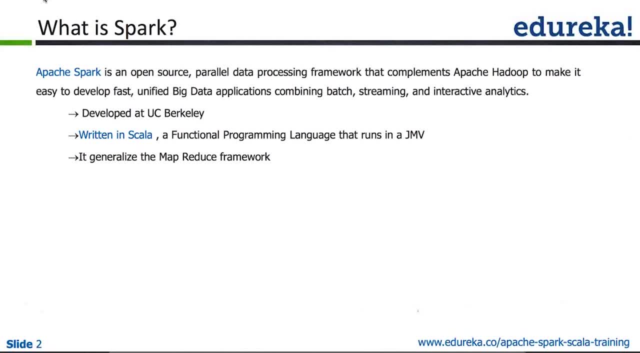 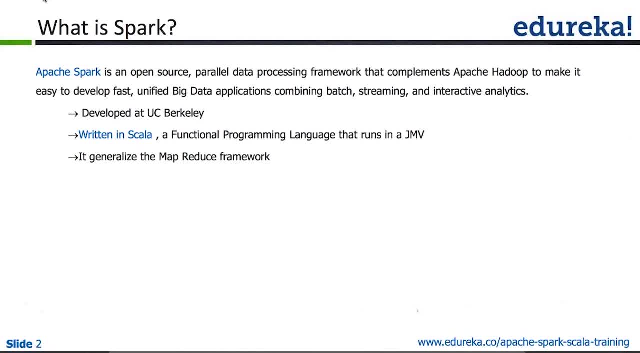 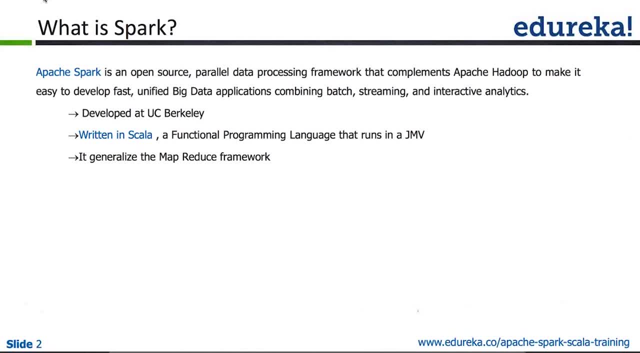 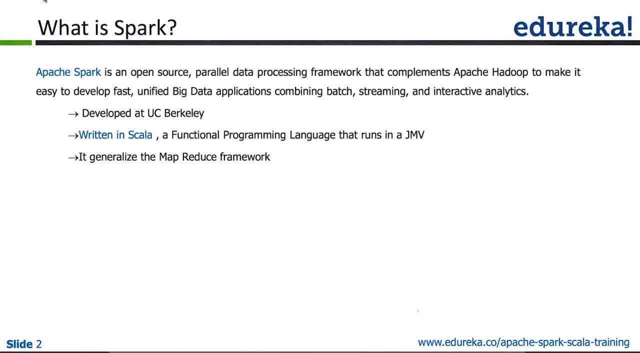 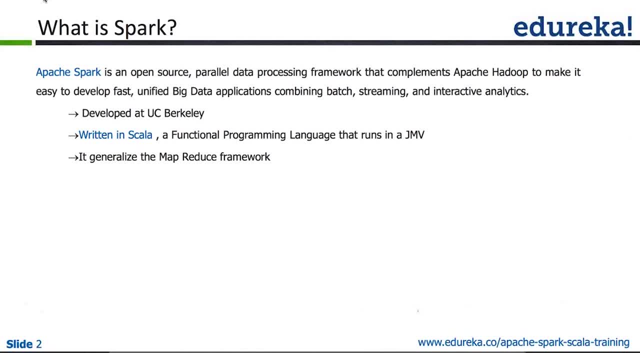 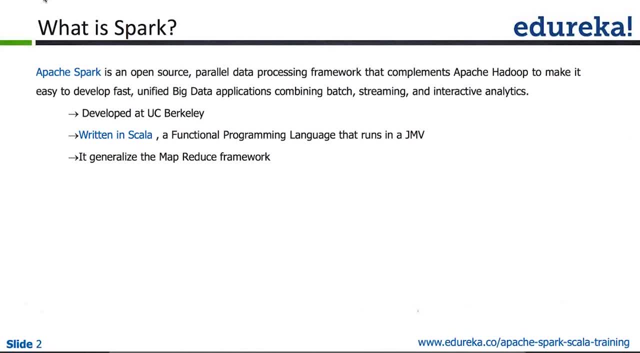 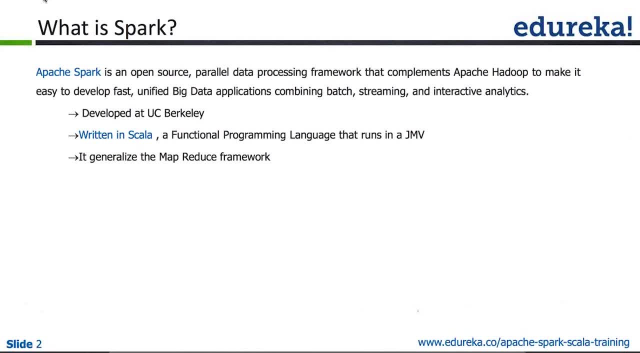 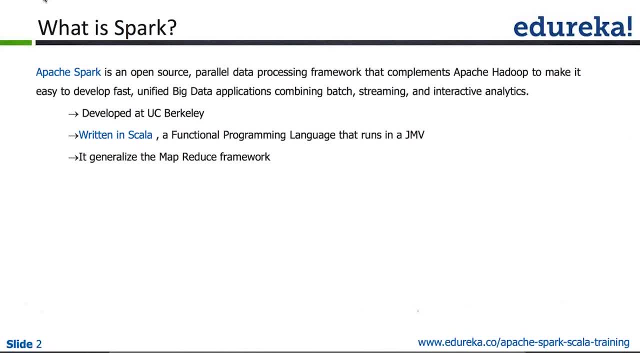 So let me just tell you the objective which we have- Spark is written in Scala- the best advantages or some of the reasons why it has gone Scala way, because over the period of time when the big data systems were being evolved, people really found that the kind. 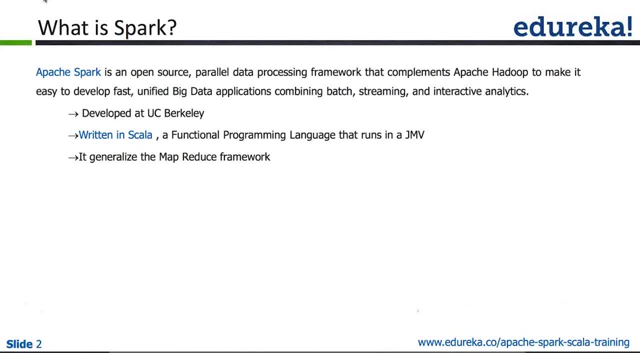 of problems which they are trying to solve are really functional in nature rather than object oriented in nature. So you know, right up to Java 7 does not really support any functional programming. the functional programming support and all has come from Java 8.. 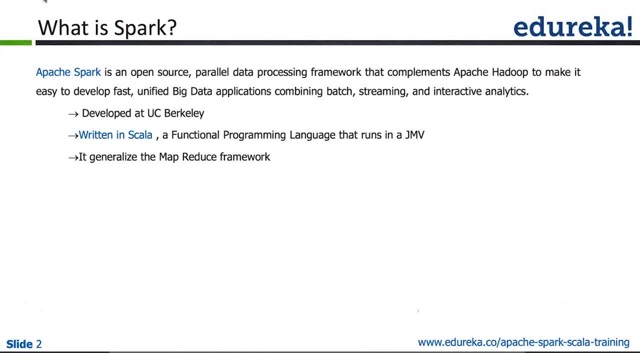 So you will see very soon. Spark even supports Java 8 also. You can do the very same thing in Java 7, but they will be really painful. but yes, right, the support is available for Java also, but the entire source code of Spark is in Scala. 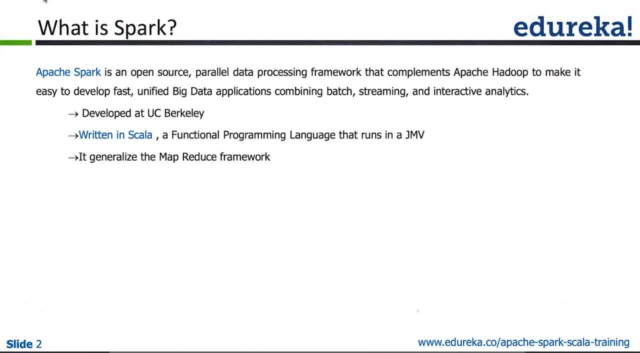 and it generalizes the MapReduce framework. So you will see what I mean by that when I actually go through a simple MapReduce code in Spark. okay, So guys, so far, so good. are you having a better understanding what exactly Spark means to you? 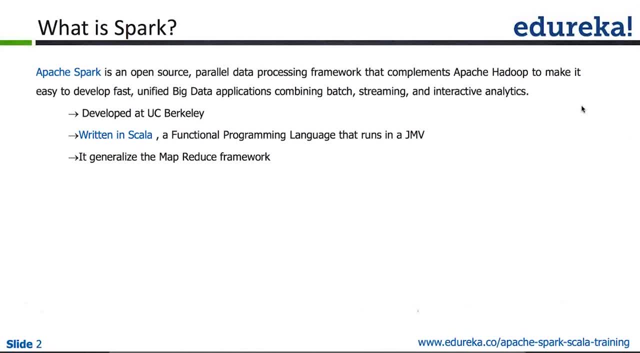 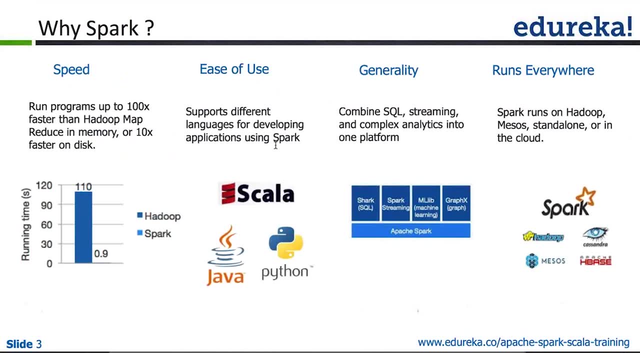 I will now go into the dissection of it and we'll go into the details of, you know, Spark ecosystem. When I say framework, right, what are the components of framework and things like that? those are the things which I'm going to cover now. 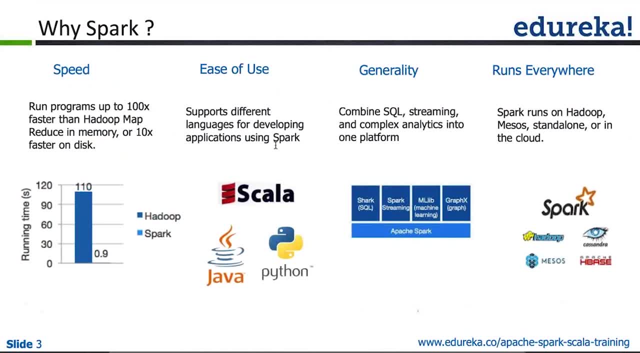 Well, this was the place wherein I just told you, right that, what is Spark Being a framework? The next question: well, why are you trying to sell me Spark? Okay, why are you trying to, you know, give me the idea that I should be using Spark? 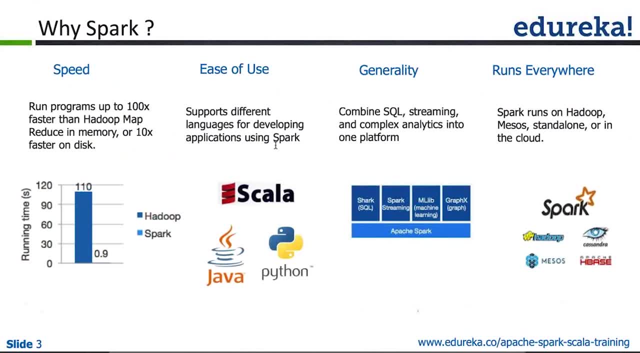 I have already started my big data journey in Hadoop and I'm quite happy and other stuff, right? So these are some of the reasons, guys. Again, these are the reasons which might be applicable to you or might not be applicable to you, right? So the reasons to go to a specific technology or not. 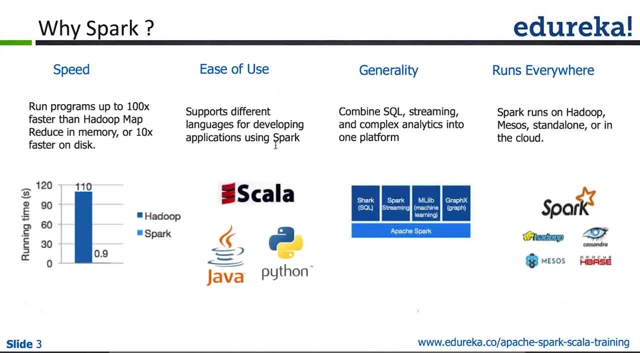 will be completely driven by the context, The kind of application development or the framework development, whatever you are doing in your respective areas. So if you have following concerns, as I'm going to, you know, consider them one by one- you should consider Spark as a solution for your- you know, whatever project. 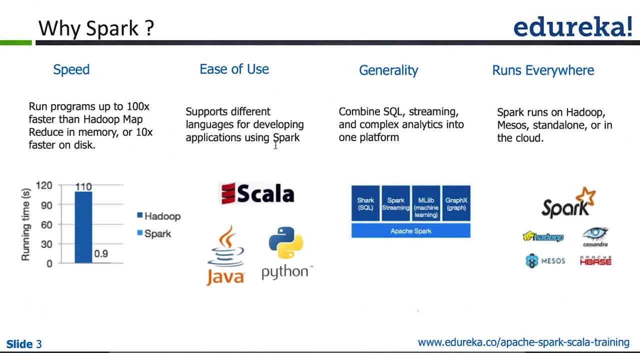 you are doing The first thing, speed. Well, this speed thing comes with a rider. okay, It comes with a rider that you want to. whatever processing you want to do, you are doing on a huge set of data, but you need to do it at a very high speed at. however, 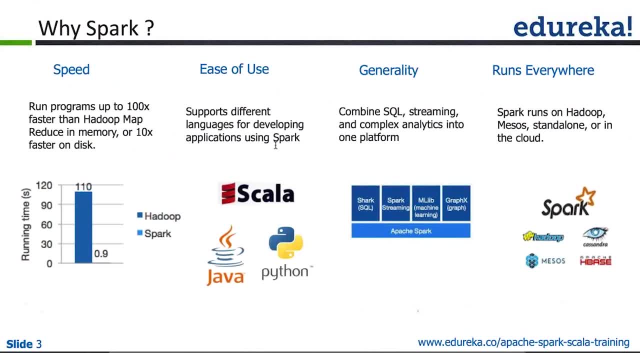 at one point of time when you are processing this huge amount of data, the kind of volume which you are processing at one time is not very huge. okay, So the difference between, let's say, a Hadoop processing or a Spark or, for that matter, any Hadoop process, 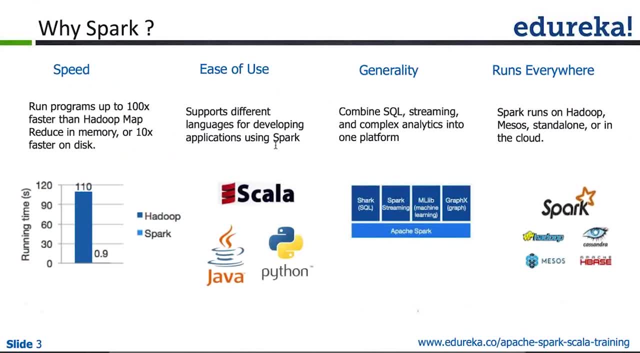 for that matter, any other near real time system processing is Hadoop- will go through, let's say, five terabytes of data in one pass. okay, If you have that kind of requirement, that you have an entire five terabyte of data and you have to go through. 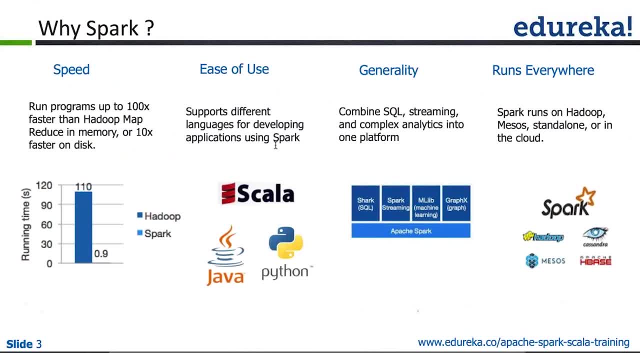 that entire five terabyte of data in one pass. you better need to do the Hadoop processing or the conventional MapReduce processing. There might be another case, guys, in which you- I don't know Again- have five terabyte of data but you don't have. 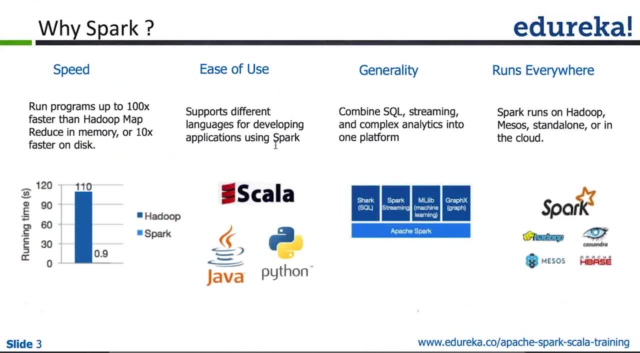 to go through all of that- five terabyte of data in one go. Example, the best example, is: let's say you have an event, right like you had IPL, you had World Cup, cricket, and you know there are various other events which keep happening. 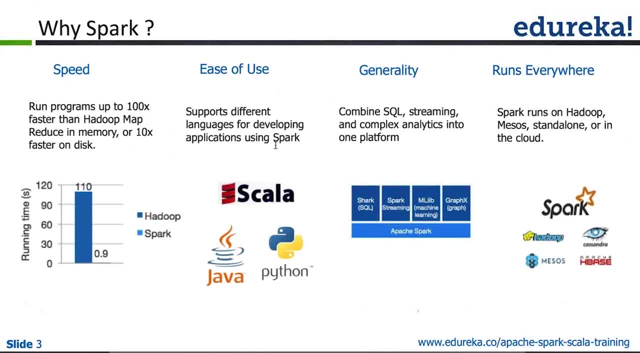 Then there are tweets which are coming in, which are pouring in right Now. if you combine the length of all of the size of the data which comes in the form of tweets, right, Let's say for an event like Indian Premier League- it will be several terabytes. but is all several terabytes? 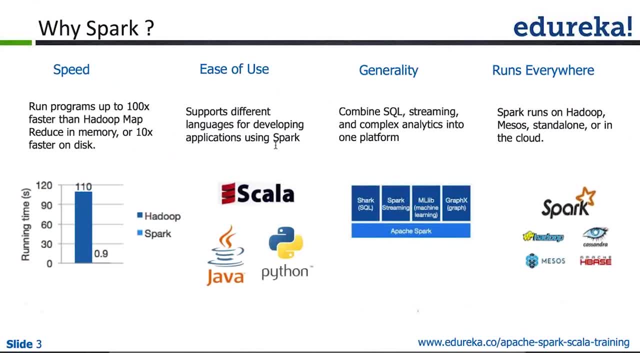 coming at the same time? Is all terabytes coming at the same time? No, it is coming over the period of days. Are you guys getting the point? So let's say you have the analysis wherein you want to find out today, as of today, or as of, let's say, last 20 minutes. 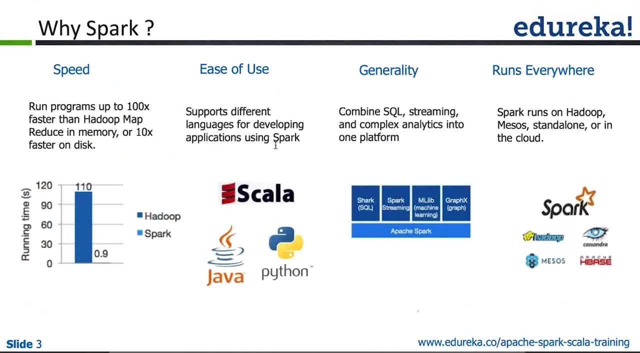 which team was the most talked about team right. So some team is really performing well today. That would be probably the most talked about team. Then the other team starts performing, let's say, by the match which happens at the end of the day, the other team takes over, right? 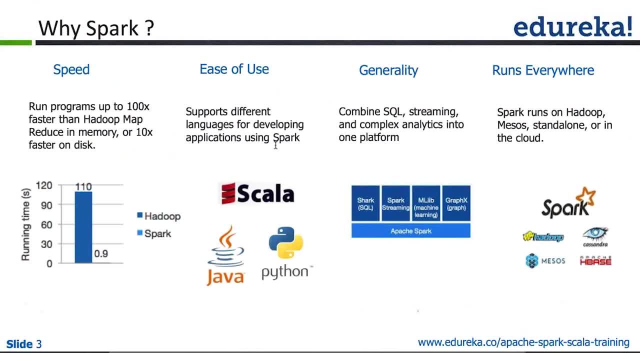 You want to do these kind of analysis Continuously. you just want to show those kind of real time, you know updates to them. At that point of time you don't really need to process all of the five terabyte of data, or you know? 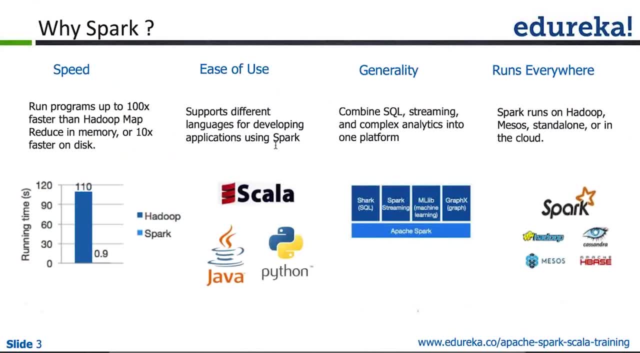 all of the data, whatever has come in the history. You're processing a chunk of it continuously. That is where you know Spark will come into picture. That is the kind of analysis which you would definitely like to do very quickly, pass through your data. 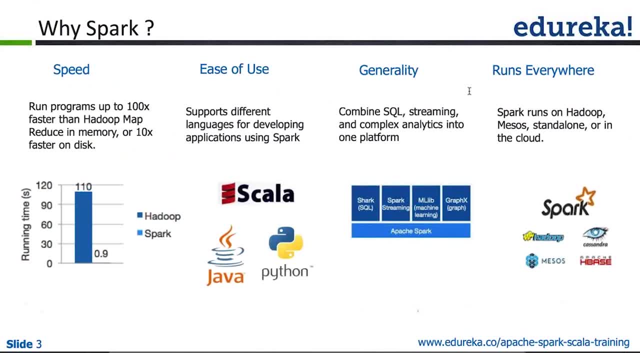 and then show it to your customers. Typically, we call them as the windowed operations. Is that clear guys? So why Spark? even before coming to that part, I just wanted to go to the detail Of the difference of use cases. Guys, could you confirm whether was that helpful? 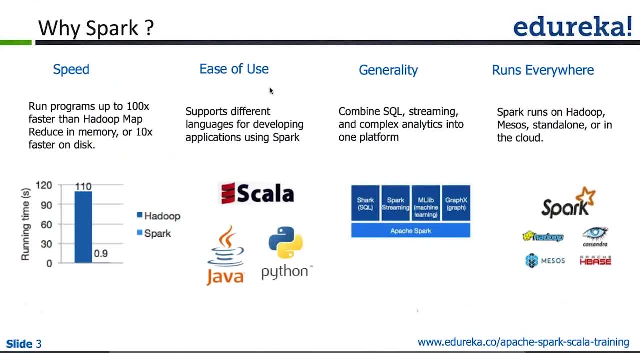 Was this example helpful to understand the basic difference of the use cases? Right, thanks, thanks a lot for confirming. Sure, now the next thing. right, So the speed part. I hope it is quite clear that if I'm going to give you The idea about which is the most talked about team, 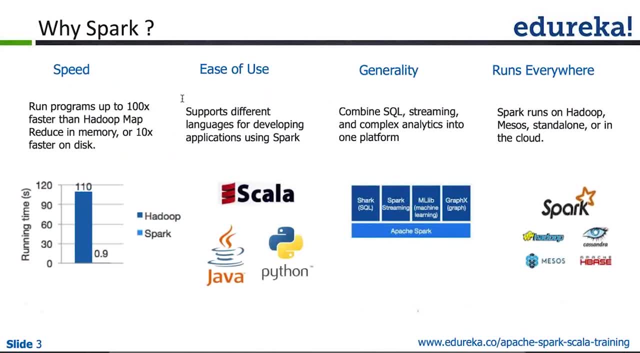 and other stuff, Then I would better need to do it in a at a higher speed. Right? I cannot give you the. you know the details. which is the most talked about is team when the matches are over. Of course, it doesn't really So. speed is one aspect and, as a comparison, 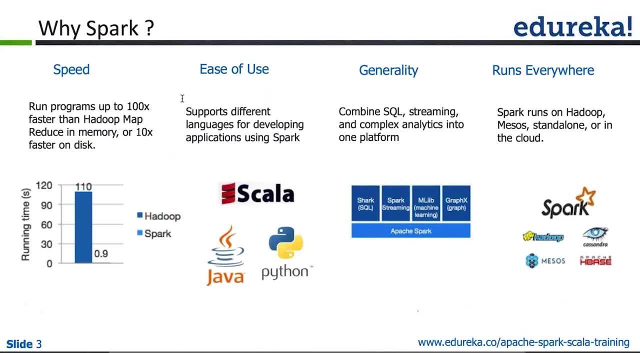 I'm not saying it is the benchmark, but as a comparison, in some cases the performance of the same program In Spark is almost hundred times faster as compared to the operations happening in Hadoop. that is first thing. Second, Spark can never become a very popular system. 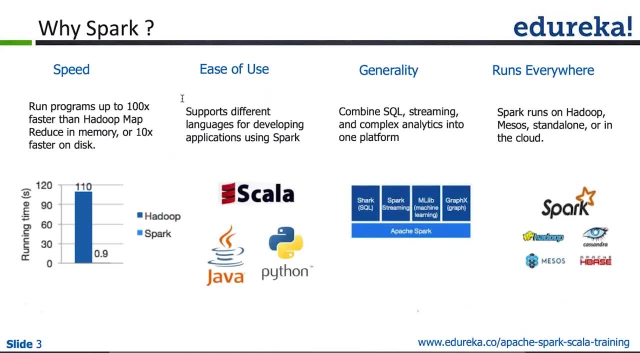 until and unless it opens it up for the people coming from different background. When I say coming from different background, it is written in Scala. if I ask in this forum All the people who are listening to this webinar, right I'm sure if I say how many of you have worked on Scala. 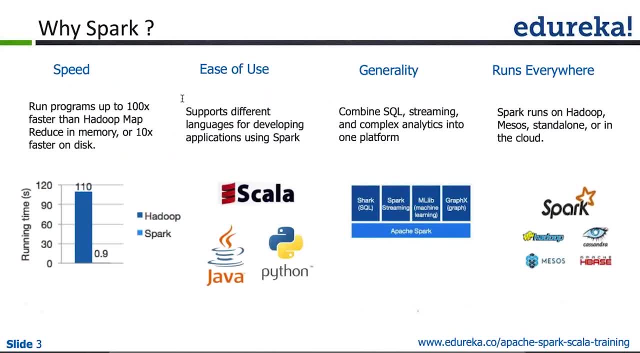 Not many would have worked on Scala. You must you. some of you might even be hearing about this language for the first time, And whereas. so if I say that my framework is just going to support Scala, Not many people are going to, you know, being it being. 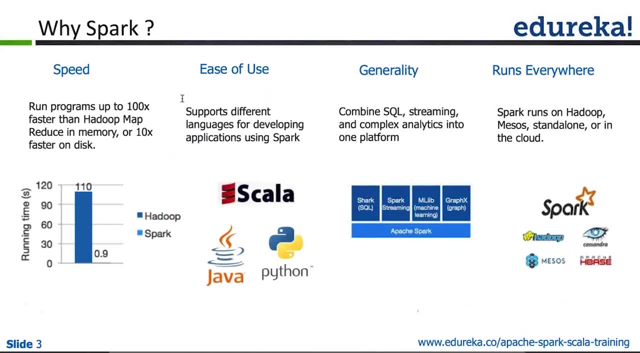 or open source community. Not many people are going to contribute, So Spark Spark opens it up for multiple languages. Sometimes we call it as polyglot or nature. right, You can write your programs of Scala- sorry, your programs for Spark- in Scala. 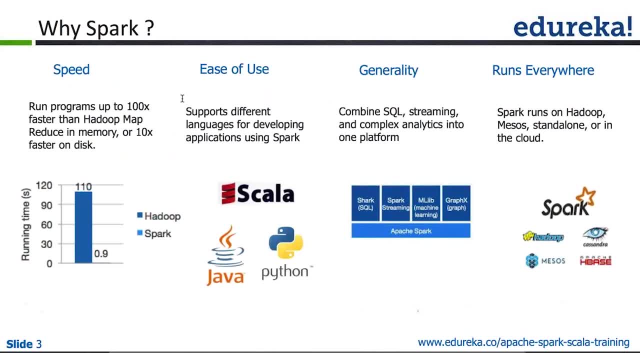 You can write them in Python and you can write them even in Java. Well, with Java, I will say: write your program in Java, but please try to use Java 8, don't use Java 7 or any version below the reason being: Java 8 introduces new features, like streams, like lambdas, 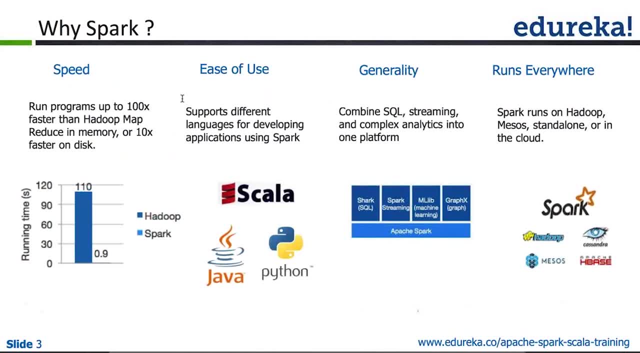 and you know optionals and other stuff which is best suited for the kind of programming which you need to do in big data world as compared to the old-style Java programming. So that's the only rider. Please just keep it in mind. However, you know Spark is in under active development. 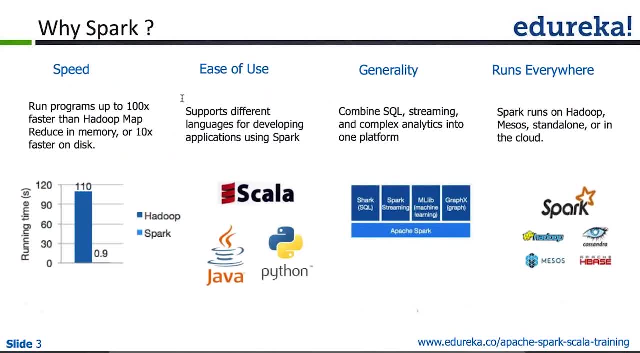 for the support for the language, So that's the only rider. please just keep it in mind. However, you know Spark is in under active development for the support for the language, So that's the only rider. please just keep it in mind. So Hadoop is a framework wherein you know. 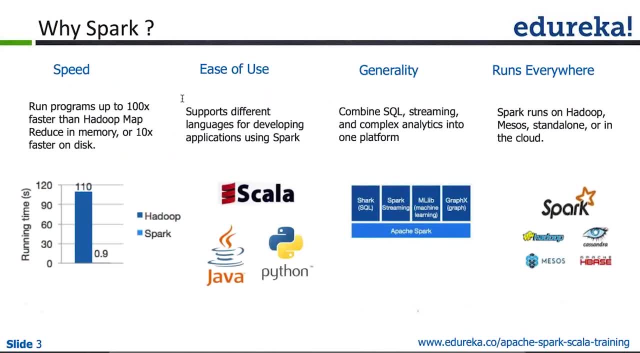 you can write a plain MapReduce program. or if you are coming from a you know SQL background, you can use hive. if you are coming from the data flow background, you can use pig and things like that, right? so people coming from different backgrounds can still leverage the power of 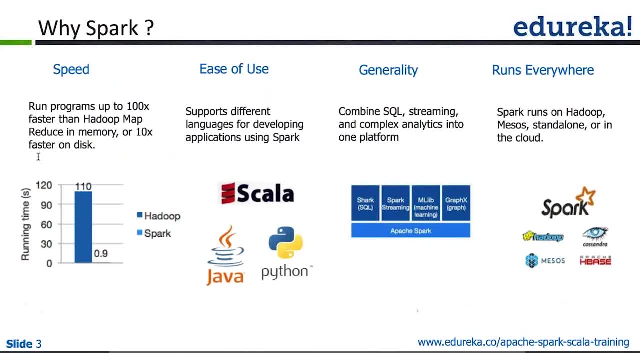 Hadoop and spark has gone exactly in that direction. so if you look at this, this particular part where my cursor is right now- general generality, and under that there is a small figure right, I will be explaining it in bit more detail in a dedicated slide, so at the bottom of it you can see Apache. 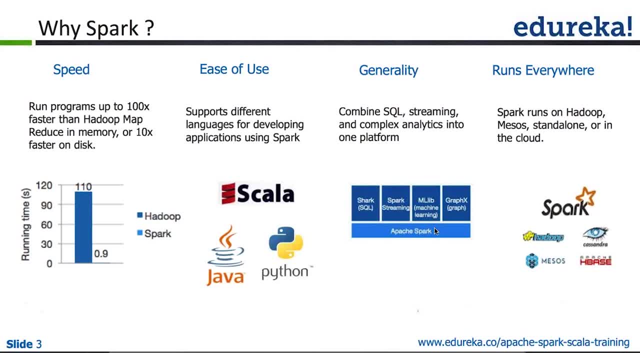 spark. this is the core engine. okay, it's like you want to write raw Scala program which just deals with the core, you know, which just spawns a pure spark process altogether. you can do that. there might be some people who are not really good in Scala or you know that basically they are not. 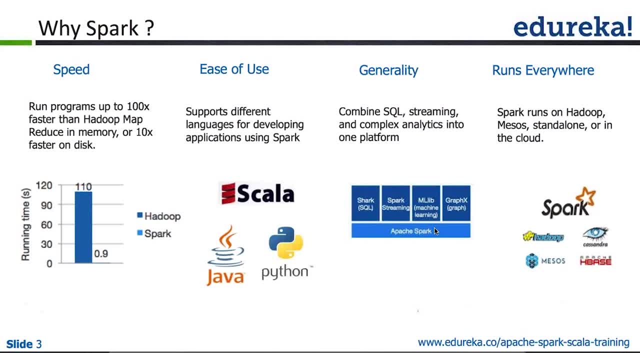 coming from the program background, they might be coming from the queries and, you know, the data analyst or the data guys. basically right, so those kind of people typically would like to use shark, or now we call it as spark sequel. okay, so shark or spark sequel they would like to use. so in that case, for them all, they 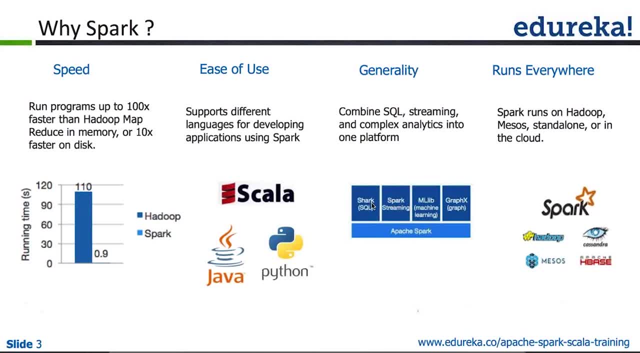 would be doing is they would be writing SQL queries and they will be converted to the spark programs and you know they just so they just get the benefit of the program and they will be able to send it to the the same speed and all that stuff by spark. there might be some people who would like, who might be. 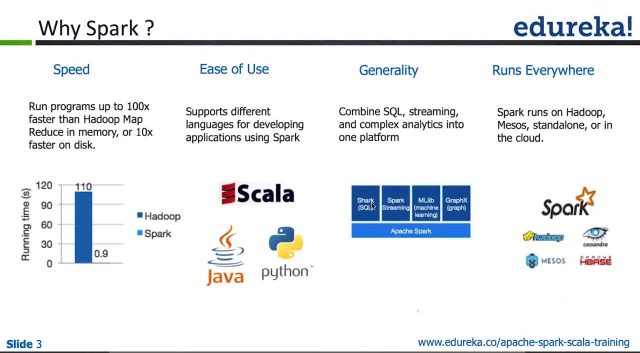 having the requirement of streaming operations. well, the best example of a streaming operations is: you are getting the tweets right for an event, you, so it's a continuous stream of tweets. altogether. you want to do those kind of operations. you know spark streaming supports that. well, you want to do. 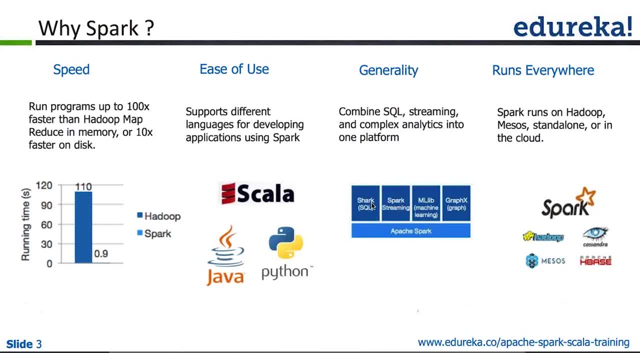 some sort of a graph processing or machine learning kind of algorithms. you must have heard about Mahout, Apache Mahout and all right. in fact, the next version of Mahout will not be on Hadoop, it will be supporting spark base engine. okay, so anyway, the idea is. 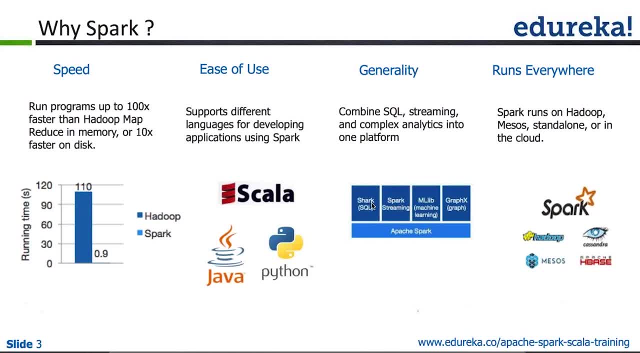 you want to do some sort of machine learning or you know some sort of graph processing and all. so those kind of libraries are also being built. okay, some of them are out. when I say out means they are released for public. some of them are still in the, you know beta releases and other stuff, so that that is. 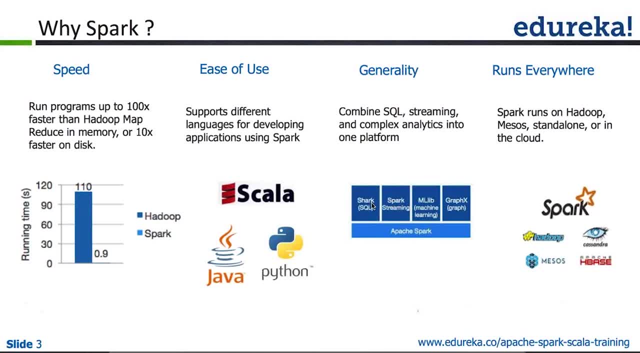 one. the other advantage of spark is: well, when you say that I'm going to use spark, you don't really need to create a silo in your organization. you don't really need to say: well, this is the spark system and you know, give me a full-fledged cluster. and you know, give me a, you know, entire, entire investment. 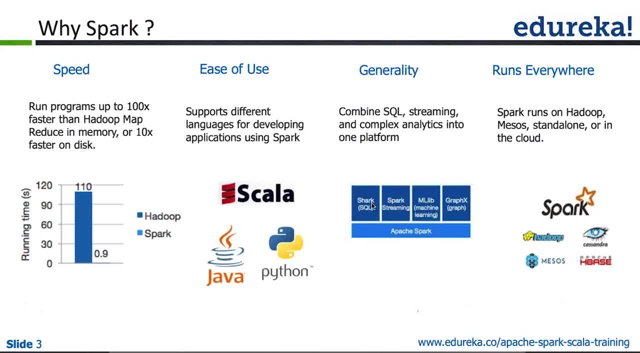 directly from zero. you don't really need to do that because if you have spark, you can deploy that in the existing Hadoop cluster itself. so a spark supports the integration of Hadoop and Spark and you can deploy that in the existing Hadoop solution. with Hadoop, spark can run standalone, spark can even be integrated. 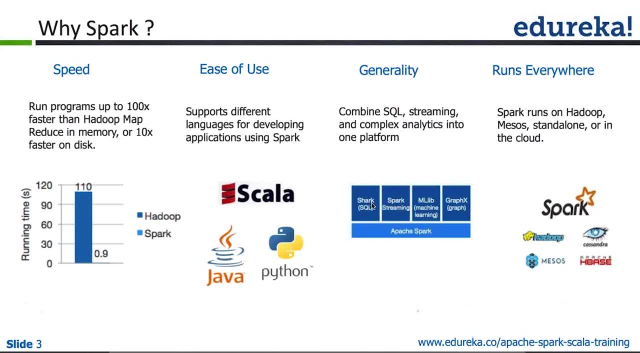 to another cluster manager called mesos. okay, so I will come to coming slides. but yes, it can be integrated. at the same time it supports the storage is like you know Cassandra, you it can fetch the data from Cassandra, store it back to Cassandra, and the same goes true with HBase also, and I mean those things should not come. 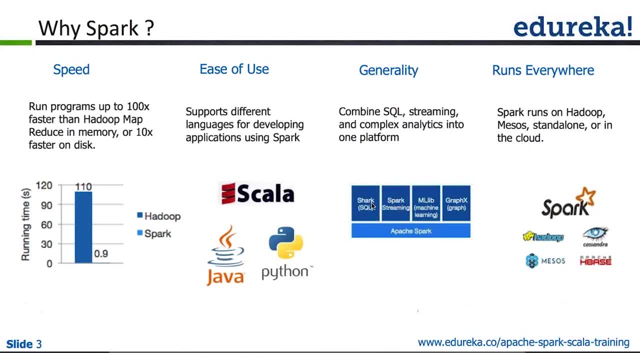 as new because it is integrating with Hadoop right, in fact, that that kind of integration is the most popular in the industry right now. wherever you talk about, you know applying lambda architectures and things like that right. so, guys, I hope it gives you enough idea about the reasons, the main concerns: 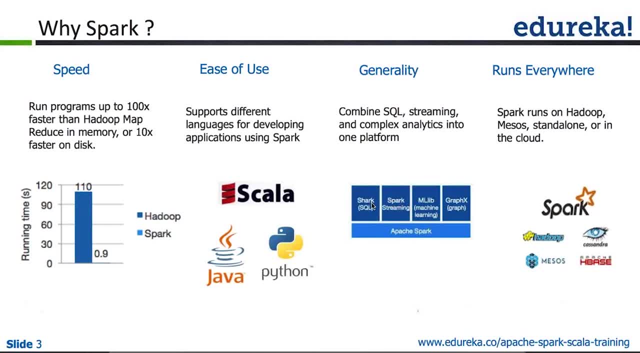 if you have any of those concerns, probably you should start considering spark as a solution, part of your, you know, as a part of your entire solution. I would say: right, so far. so, good guys, I hope you are there with me now. I'm just going to go back, okay. so why spark? basically, it just continues the very same. 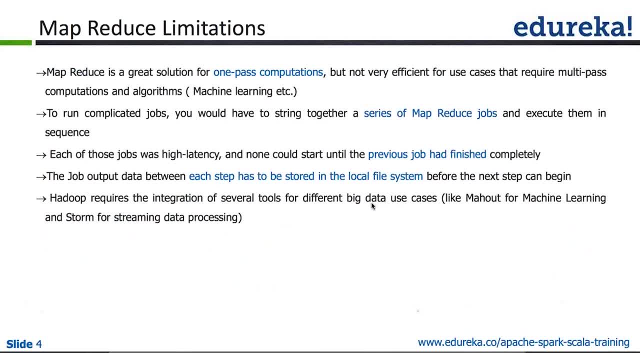 discussion and the assumption here is most of the people must be aware of map reduce, right. so map reduce is a very important paradigm altogether and it is a it's. it's a great solution for one solution and it's a great solution for one pass computation. as I told you right, Hadoop is best. if you have to, let's say: 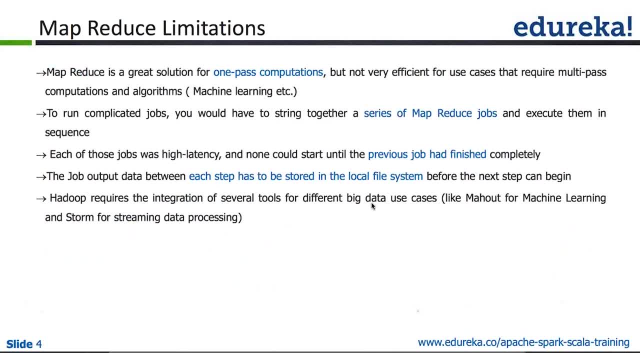 go through five terabyte of data in one pass and do some sort of processing. you cannot beat MapReduce at all. but, guys, this algorithm is something which is not really very good for multi pass computations or iterative kind of algorithms like machine learning, like clustering, right, the same kind of. 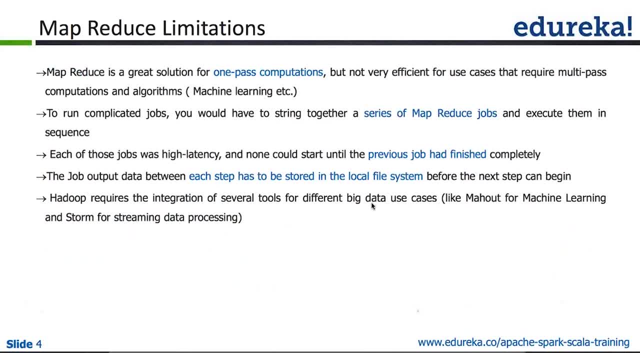 program you have to run ten times. are you planning to do it in Hadoop? yes, you do it in Hadoop. you do it. why I'm out? yes, you do it, but it's not the most optimized way. that is first thing. well, as I said that, you know one pass nature of typical MapReduce programs and all 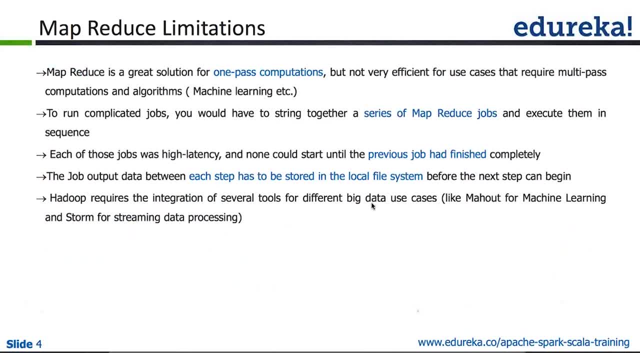 with the same logic. if you have a very complicated kind of a business logic, right, you will have to do the same kind of business logic, right, you will have to do the chaining of the jobs and all, and this chaining of the jobs is something which is a real pain in MapReduce applications. if you have to do a 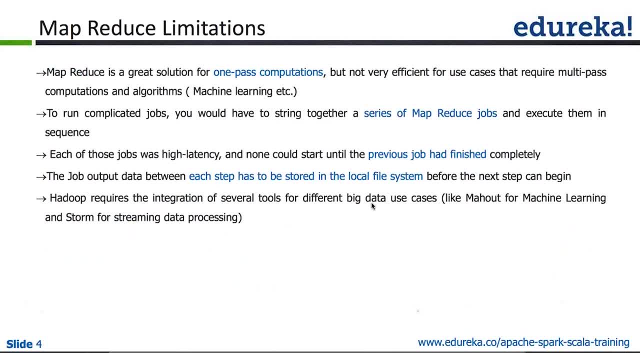 chaining of one to two to three programs, still fine, but if you find yourself doing the chaining, let's say, ten programs, something is wrong. okay, so those are some of the things which are like the real pains, and the worst part is, if you do the chaining, your other. 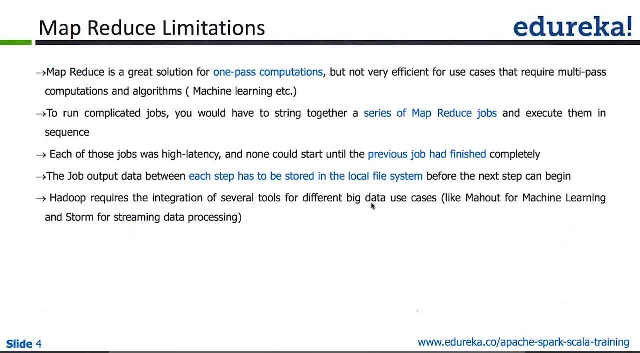 program cannot start until unless your previous MapReduce program has completed and persisted the data. okay, until unless the data has been persisted, you cannot really start the next system altogether. okay, so that is something you know a bit clunky part of the MapReduce thing. these are some of the you know basic problems. 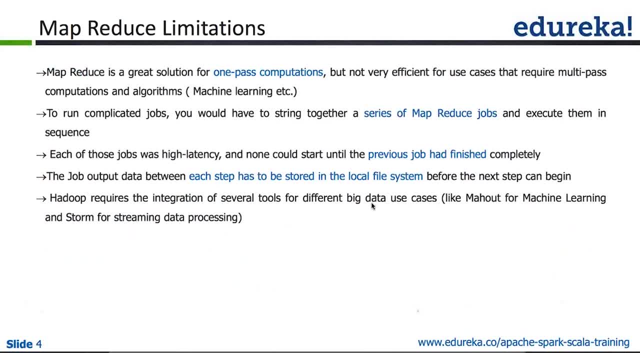 wherein people identified that, okay, MapReduce is actually having the limitations on these areas. okay, and in fact, these were the driving reasons also for the evolution of, you know, other systems like so, by the way, spark is not the only system to do the real time processing, there are other. 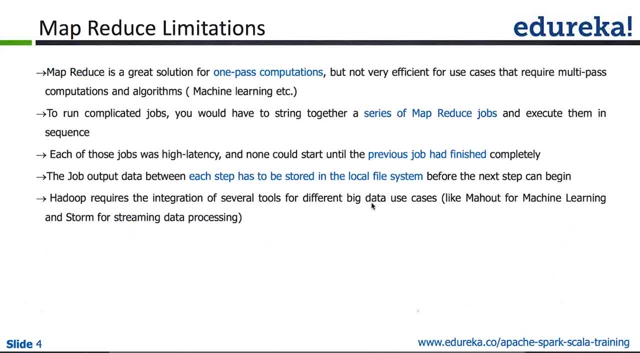 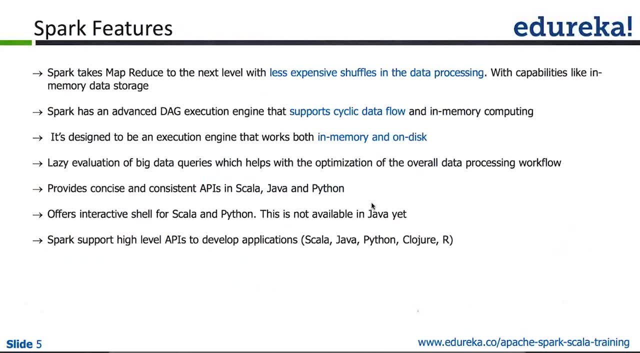 systems like a storm. there are other systems, like asper and others, but spark holds the advantage because it is a framework, not a specialized system. okay, so these are some of the limitations of MapReduce, now how exactly spark handles these kind of scenarios. so some of that you must have heard already. I'm just 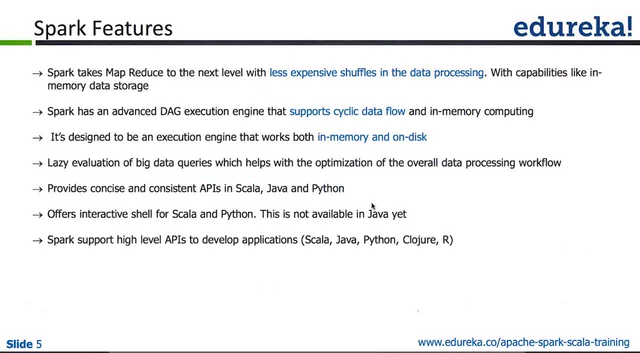 going to explain them in bit more detail. so, guys, the first thing, first spark, generalizes the concept of MapReduce, okay, and it basically leverages the distributed memory altogether in memory, all together in memory, all together in memory. data storage, I would say so, the backbone of your entire, you know. 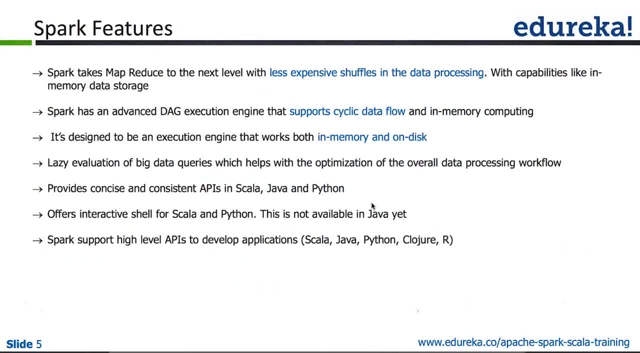 operations is called RDD, we are called resilient distributed data sets. you will hear more and more about it when you know we'll be talking about the actual course and you know how exactly Spark works and all. of course. one is not the enough time to discuss about that, but yes, just to give you a hint. anything and 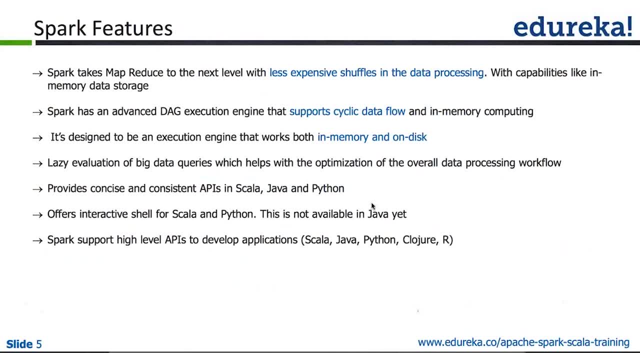 everything you're doing years world. you are working actually on the RDDs, resilient distributed data sets. they basically, as I said, distributed data set. so it's like in-memory distributed data set and you do the processing in in-memory part altogether. so of course, in-memory processing is going to be many times faster, as 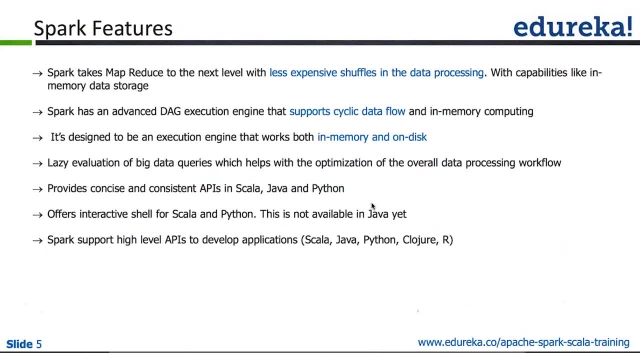 compared to on-demand paging of the data from this right. that is first thing. the other part: is it so all of the computation? don't think that if I have expressed a computation and when I execute it, all of the data would be there in memory. no spark holds the directed acyclic graph of the execution. 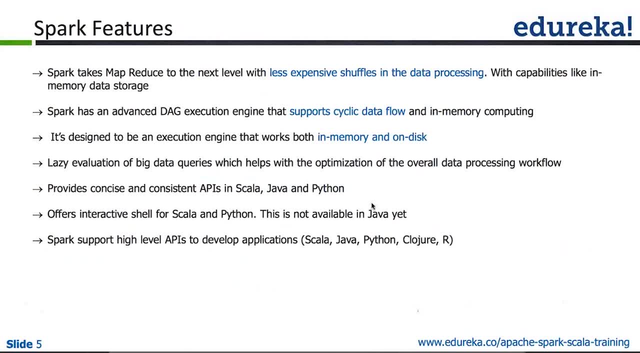 not the actual result of the computation in memory. okay, until unless you persist the data. okay, so you have to explicitly persist the data if you really want to do that. you have to explicitly persist the data if you really want to do that. but it just holds the directed acyclic graph of those executions. use some of: 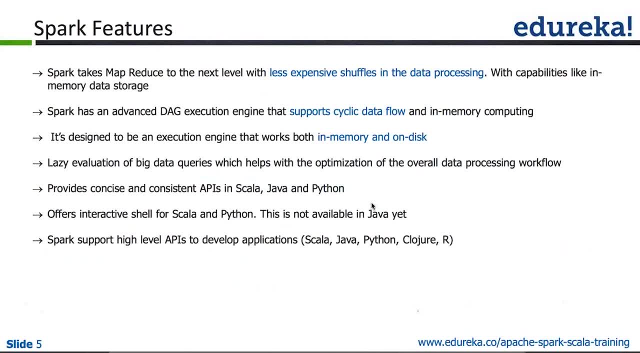 you who are aware of PID, you might be finding some resemblance here right now. this is something which is very useful because, guys you are talking about in memory storage and if something goes wrong, spark uses the very same, you know, acyclic graph to reconstruct it, to reconstruct the data. 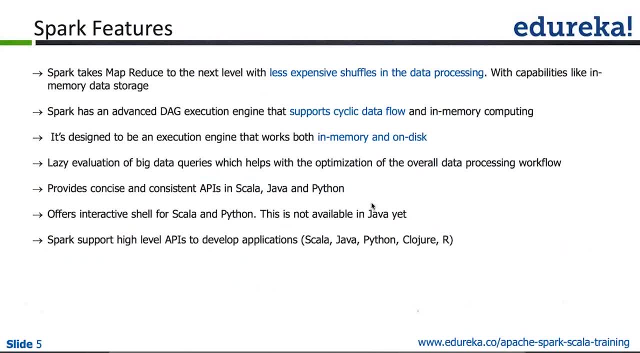 just in case you wanted to persist the data and it is lost, spark still can use the very same acyclic graph to do the computations again. so anyway, more details when you will come in the- I mean when, if you choose the course, and at that point of time we, when we talk about the failover capabilities and other 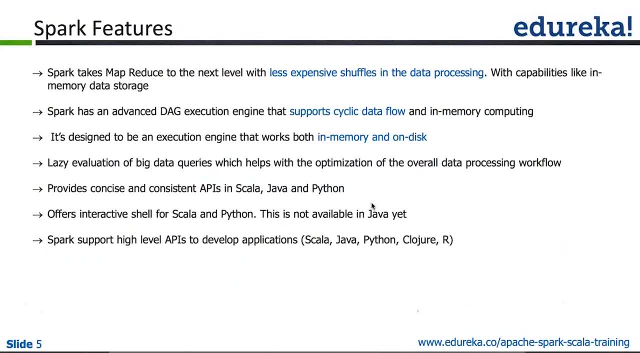 stuff. we'll be dealing with this, these things, in bit more details in the course. the next thing: I just told you that you keep the directed acyclic graph in memory and at the same time you can store the data either in memory or on the disk, or both. so when I say both you 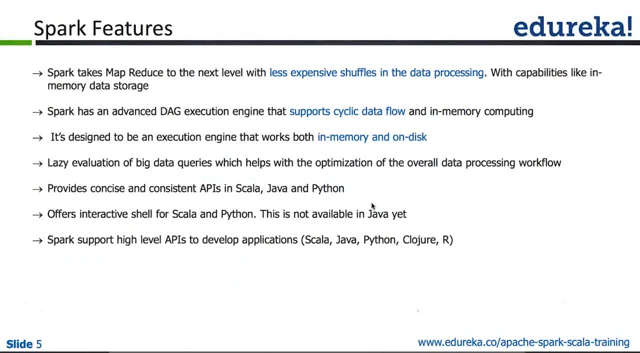 can say: 70% of my data is going to be in memory, 30% of the data is going to be in disk, or vice versa. so spark gives you all of that flexibility. all together, right? it's the lazy evaluation of big data queries. the same thing, guys, that you. 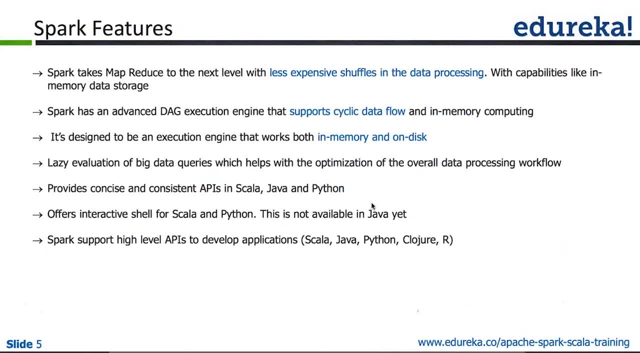 spark is not gonna execute your program as it is. it will. so you have created an expression until unless you are going to use that expression, spark will not execute that computation. so those kind of optimizations come by default. you don't really have to do all of that stuff. and last two points are last, but 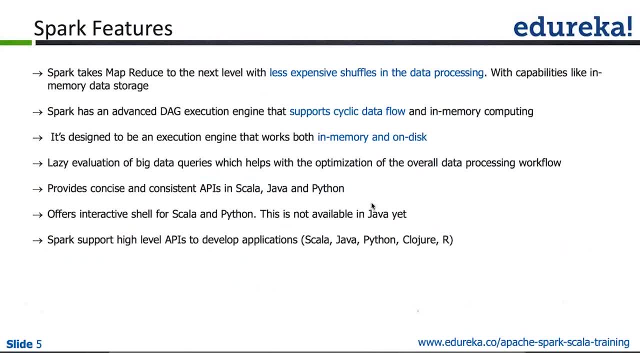 not the least. okay, so the best advantage. I mean, I'm assuming some of you are already working in this big data domain and are aware of systems like pig and hive and not other stuff. what is the best thing which you find about pig and hive? the best thing about pig and hive is one: they are convenient, but even 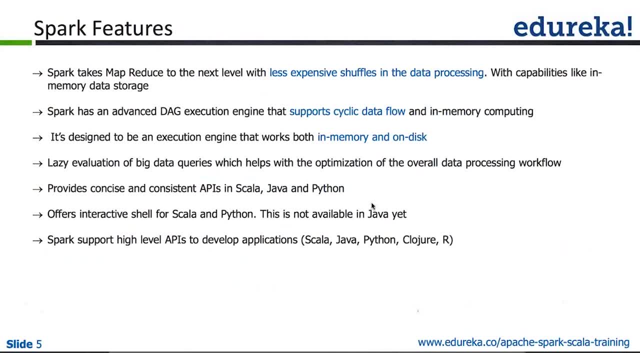 even more than that. they provide you the interactive shells. okay. so you being the engineer, you don't really need them, but typically, if you are, if you have ever worked in the analytics area, if you have ever worked in the analytics area, you okay. then you must have found some of the data scientists, and they are the guys. 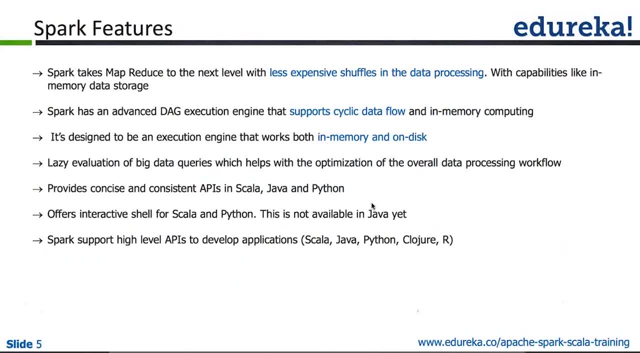 who typically like to do very ad hoc work. right, they have some kind of hypothesis. they just want to do very quick modeling of their hypothesis, the quick test of their hypothesis and whether it is producing the right result or not. they don't have the patience of writing the program, they will just want. 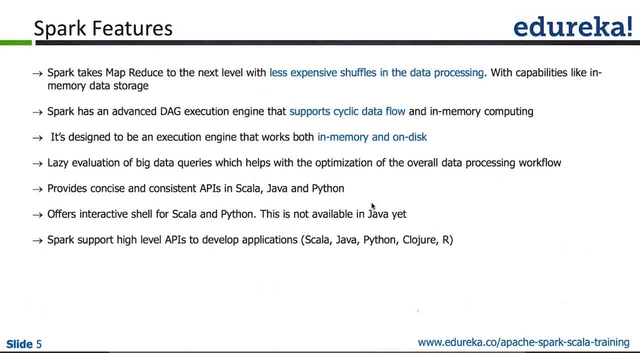 some sort of interactive thing, and spark does exactly that. so if if you are working in Python, if you are working in Scala, you get the interactive shell, Java, of course, cannot give you the interactive shell right. so interactive shell is available in Scala and Python and the best thing is if you have done. 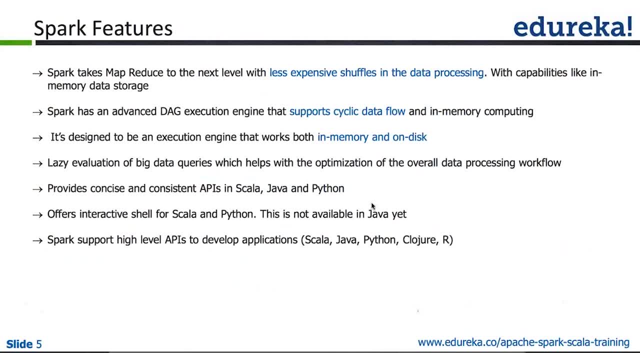 an operation there. well, you can guarantee that it is going to work in production also. so that is first thing. the next part, I think it is repeated. so the API is support the application development in multiple languages and Scala, Java, Python. as of now closure and are sometime in future you should see. 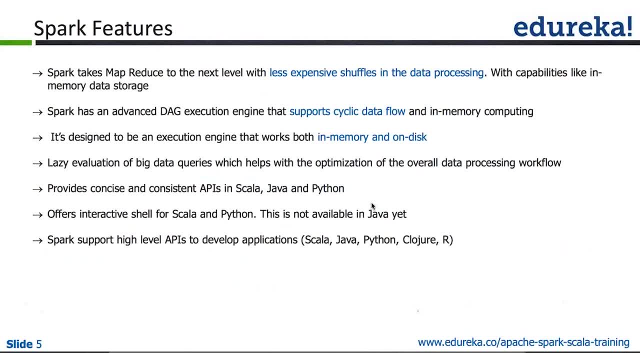 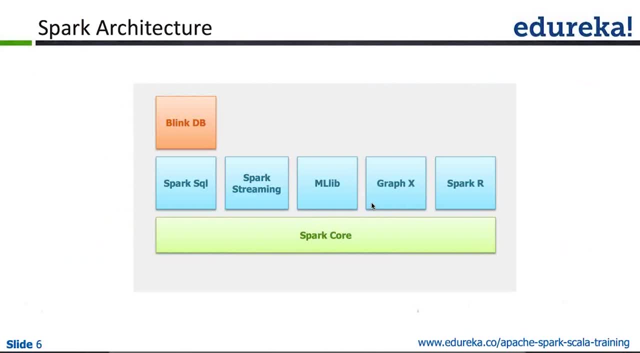 the support from these two languages also. okay. so I hope it just gives you a better idea about the features of you know spark. well, guys, I was mentioning about the ecosystem spark being a framework. this is the time when I I can devote some more you know minutes to it. so, as you see this you know picture by 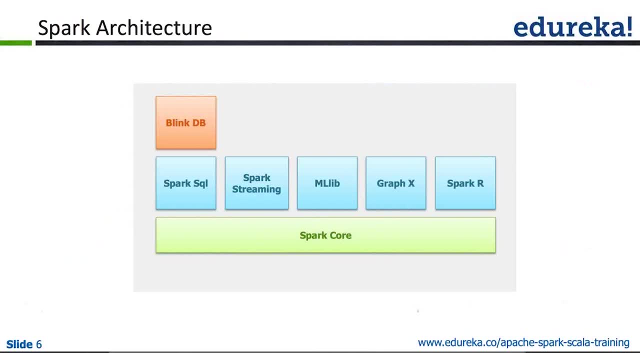 the way before I proceed, guys, is it going good? are you there with me? speed and all is this okay or bit fast or just want to quickly understand from you all: good, thank you for confirming those guys who are confirming. sure, thanks a lot, guys. this really helps me. 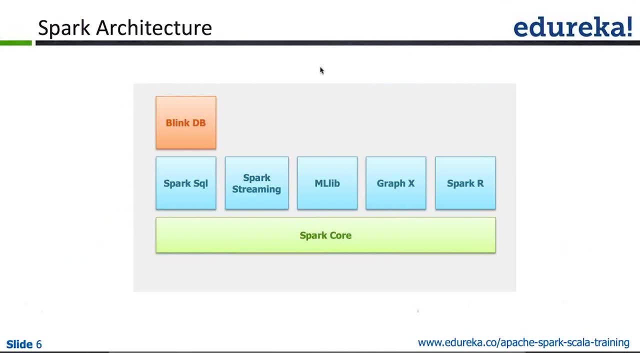 to understand whether you know it is relevant to you or not also. thank you, guys. so I'm just continuing on the very same lines here. now the architecture of it. so, as you can see, there is this spark core, which is the at the bottom right. it's just like those people who are 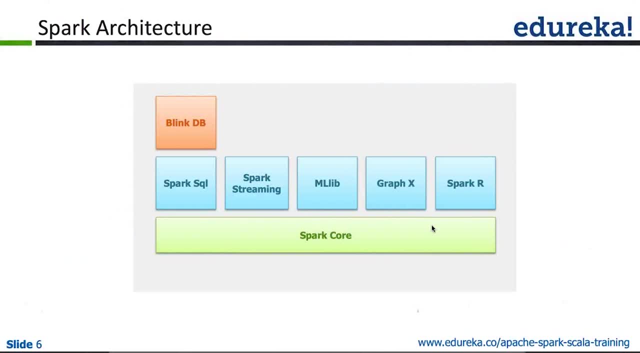 aware from Hadoop ecosystem. they must have seen HDFS and MapReduce being the core of components of Hadoop right. similarly, spark core is the core computation engine you can. so if you really want to deal with it, you can just write your programs either in Java. 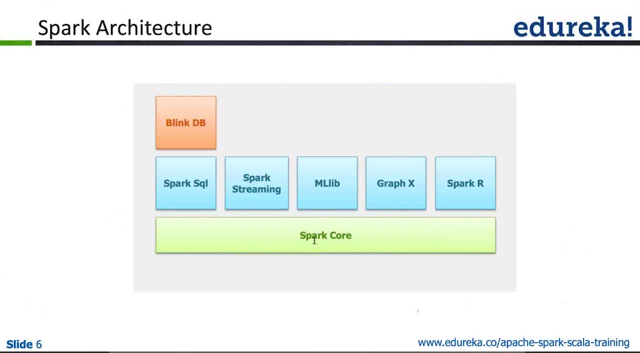 or Scala, and when you fire your programs, you are actually dealing with this layer. you are actually dealing with this layer. but if you are coming from SQL background or you want to do some sort of streaming operations, as I told you, you know. that's why I am calling it as this ecosystem, because if you are coming from the SQL background, 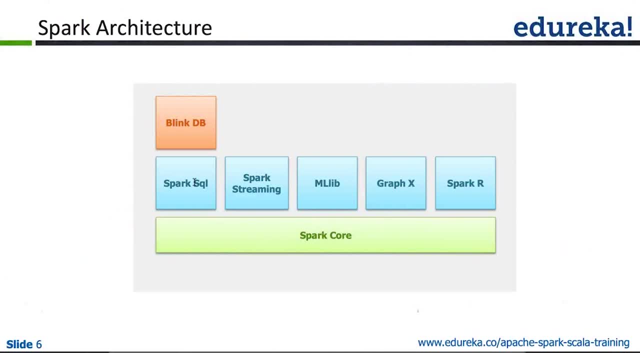 you would like to use spark SQL. it's like equivalent of hive, right, but the difference being it is hundred times faster, in fact, in the course. so, by the way, let me just tell you the thing till some months back, I think. when I say one months back, just two months. 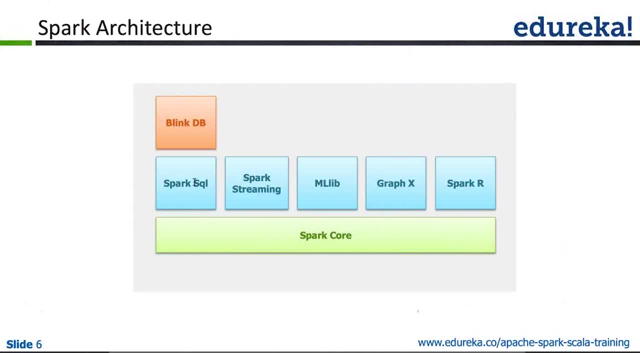 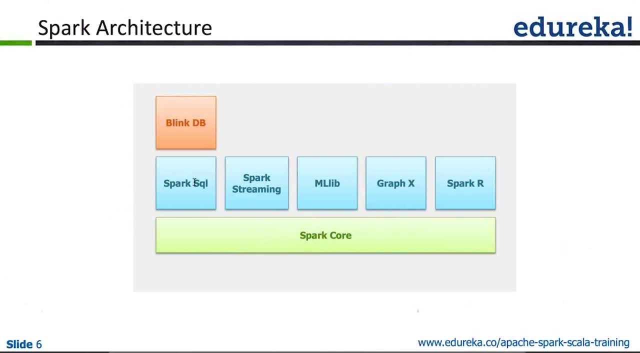 it's the duplication of a word, right? you know the good thing: spark SQL is now integrated with hive. the best advantage: your same hive query, same hive query, copy paste and run it in spark. you would be able to run it hundred times faster. so what did you do? just a copy paste and nothing else. you don't have to even define the table. 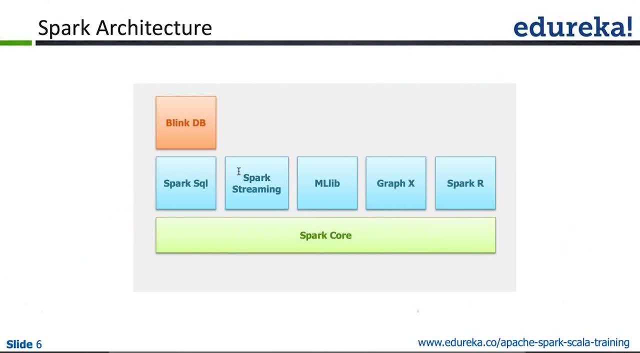 nothing at all. so isn't it one of the great things: all together, just connect and you are able to plug and play all together. that is something which, so, in this version of course, which will be, I think, launched from tomorrow, we'll be covering the integration of a spark. 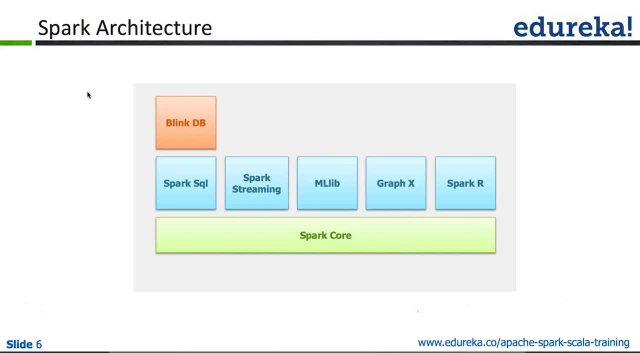 SQL and hive. that's a new feature which we have added from this batch onwards, so that is something which will be covering. then spark streaming- it's a I would. I'm not sure how many of you have heard about Apache storm, so apache is basically, I would say, spark. 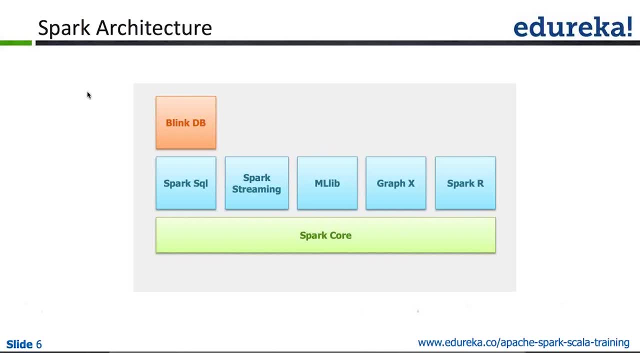 streaming resembles to storm operations a lot. I would stop at this point of time. more about that when we'll actually be covering you know when we'll actually be covering our course. then ML live and graphics- I just covered them right there, like machine learning libraries as well as your graph processing. 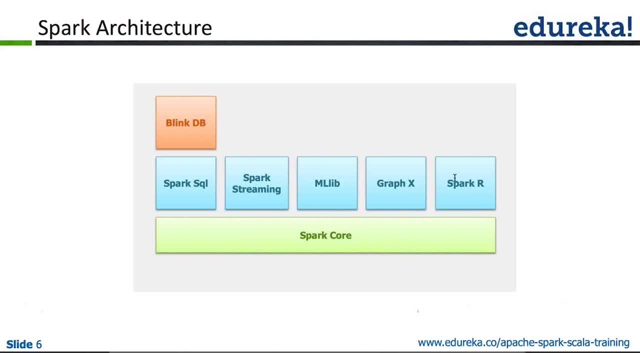 if you want to do and then you have a spark are. well, this, this color is wrong guys. it should be. it should not be blue. it is the orange color- orange color for graphics as well- as a spark are also, so they are the libraries. spark are are is a statistical programming. 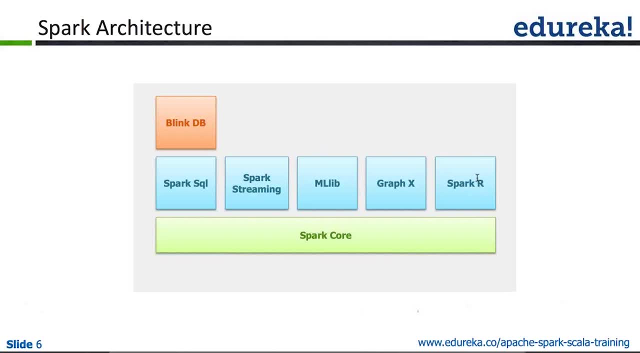 language and spark needs to provide the support to Spark. it is not yet there, but, yes, it is a work in progress. okay, so once it is ready, all those people who do the statistical analysis and are they can integrate. there are programs to spark and again take the advantage of the very same speed. right, so that that is the 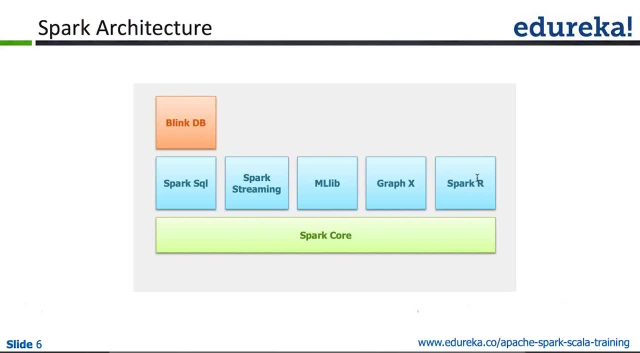 direction which will come. then there is an interesting database called blink DB- blink database altogether. well, as the name says, blink it's a, so it supports something called approximate SQL. I will not go into the details of it as of now, just that sometimes you are not. 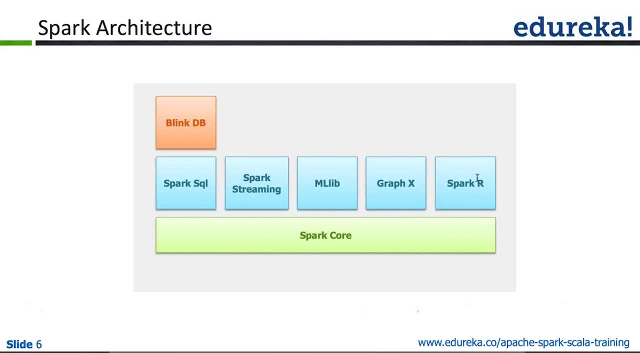 really interested in exact numbers. for example, I will take my favorite example of IPL. right, there are three hundred thousand two hundred eighty seven tweets, right? are you really interested in this? or are you interested if somebody tells you you know what? till now, I have got three hundred thousand plus tweets. 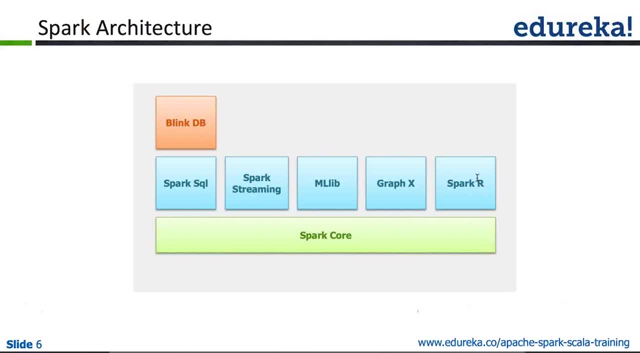 Right, So that's the idea. first is the exact number, second is approximation. only thing is the first one: if you execute it will be slower. the second one is just going to do some sort of sampling to you and it will be much faster. right, so blink. DB is sometimes called as approximate. 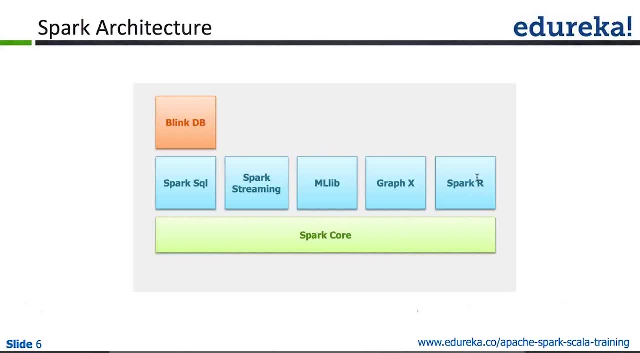 database and it is basically for the approximation queries and all again, this is something which is work in progress, it is not yet released, But yes, as you can see now that if you combine all of that, you have got something for everybody. you know a database guy, a guy who is a core programmer, a guy who is a machine learning. 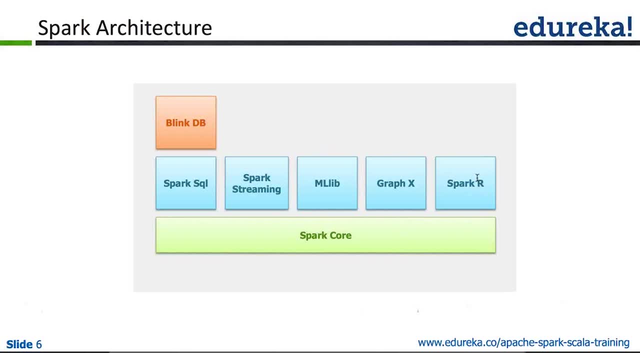 enthusiast, or the social media. you know those, those graph processing guys, the guys who are coming from the statisticians, right, the statisticians all together, so you can see that many people from different angles can use the very same architecture To do whatever they want to perform. are you guys now clear? what do you mean? what do I? 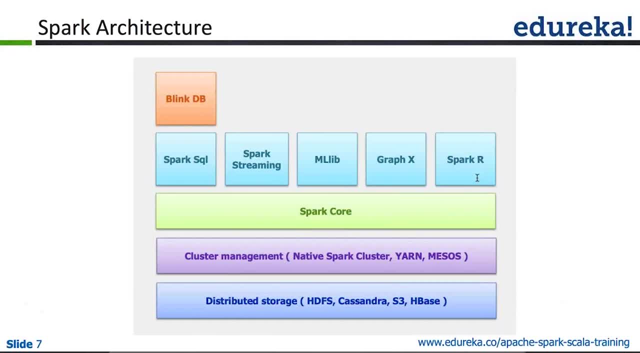 mean by spark being a framework, right? I hope it should be quite clear to all of you. I tried, like my level best one explain that. why am I calling it as a framework altogether right now? the next thing is: well, these two things are just the add on. I would not spend much. 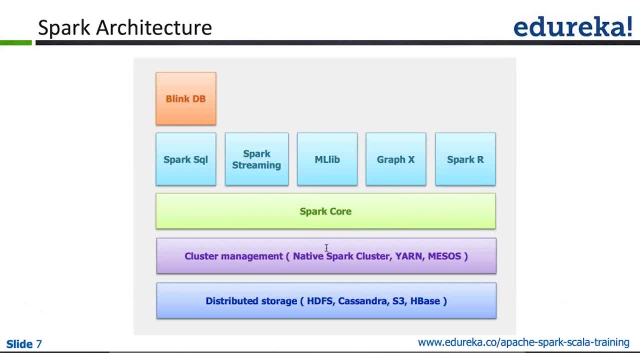 time at this point of time, As you know that this was the ecosystem, but it can be integrated to any cluster management. as I told you, it could be hadoop, it could be its own cluster or mesos and the data could be stored where. it could be your native file system, it could be HDFS, you might be fetching. 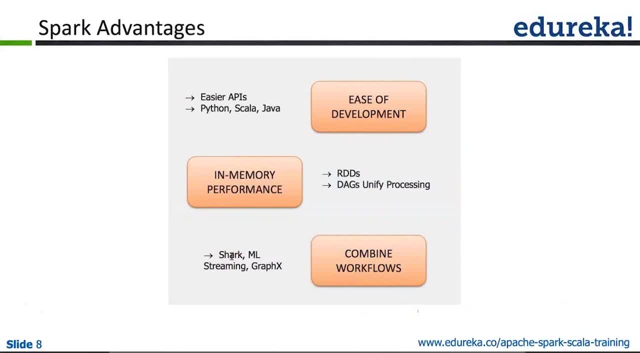 the data from HBase or Cassandra or any other file system. so, yes, spark supports that kind of integration And that's what makes it very, very powerful all together. now I will spend few quick minutes, okay, to tell you the advantages of a spark. to tell you that I mean advantages of a spark. 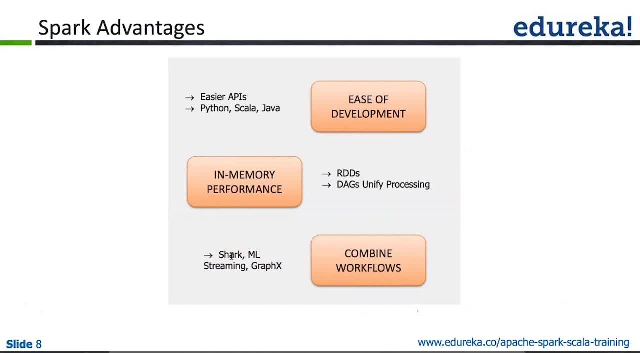 should be quite clear by now. but then the advantages of hadoop and what you really get when you integrate both of them. okay, So let's start with it, okay, Well, So these advantages should not be new to you. ease of development because of the easier. 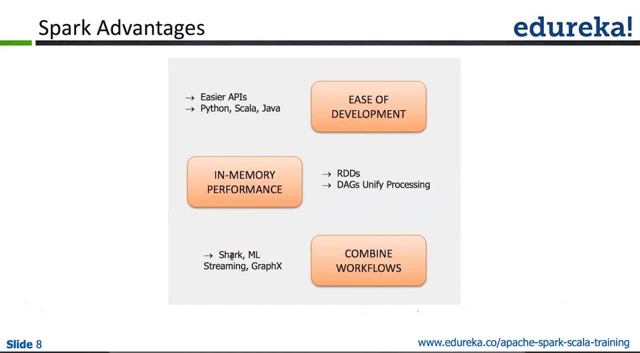 APIs, because of the support to the multiple languages, performance improvement, because you are talking about the in-memory data, RDDs and all that directed, a cyclic graph of your entire processing and other stuff, combination of workflows. well, yes, why not? because you are talking about graphics, sharp ML, streaming, things like that, right. 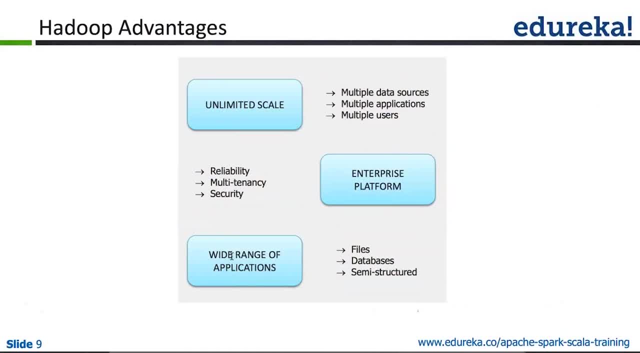 So all of these are the advantages of spark. okay, if I go to the next slide, it talks about the advantages of hadoop. right, some of the advantages again, you don't really need to be expert about it. unlimited scale: right, you need more processing power, more storage, just. 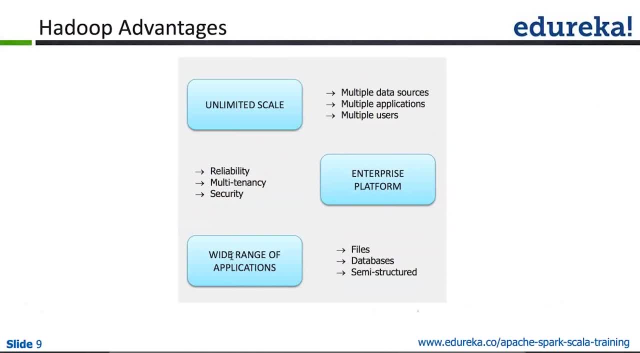 add more systems. basically, you are talking about the horizontal scalability. it's an enterprise platform. I don't need to talk about that. You already know that hadoop is kind of an enterprise platform already. it's kind of a defect to a standard for big data batch applications, altogether right. so over the period of time, 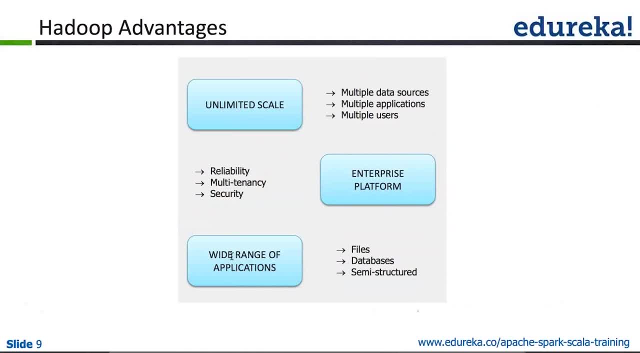 it has matured and the kind of security features, multi-tenancy and reliability features which have been developed are now quite tested altogether. and at the same time it supports wide range of applications- or I would like to replace the word applications- to wide range of formats. 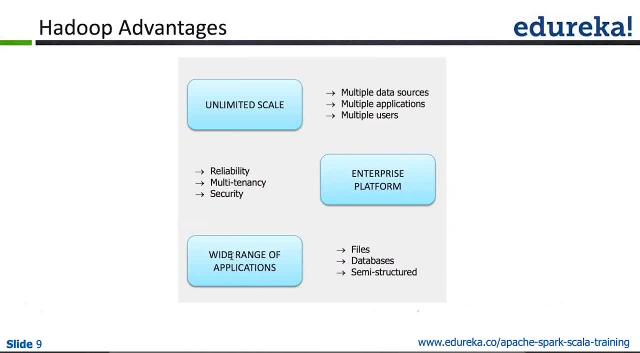 altogether. You might deal with the semi-structured data like XML, JSON, etcetera. you might deal with some sort of- you know- completely structured data or unstructured data altogether, or even you might be fetching the data directly from the databases also. So, yes, it gives you all of those advantages. they are very well known advantages. what really? 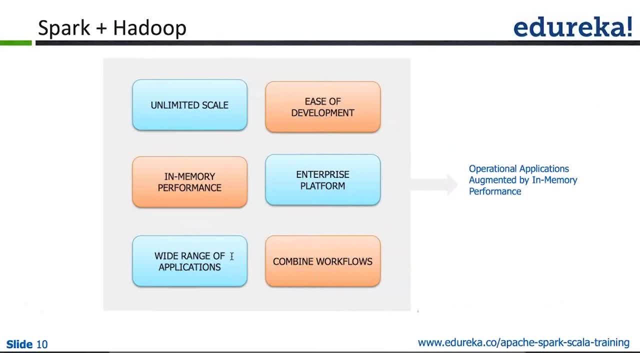 happens when you marry these two, and this is literally we mean by marrying these two, you get the ease of development at unlimited scale. You get the in-memory performance at the enterprise platform right in memory performance- fine. but the moment you have married it with the enterprise platform feature, basically you 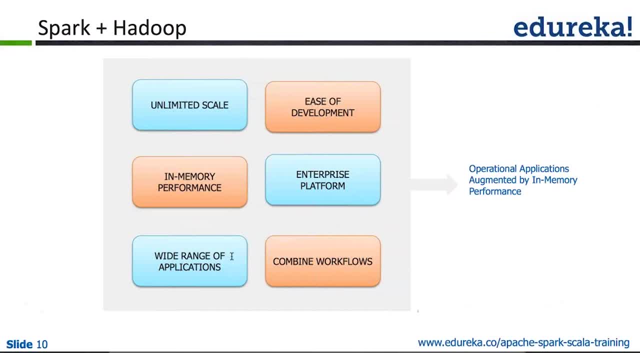 have got all the security and other features already for free. right combining of the workflows- fine, But remember your HDFS is supporting multiple types of applications. You get the ease of development at unlimited scale. you get the in-memory performance at the enterprise platform right: in-memory performance- fine. but the moment you have married it with 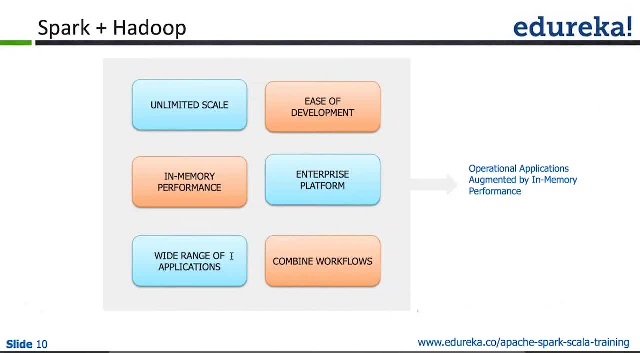 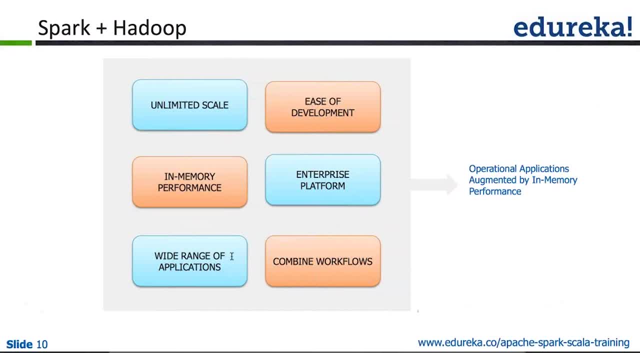 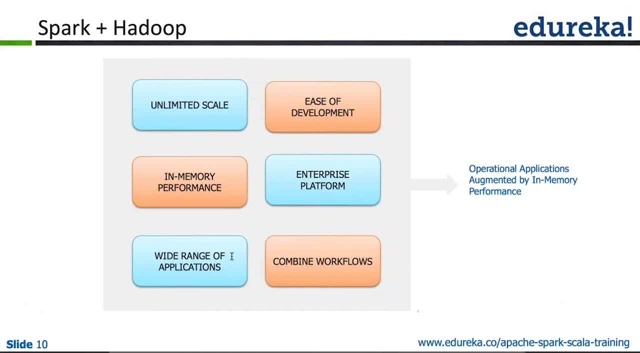 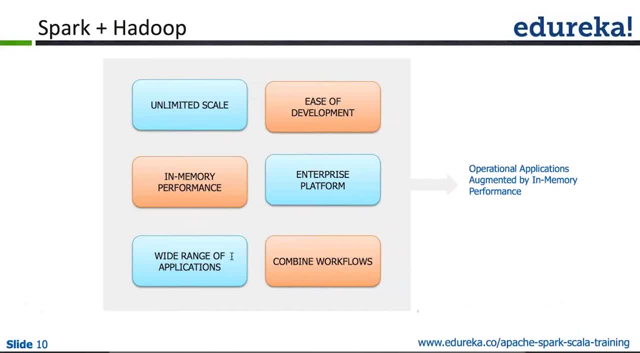 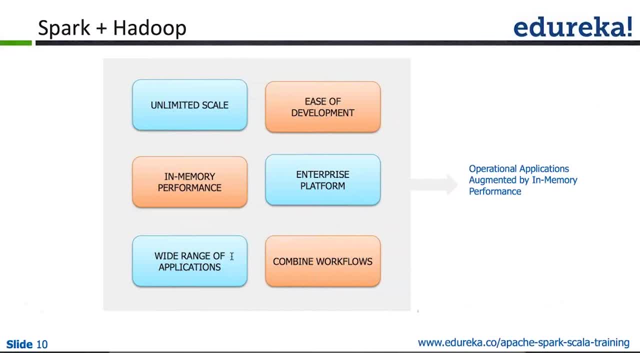 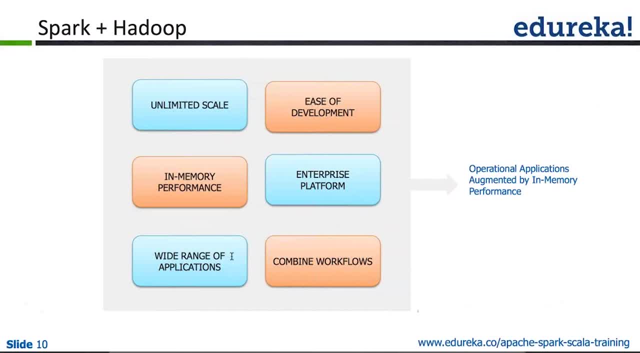 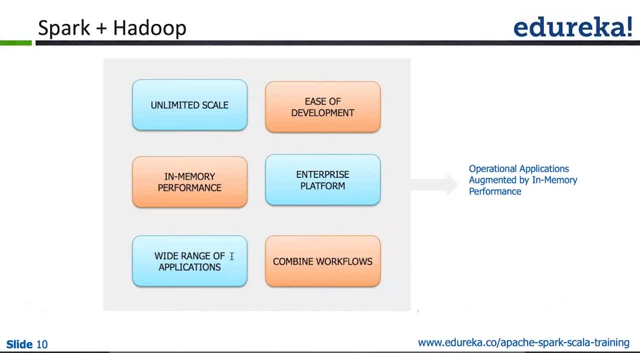 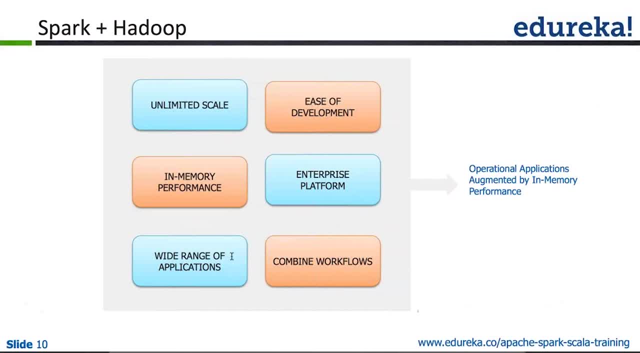 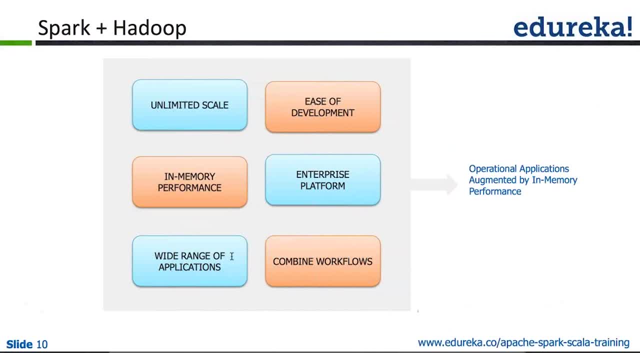 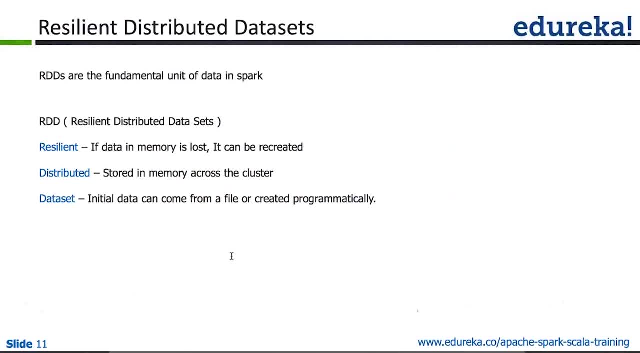 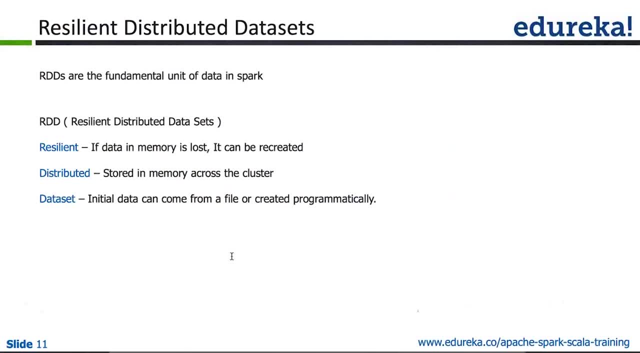 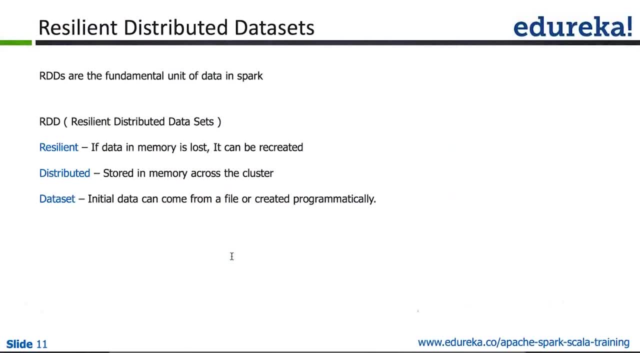 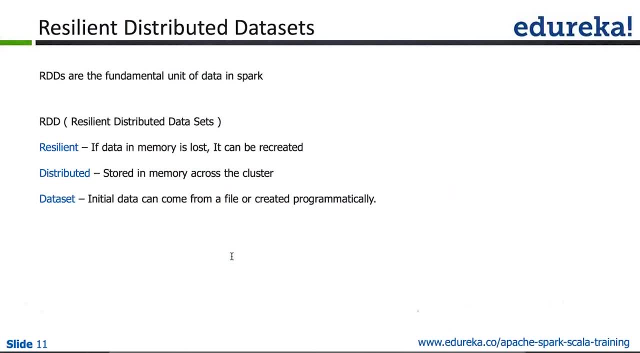 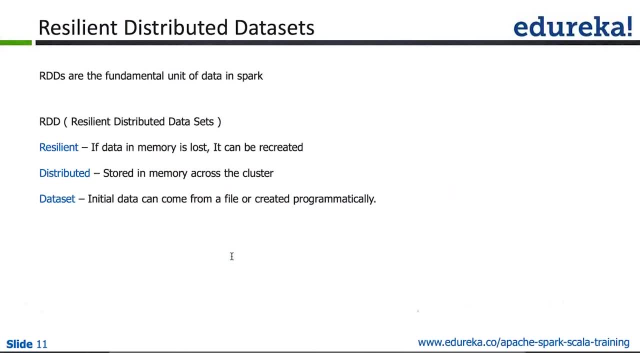 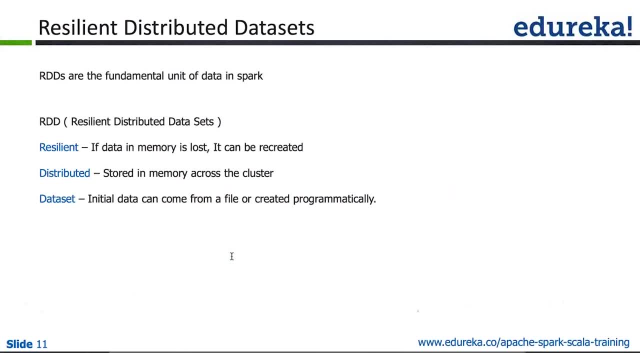 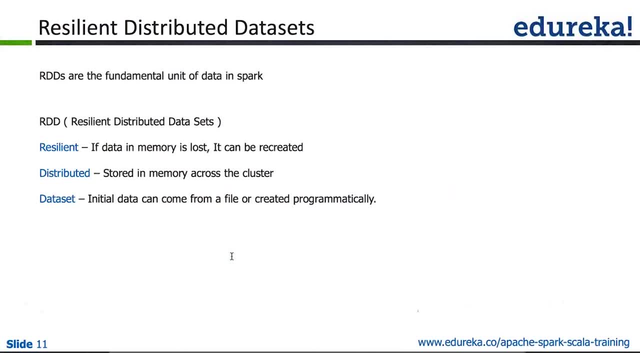 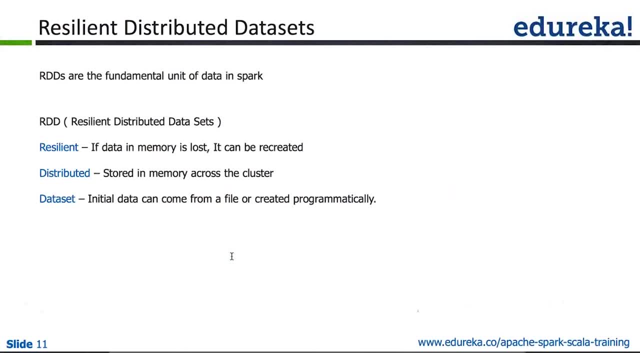 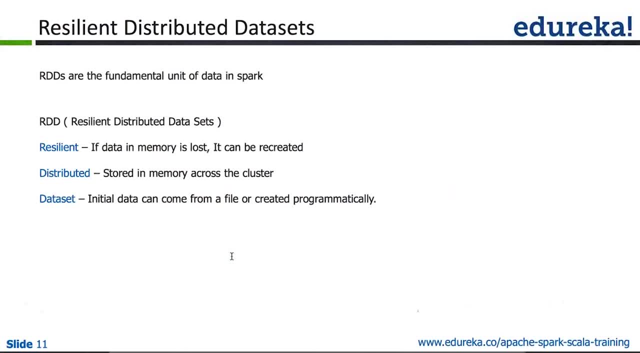 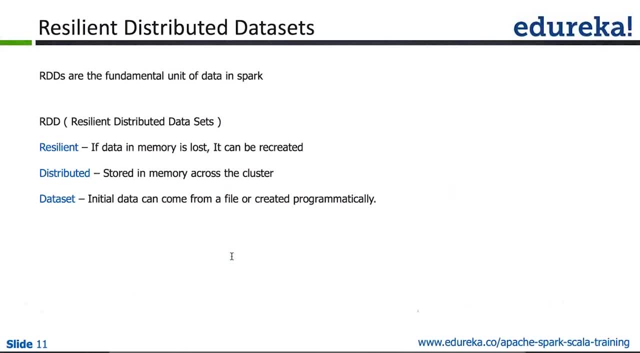 as I plan to do a bit of demo for you. is this okay if we, let's say, spend some more 5 minutes, or 5 to 10 more minutes into this webinar? I hope that should not be much of an issue with you guys, right? not more than 5 minutes or something. sure. my entire focus right now. 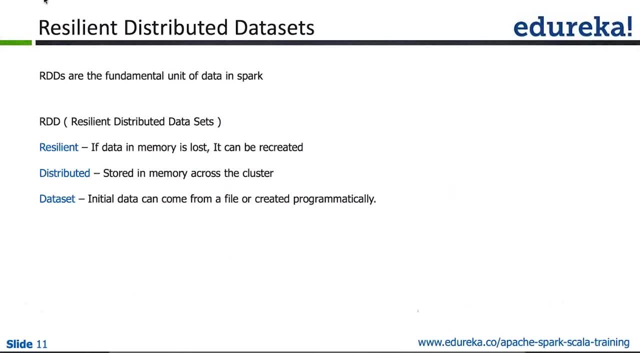 is to deliver something so that you can also understand. right, it should not be like very fast and you didn't understand much of the things. also, the next part is resilient distributed data sets. I would not go much because I have like touch based on this thing. just few slides. 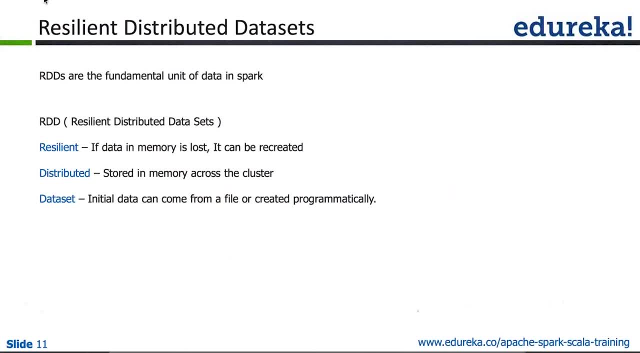 back resilient it's. it's called resilient, distributed. it's resilient because if your memory is lost, you can recreate it how, if you remember, I told you that spark is going to carry this entire directed as I click graph in memory. all together Right. so even if your data is lost, it will recalculate entire data. it is distributed. 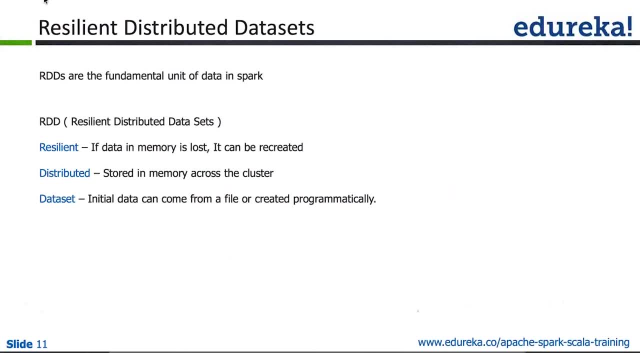 when I talk about it is distributed, because you know like your data is distributed across cluster and your memories also distributed. the next thing it is data set. well, I don't really need to talk about that. any data, whatever you are holding, is called the data set on. 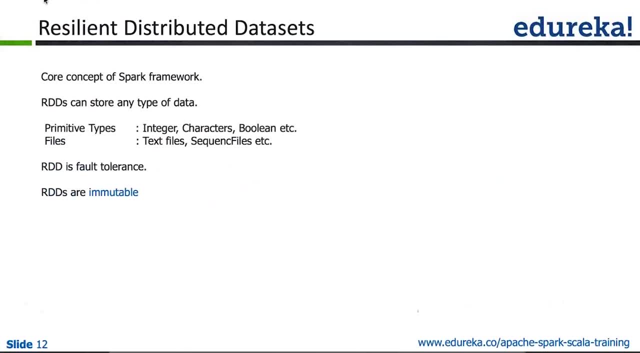 sorry all together. only thing is it is fault. tolerant, there's a best advantage. Okay, And I, as I told, what so ever you will do in spark, ever, even if you are saying one type one and enter: okay, that is also the RDD. okay, so it supports multiple things you want to. 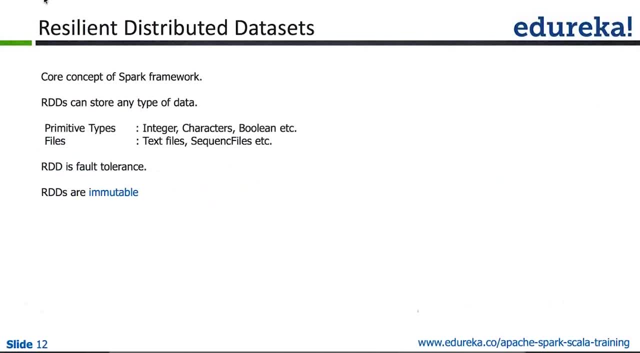 do some sort of primitive operations. you know those, those primitive operations, like your integers, characters, booleans. you just want to create them, feed them, do some operation. you can do that. you want to get the data from files, Etc. and do those processing. yes, you can do that. and, of course, all of the fault tolerance. 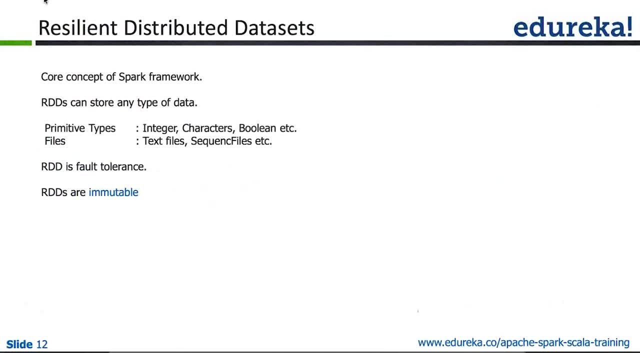 and immutability. at this point of time I would not talk much about immutability. just I will give you the pointer that, guys, immutability is something which is must if you are dealing with the distributed concurrent systems all together. okay so, and RDDs are, by nature, immutable. 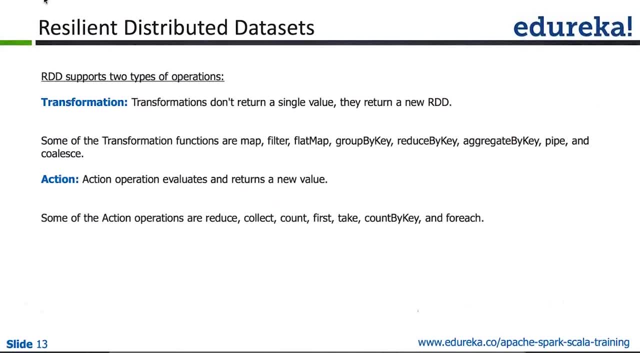 so they are thread safe, by the way. Okay, so just just I'm giving you the hints, because of course that's a longer discussion for the actual course, but just right now giving the seeds about it. right, there are typically two types of operations which RDD support. whatsoever you will do ever in spark will. 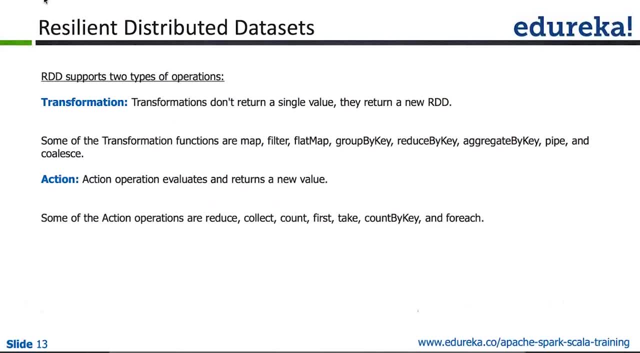 either be a transformation or it will be an action. so transformation it's like you know. I hope everybody understands What a transformation is. you are not doing any calculation, you are just changing the form of data. right, for example, you have all the names which you want to cover, convert. 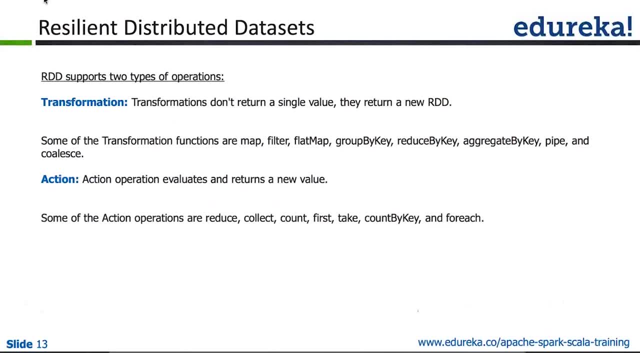 to uppercase. this is a transformation, and action is when you actually perform some sort of calculation altogether. so when I say calculation, you know, take all of the numbers, sum them up to a number and print it. now, this is an action, right? So all of the operations in spark can be divided into transformations and action, and we'll be 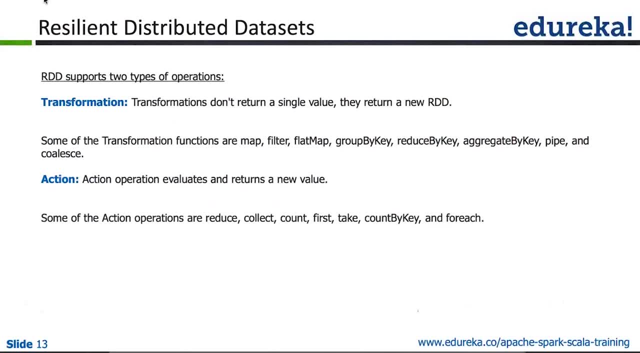 dealing with them, what are the different transformations, some examples of them, actions, some examples of them, and doing that in the actual course. in fact, in the small example which I'll cover today, I will still show you- I mean, you will not realize it right now- what has happened. 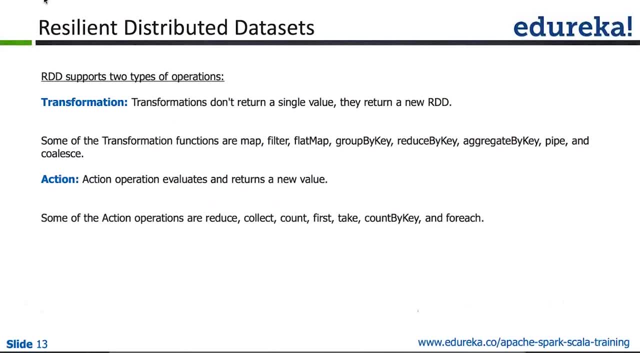 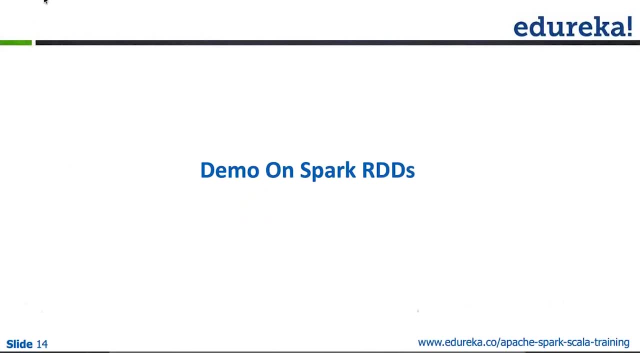 in a transformation or where did you perform an action? But even in the core, even in the code, today you will see a transformation and action happening in front of you. so I will still indicate okay. demo on spark RDD. time has come to do a quick demo, but I just want to club one more demo along with it that quickly talks about spark. 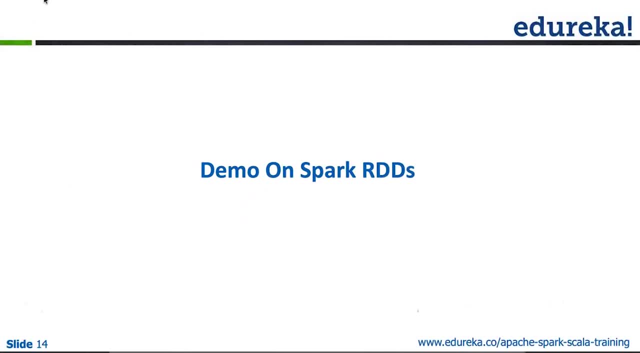 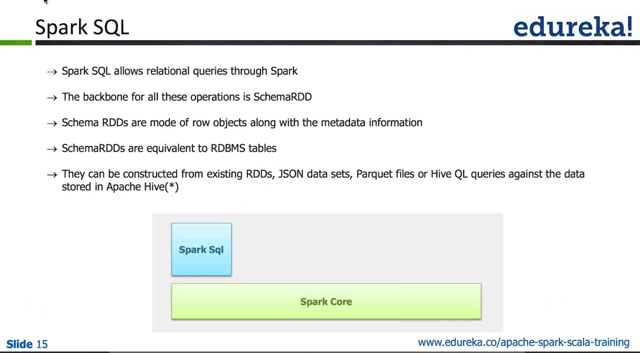 SQL, and then let me just combine both of the demos together wherein I should be able to show you the you know spark RDD As well. The spark SQL thing is that fine, right? so my only thing is, once I move to machine then I should be in machine, sort of okay. so I like quickly come back to the demo part in the 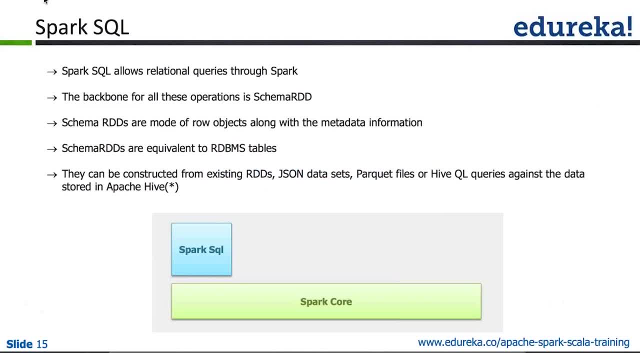 machine. I just want to give you a very quick heads up about spark SQL and a brief history about it. right and why did? why am I covering only spark SQL at this point of time? one, of course, the time is less. second, there are many people Who are coming from the background of data. you know the other data guys, SQL guys and 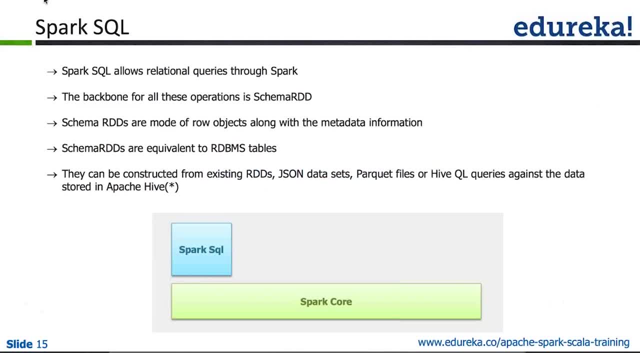 all and they typically say: how can I use spark? so we just wanted to address that problem, also assuming that there might be some people from that background in this webinar. okay, so guys, first thing, first those people who are from that background. you can always use spark SQL to write your queries to spark. we will even show you that there are various 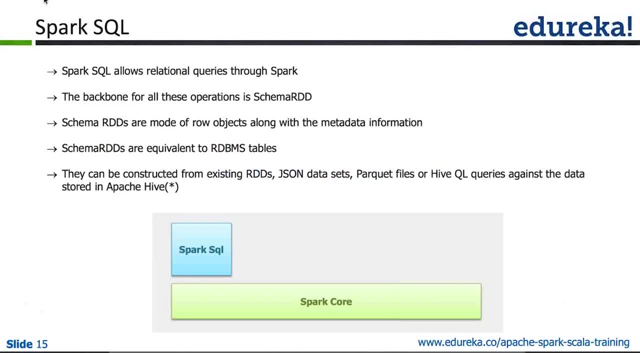 fashions You can use. okay, there are various fashions. you can use spark. you can either query the hive database directly, so you- you want to work purely with hive- create your database tables and all and then do the very quick analysis using spark. you can do that, you don't. 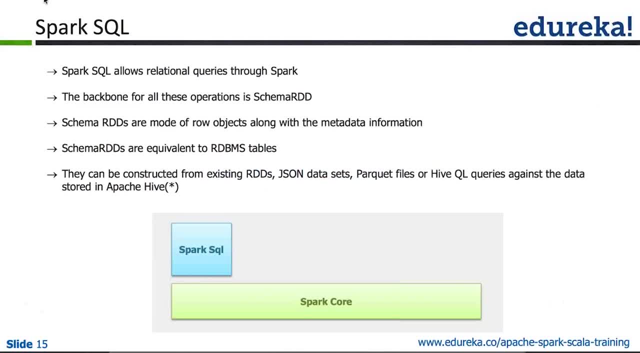 want to do this. you have some JSON files, you have some parquet files, you have some plain text files, right? any of them you have, you can still expose them as tables and do the query as you typically do. Okay, so that is. that is something which I would. I would show one quick example of it. 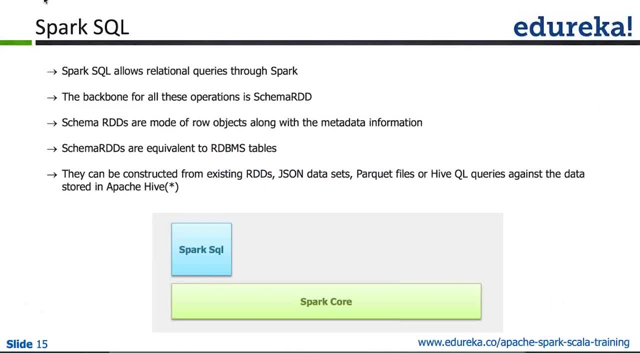 also. okay, I will show you one quick example of spark SQL, also in today's demo itself, but that would be just one example. there are many such examples which will be covered in the actual course all together. however, the backbone of all of those operations is schema RDD. so 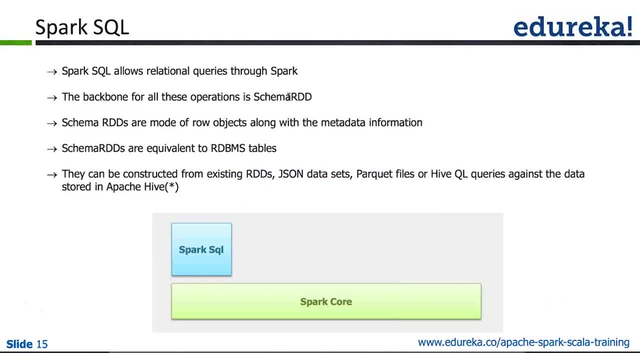 as I told you, everything is RDD, just that schema. RDD is a different class in Scala which lets you schema like operations wherein you know you define some sort of table structure and do some sort of SQL operations all together. I would just limit it to that and would go. 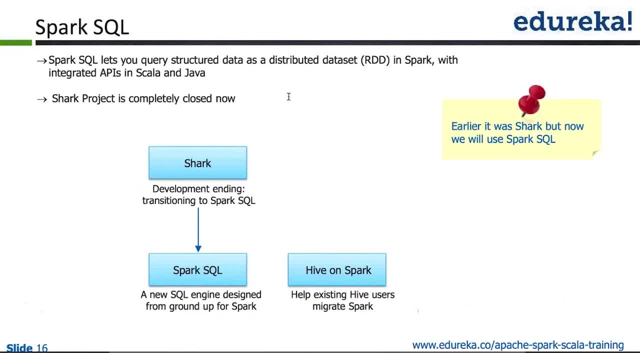 to actual hands-on part itself, rather than talking merchant or you know what is, schema, RDD and other stuff, because that's a very long topic all together. A bit of history, guys. so spark SQL, I'm sure I'm assuming that many of you would have done. 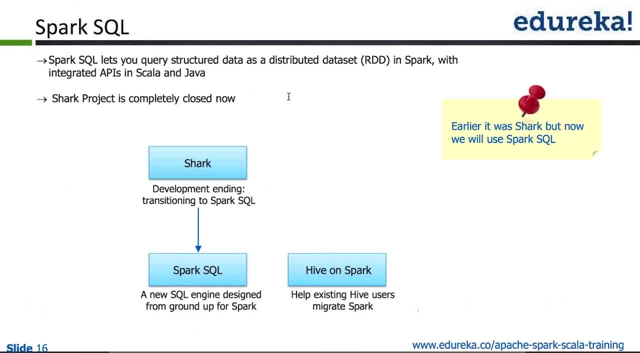 some googling. all of us are smart enough. you must have done some sort of googling, and then we are coming with some backgrounds all together, right, some of you would have heard about shark, or some of you must have heard only about spark SQL, or some of you even have heard both. 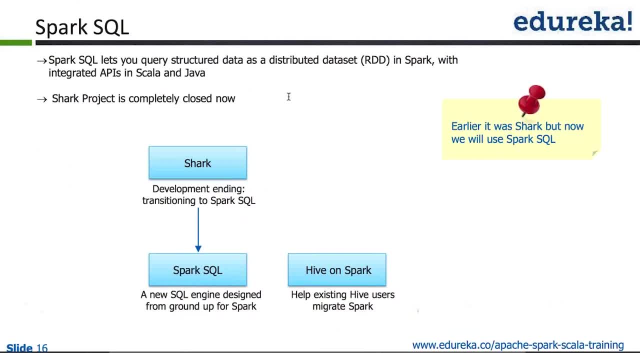 of them, right? so let me just tell, shark was the actual project which got started at Databricks. okay, Databricks is the main company which has actually worked towards spark, and then they have donated this As the open source project to Apache community and now it is being incubated and actually 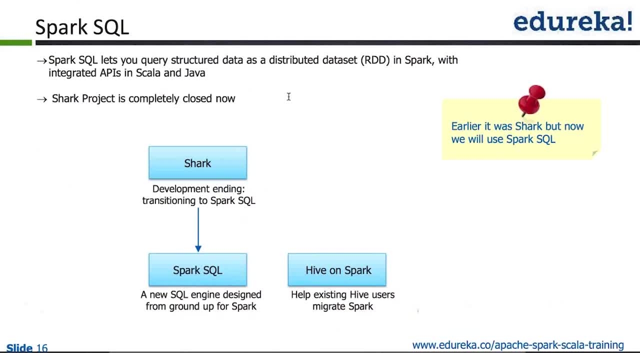 it is now the top level project. so they, when they were working on it, they called this project, which basically integrates with the, you know, hive and it is supposed to expose the data in SDFSS tables and do the queries, and all they were calling it as shark. okay, now when? 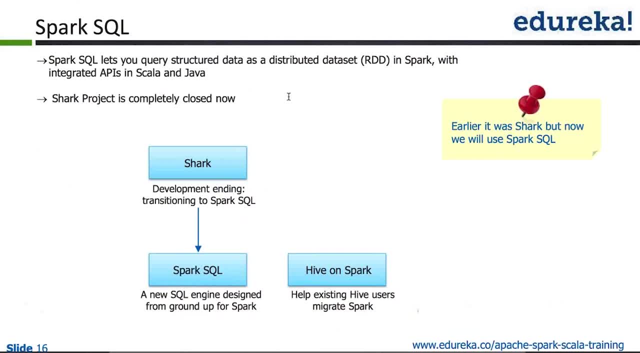 it got adopted in Apache community. there are wider people, There were wider issues and people had to reprogram it. people had to rechange its apis, even architecture also, and now it is no more called shark, it is called as spark. SQL name has changed, apis have changed, so the shark apis are no more valid now and shark project. 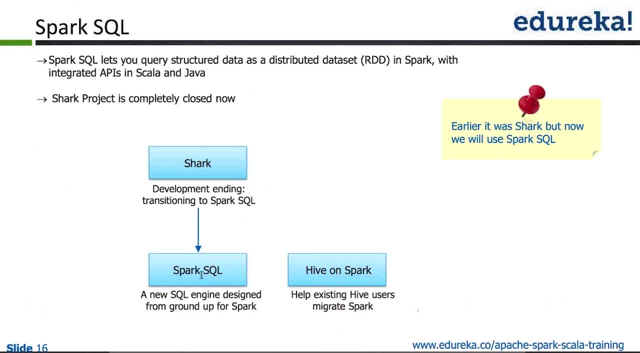 is closed. okay. however, the current support still goes on. there are People who are still supporting shark, but it is no more valid because, as I told you, just few months back now, they have integrated. just two months back now, they have integrated hive with spark SQL, and that is where people have said now shark project is closed, so hence. 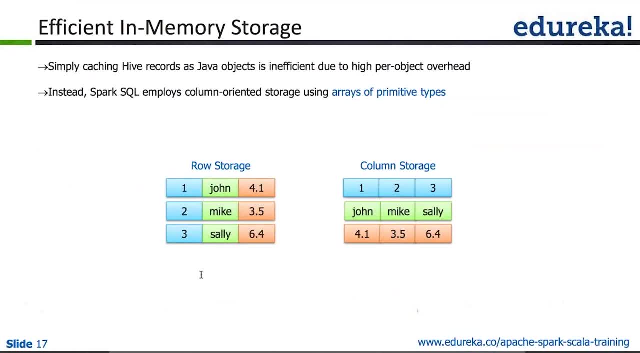 those people who have heard about it. please do not get confused. spark SQL is the. it's the successor of shark. okay, This is just a history bit I just wanted to give you efficient in memory storage. let's not talk much about this topic. all I would just say is spark RDD basically goes for the. 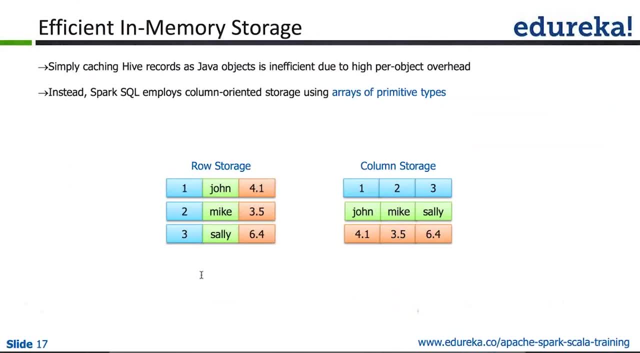 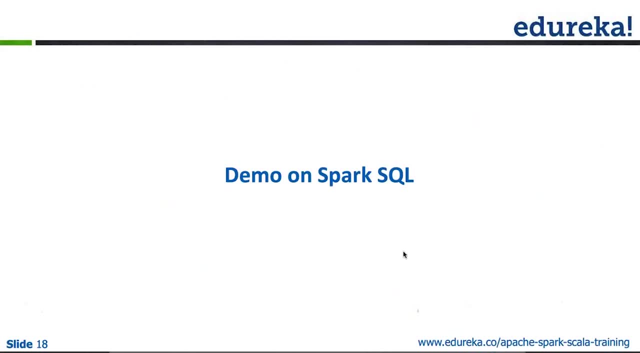 again, everything has to be in memory, so it just changes your data structures a bit so that they are better suited for in memory storage. I'm not going into that detail right now, and with that I would like to move towards the demo part. Are you all guys? 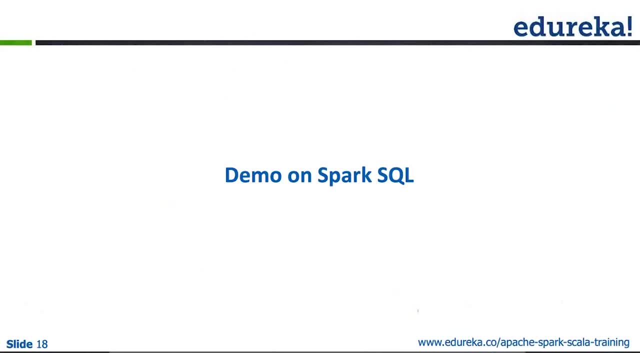 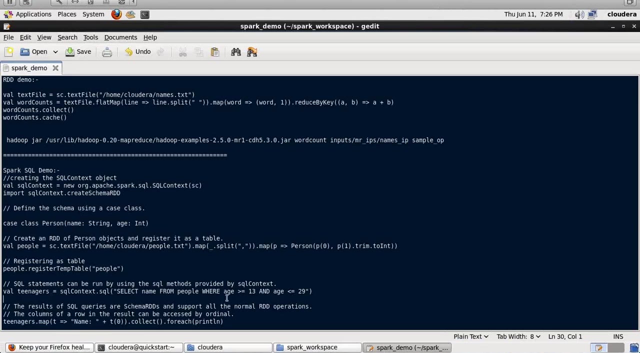 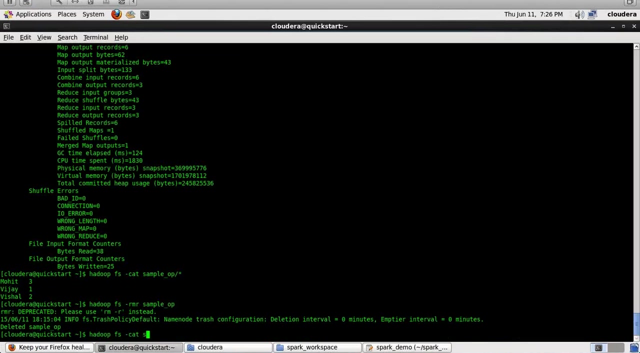 Okay, Are you guys interested into that? let's have a quick thing in the demo, right? okay? so with that, let me just open my machine and before I start my demo right, just a second. guys, always make sure that before the class everything is, or? sorry. 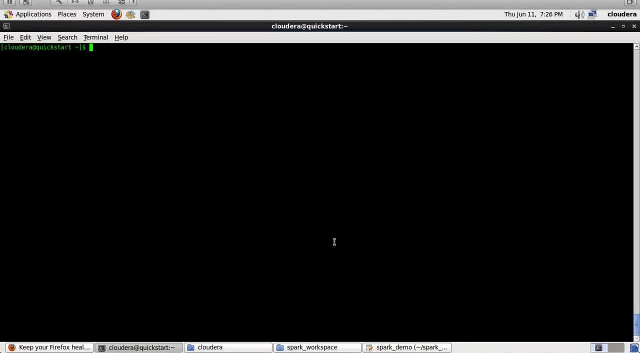 So called class. before the webinar. everything is like up and running. this is a virtual machine, which is CDH 5.3 here. the best thing with CDH 5.3 is you have got spark, Hadoop and everything pre integrated. okay and well. spark is a very active community. when I say active, there is. 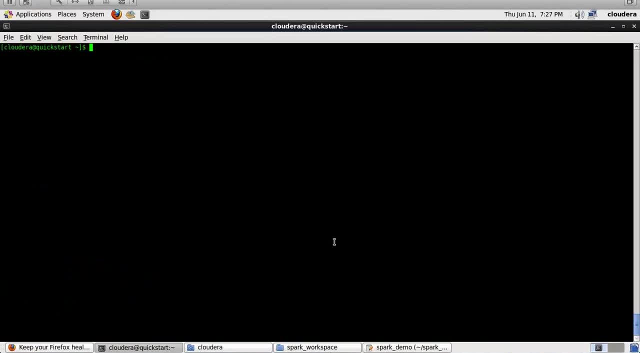 a lot. every two weeks you will see one more release, you will see one more commit happening in spark. So it also means that whatever you are doing might not be valid. let's say valid means that same version compatibility issues might come, so we typically suggest to use, you know, these. 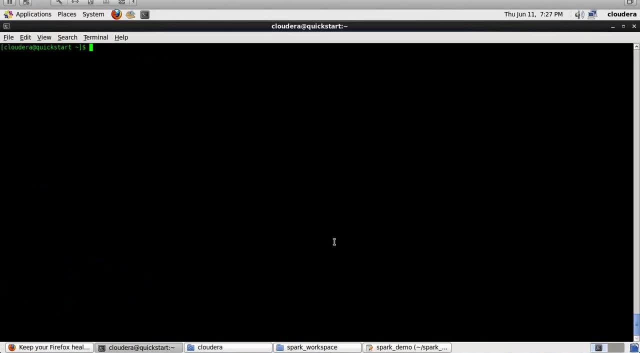 kind of package machines wherein you don't really have to struggle with the versions. okay, that Scala version should be this, Hadoop version should be this, your spark version should be this and then spark sql version should be something else. that way you will save yourself from the hazards. 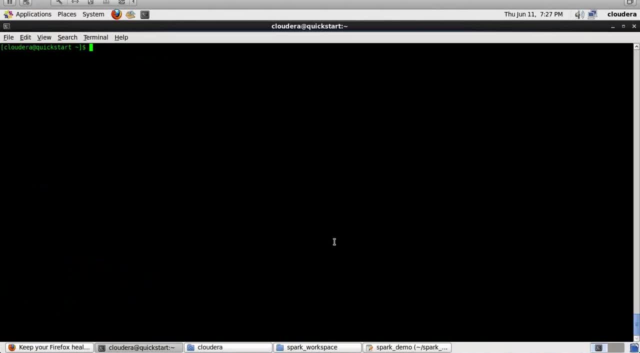 Of you know putting all the things manually. that is first thing, which will be very important, and, at the end of the day, cloud era is again one of the most talked about or one of the most prominent distributions of Hadoop also, so that's where we have chosen this platform. 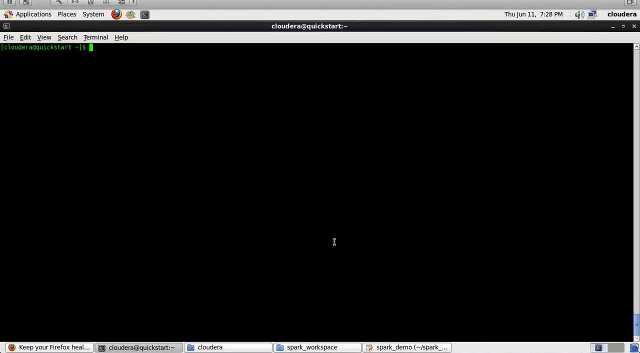 which is quite reliable also. now, this is about the platform. now, what am I trying to show you? so you must have seen two slides. one is a demo on RDD, and then there is a demo on spark sql. let us focus on the first thing. demo on RDD. so, guys, what, what will you gain? 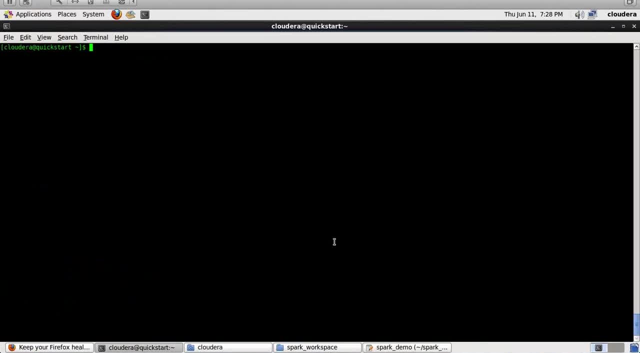 if I just show you that guys, see this, this is how I work with an RDD, how will you compare it? right, you need always a comparison. if I am telling you that, guys, you should use spark, I should be able to tell you why you should use spark. so is it a good idea if I run a? 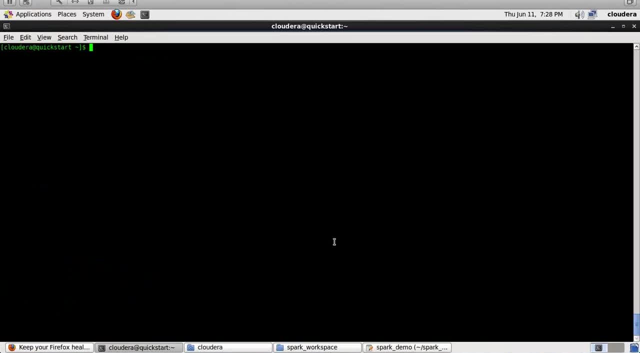 demo. show it the output, run it in front of you with the same amount of data. show you the execution time. and now I run the spark program on the same data. okay, on the same data and just compare the running time on the same machine. looks exciting, looks like. 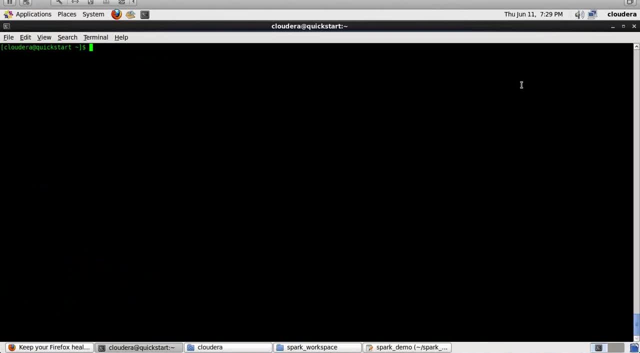 a very valid kind of a you know thing which we are trying to compare. Right, guys, make sense, right, when I am showing you, I should definitely be showing you the comparison, not just one side of story. okay, with that, with that, let me just show you very. 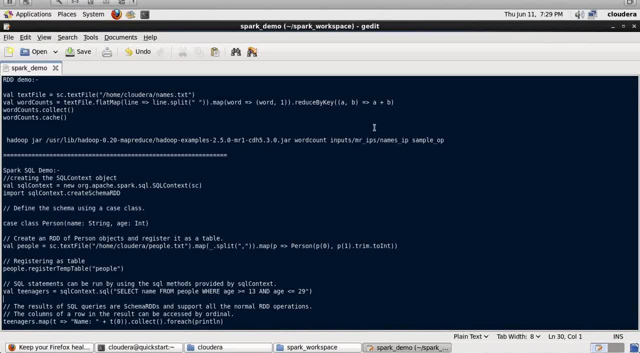 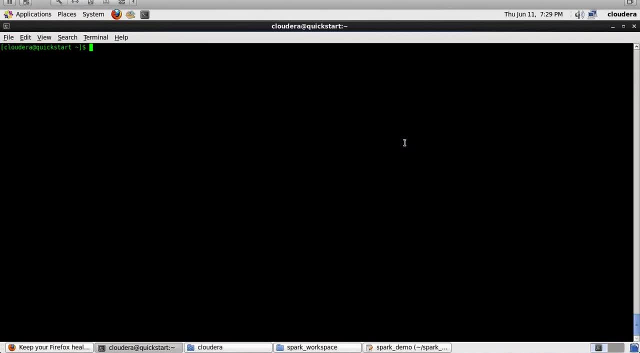 quickly, okay, so guys hold on. okay, So you can see. there is this file: Hadoop fs-cat. I am typing, so it is of course the HDFS. okay, you can see this. there are only few names: Moit Moit Moit, Vishal, Vishal Vijay. 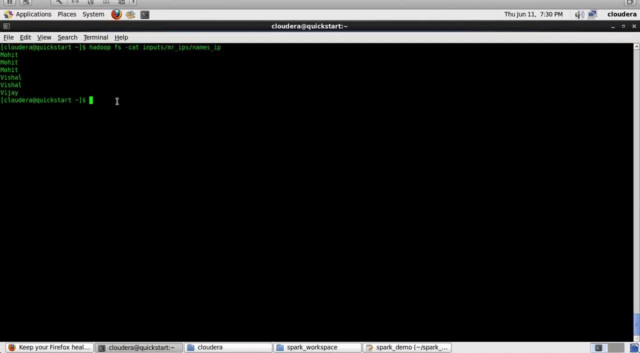 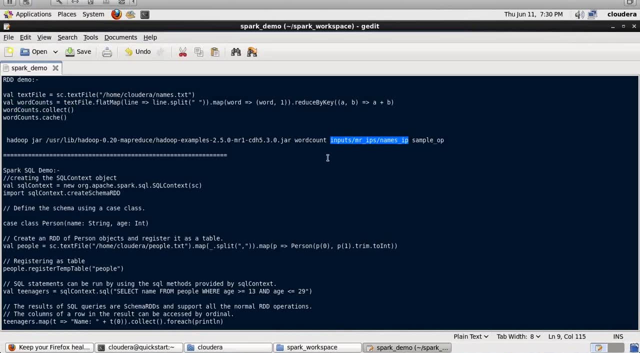 right, these are just few names which are available here right now. I want to do was you know, ages, old word count, So of course I am not going into the code, I am just using it, that pre-packaged Hadoop example right now. the idea is, the focus right now for this exercise is to show you the difference. 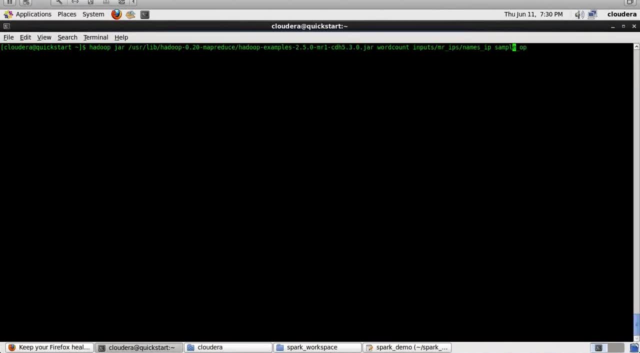 of execution times. So this is how you fire a typical MapReduce job: Hadoop jar. then the location of the jar. you can see that this is the pre-packaged Hadoop examples. jar word count is the program which I am firing. inputs MR. inputs names: 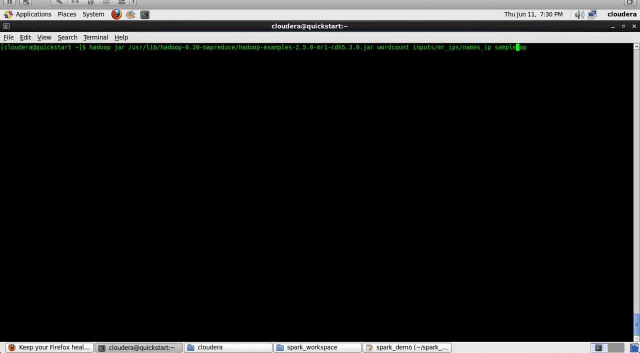 So this is my input location and this is my output location. is that clear to everybody what I am trying to achieve right now? step one, right? I hope step one is clear. let me fire this. so this is firing your MapReduce job. it has connected. you can see this job. 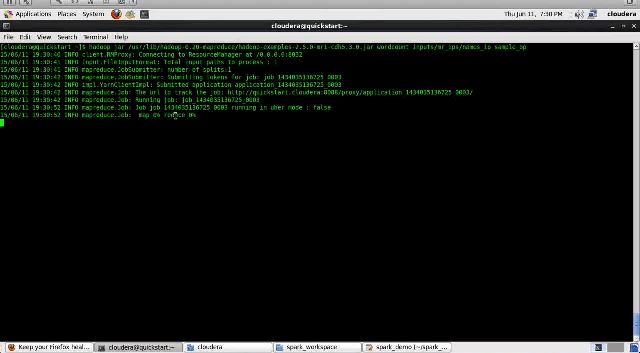 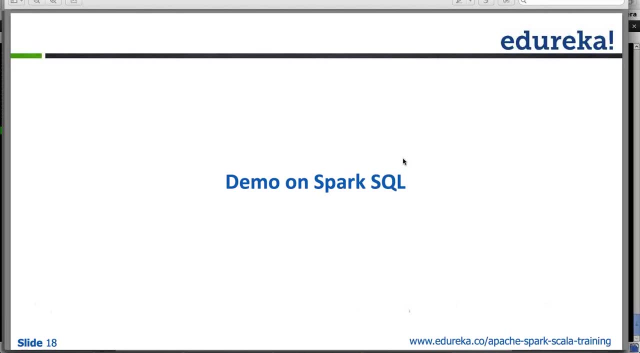 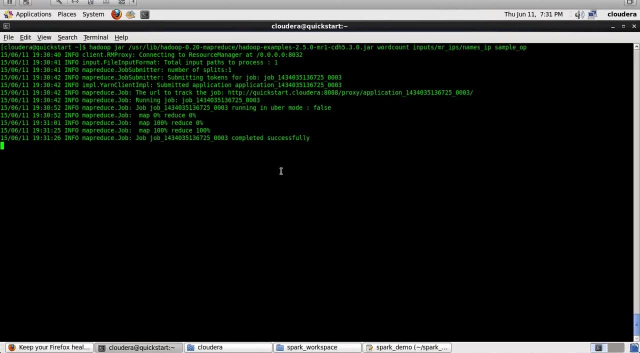 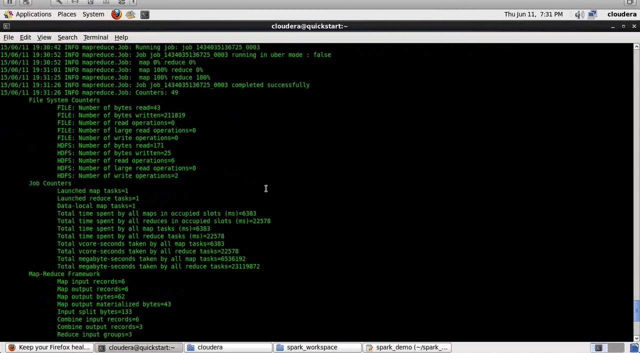 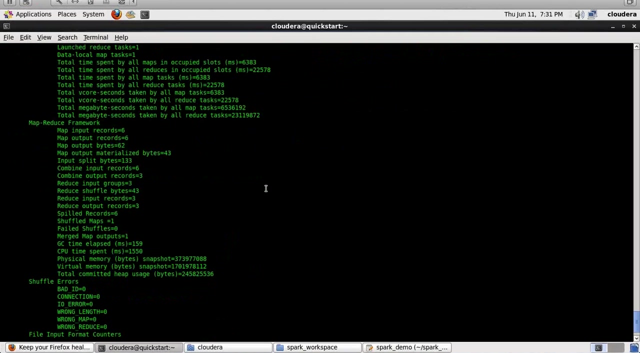 underscore this: it has now fired the MapReduce. ok, by the time it runs. let me just be ready with ok, so got over. you saw the time also right. it took few seconds, right, I think. you think if I am able to show you the time somewhere, that's fine, but all of us know that it took. 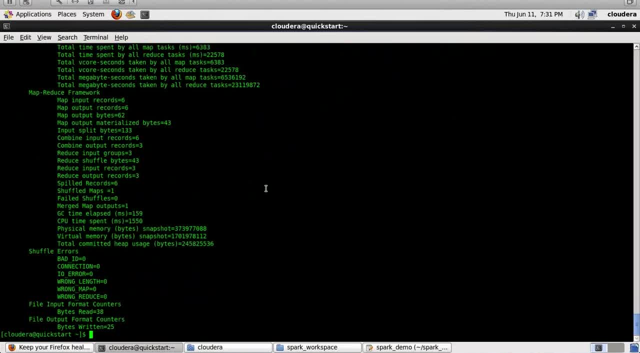 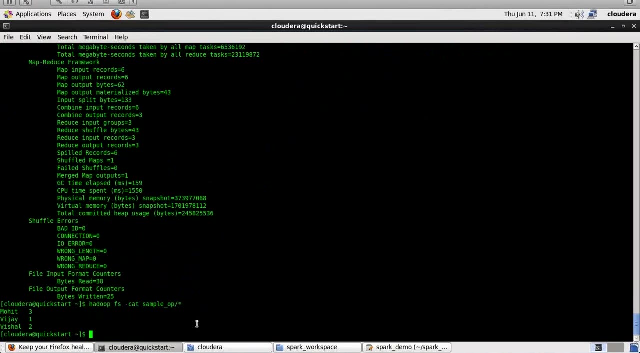 almost kind of 10 seconds to 15 seconds, 10 to 15 seconds overall when I fired the command. let us see the output right: Mohit 3, Vijay 1, Vishal 2. so far, so good. Can you please quickly confirm? so you have just seen a MapReduce job being invoked in. 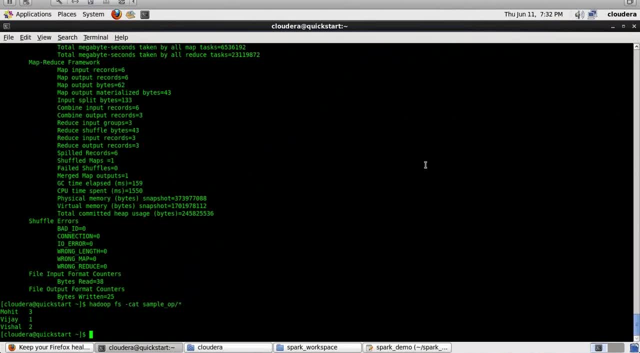 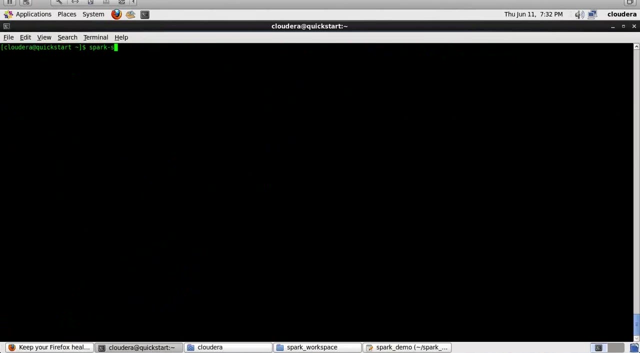 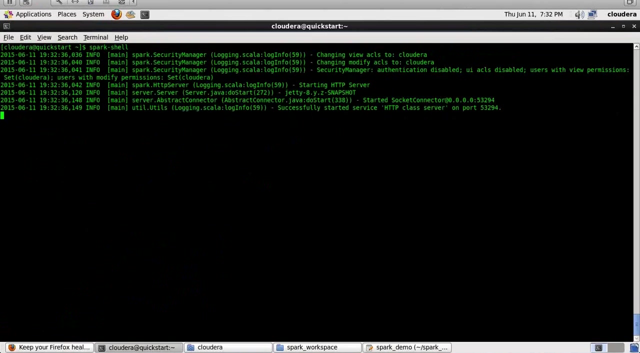 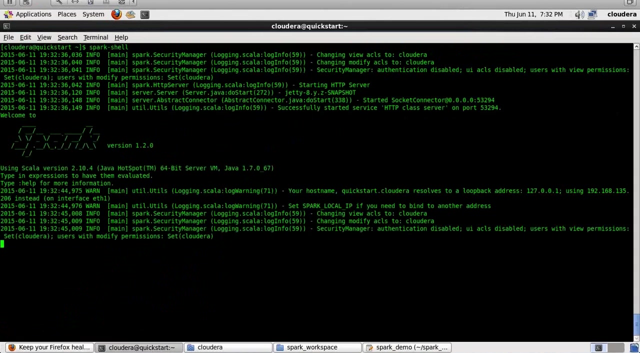 the conventional way, right via Hadoop. I fired this job. I am going to fire the very same job now. let me just clear it up. now let me fire my spark. ok, now I am firing my spark, so spark shell. When you say this, It will fire the shell for you quickly by the time it fires. let me just show you what. 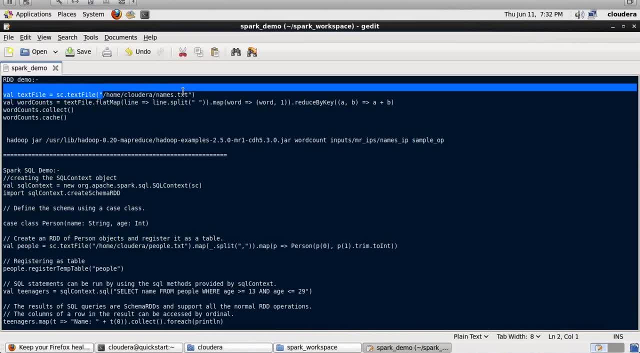 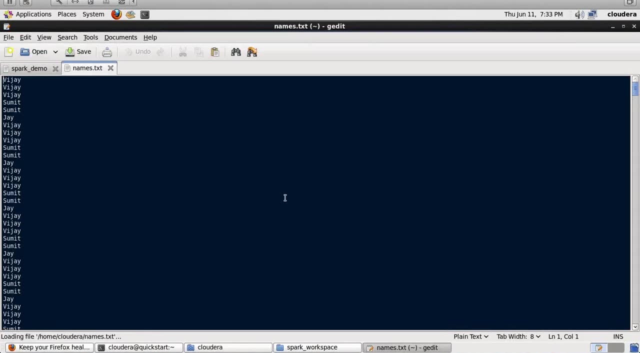 I am trying to do so, guys. I am going to load the very same file names, dot txt again. ok, let me just show you the names, dot txt also, so that you are like a bit comfortable here and you can see this. such a big file, See this, it's such a big file. that was only 6 words and this is- this is 1056 words- are. 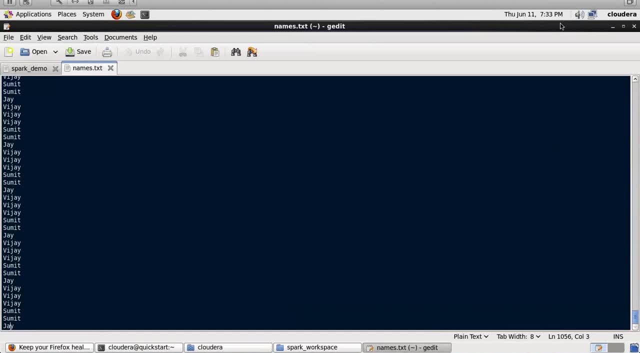 you seeing this? I have increased the load many times, hundreds of times more. have you seen this, guys? I just want a confirmation, all of you seeing that 1056 words are there. the previous one was having only 6 words. See this. it's such a big file. that was only 6 words and this is 1056 words. are you seeing? 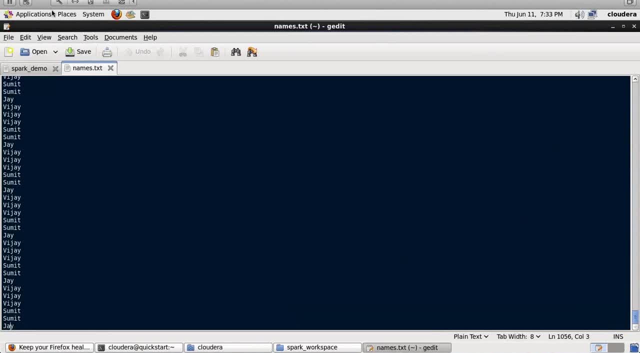 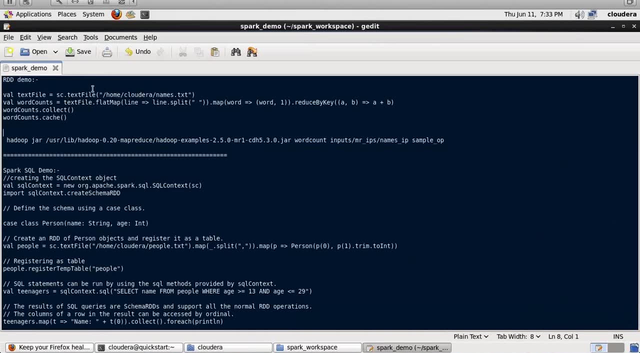 this guys. I just want a confirmation, all of you seeing that 1056 words are there. the previous one was having only 6 words. right now, let me tell you what I am going to do with it. I am just closing it, so I am loading this text. by the way, this is the word count. 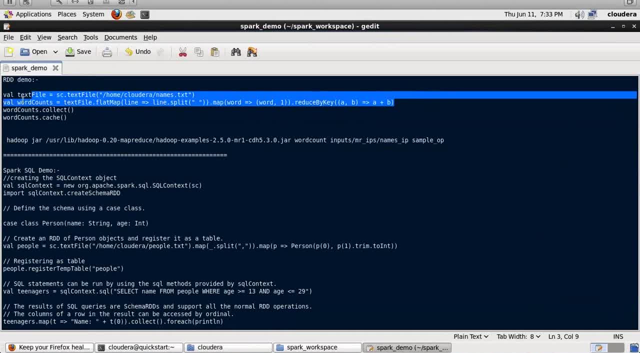 program in Scala world or for spark. this is the word count program. all of you who have ever worked with Java, MapReduce, you must be knowing how big a program word count is right. How big a program it is, depending upon how do you code. it might be as less as 60 lines. 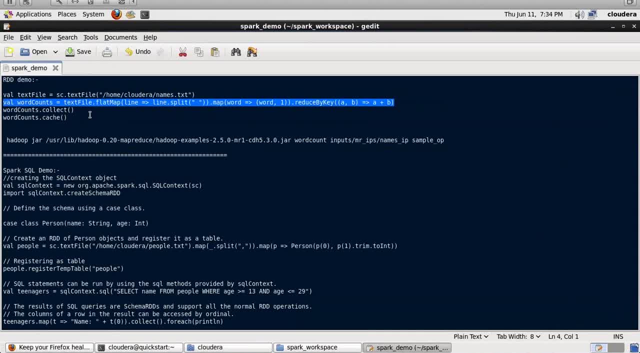 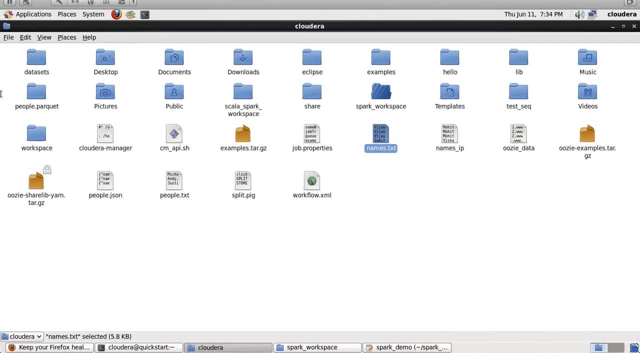 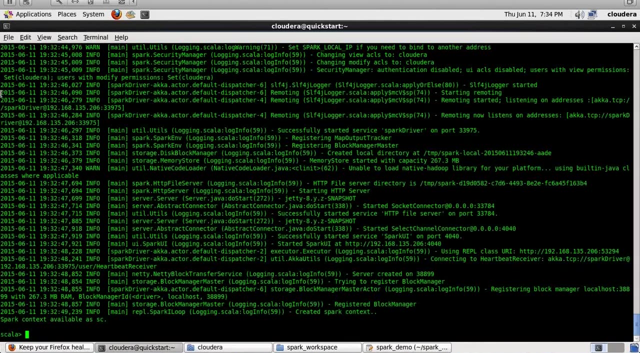 or as high as 100 lines. right, so that is it here. it is one line. now let me do the things so you don't really need to understand right now the syntax. that will be unfair. right now I am just loading that file into the memory right now. this is just the. 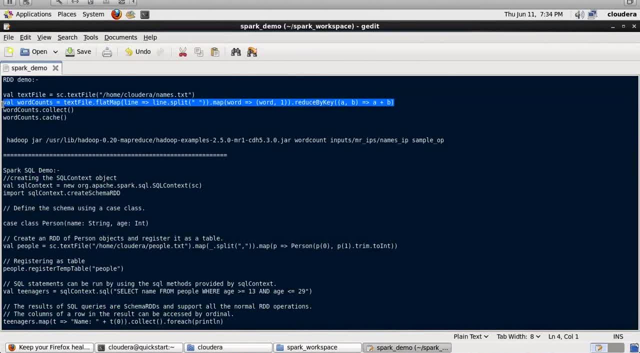 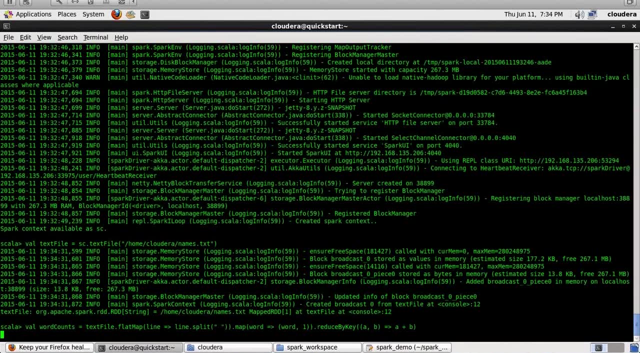 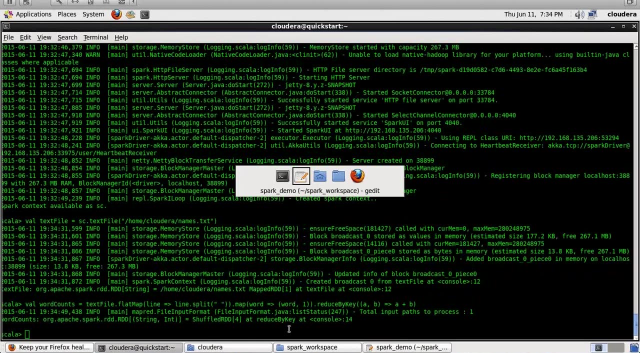 File. whatever I am going to do this, I am just telling you after this. okay, so this is the place where, in I did a transformation. I have not done any action. whatever I am going to do now is the action. okay. so this is it. when I say word counts, 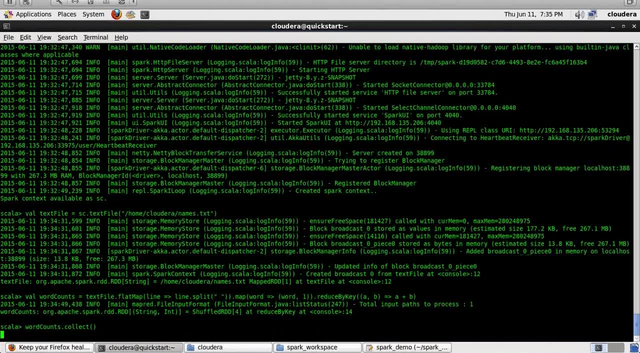 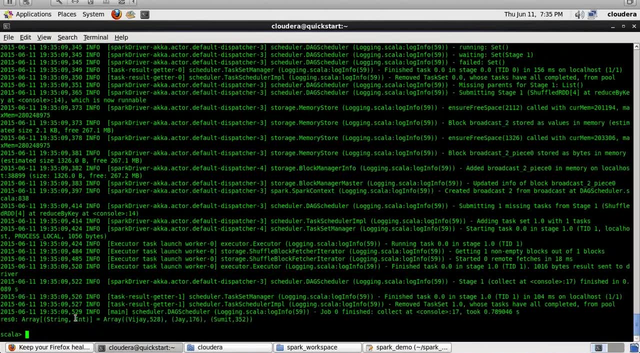 Select and press enter. done, guys, done. see this. Vijay J Sumit: 352 528 176. see the time: 0.789046 guys. it's right in front of you. saw that my load Is. My load is at least 100 times more and my performance is 100 times faster. saw that, guys? 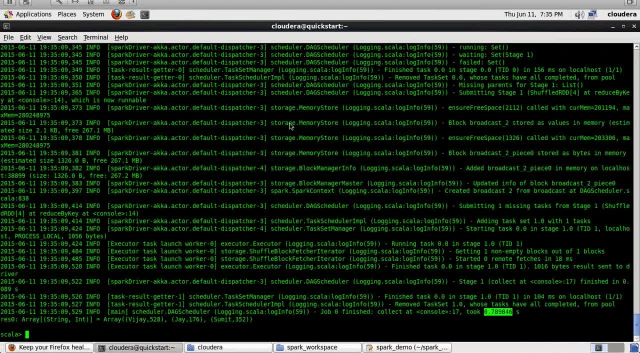 quickly. could you confirm? and how are? what is the impression? right? so I went to the both of extremes right at the same time. same machine. I increase my load 100 times right? actually, this 6 divided by 1056, you can find out. you know, in hundreds of times I have increased it and this is the same machine. 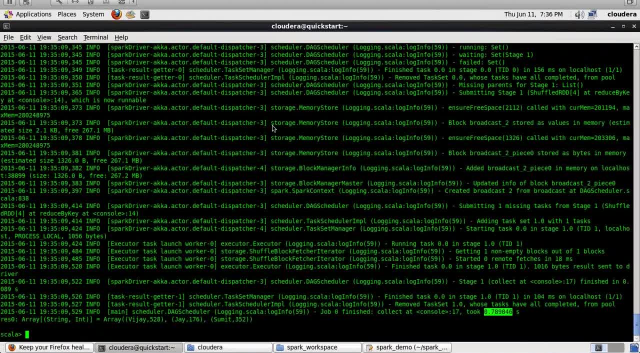 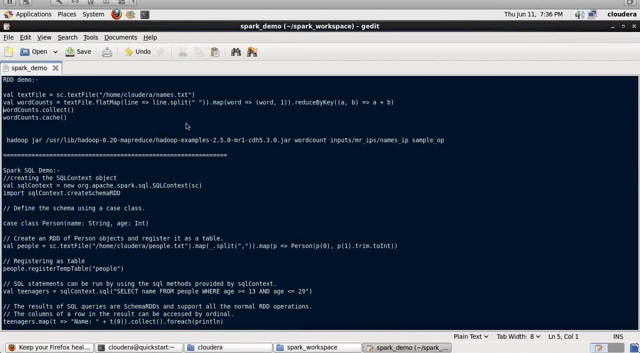 Nothing has changed, Right. so this is just one thing, guys. I just wanted to tell you right next, a very quick demo about Spark sequel also. okay, I again, please don't focus much about the syntax as of now. it is unfair, but let me just so what I'm trying to do. I am having a file. okay, people dot txt. I. 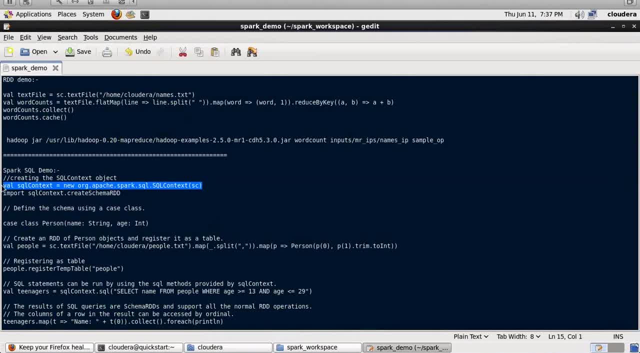 will expose it. what I'm going to show you is, let us say you are coming from SQL background and you have got a file. your manager comes back to you and says: can you just do a quick analysis on it, on this file, to me, exposing it as table. 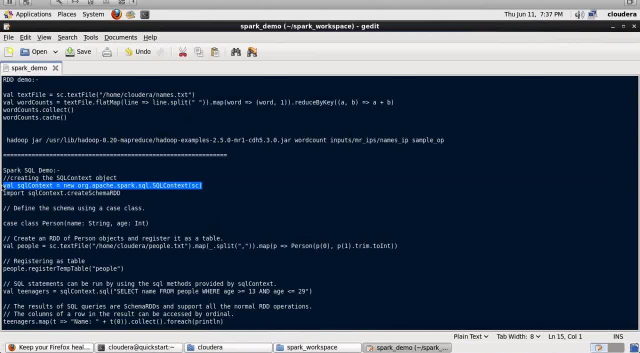 and you spark. let's say, if this is the scenario, how do you do it right? so this is something which I'm going to do now and, well, guys, this is something SQL context is something which you have to create. okay, so please just bear with me for this thing. right now, this must be. 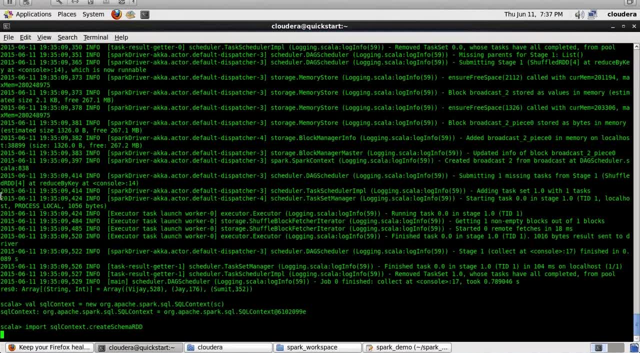 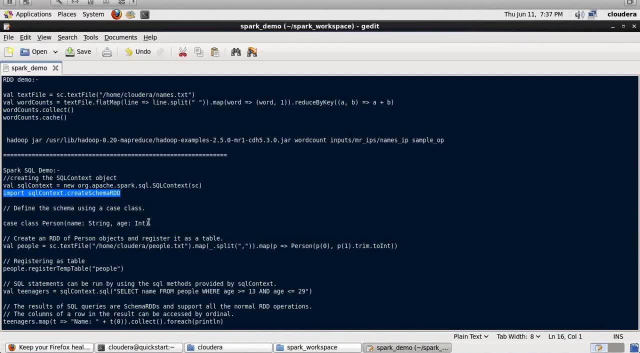 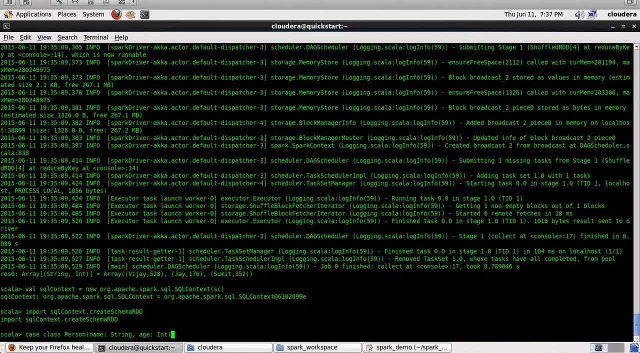 seeming new to you. then, SQL context dot. create schema RDD. it's a class which you have to import. okay, this will tell you that. yes, whatever you are trying to do now is kind of a you know thing wherein you are able to create the schemas and all. then I have. 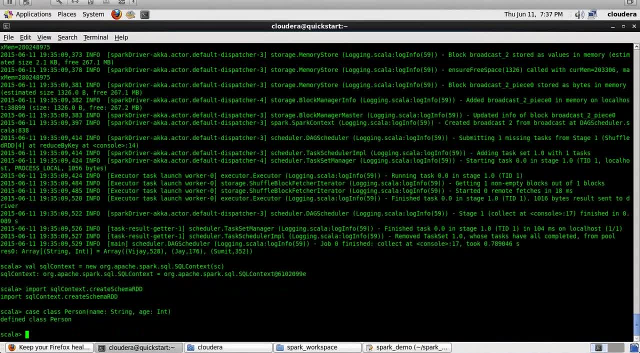 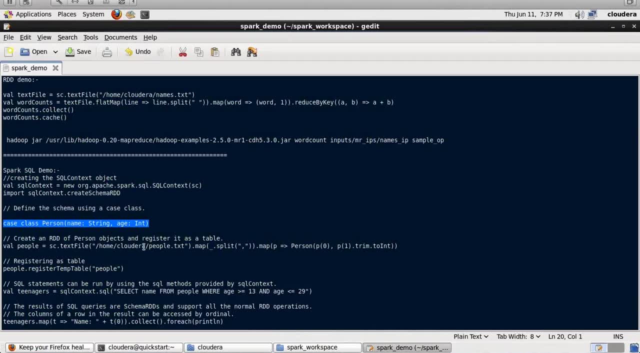 created a class person which has only two fields: name and age. name and age, nothing else. okay, now you can see there is a file: home cloud era: people dot txt. let me quickly show you people dot txt. okay, so, let me show you people dot txt. okay, so, let me quickly show you people dot txt. 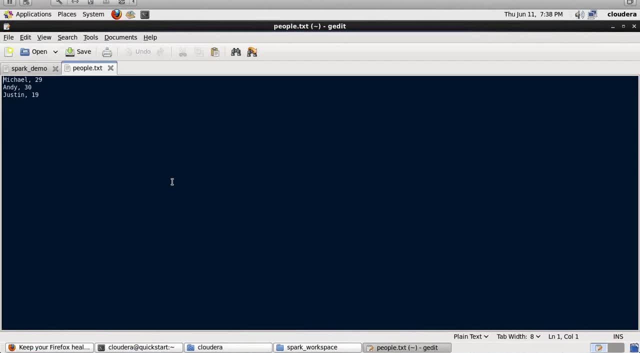 okay, so let me quickly show you people dot txt. so, Michael 29 nd 30, Justin, 19. right, these are, let's say, only three records. so, Michael 29 nd 30, Justin, 19. right, these are, let's say, only three records for you which you want to. so you want to expose this file as a table altogether? 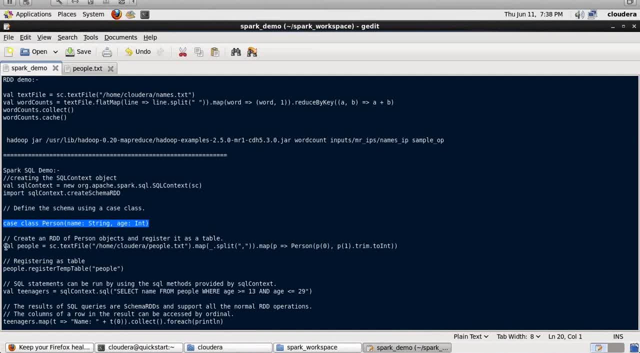 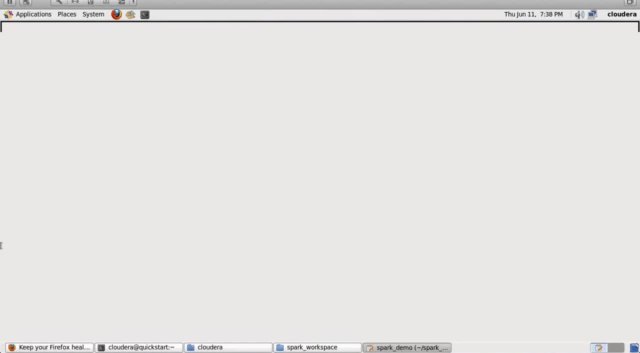 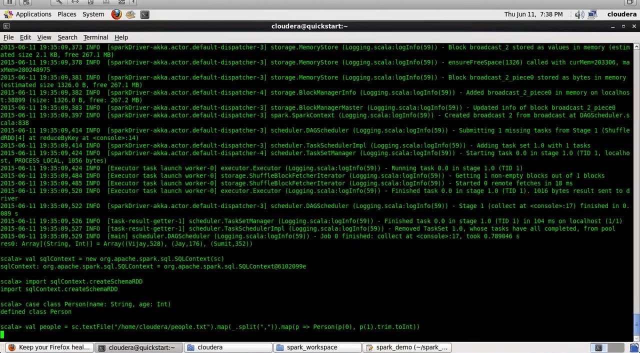 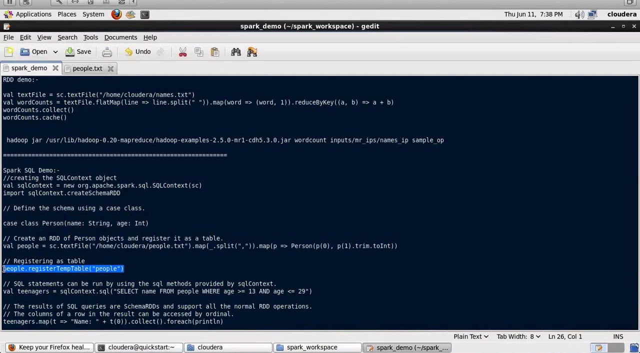 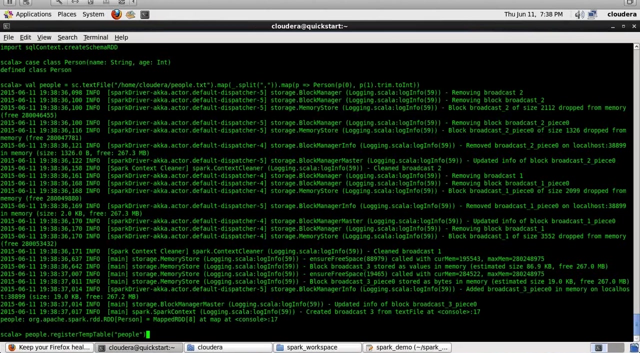 okay. so what I'm going to do is, with this statement, hold on with this statement- I am going to expose this file as a value, people, and then I am going to register this value as the temporary table. see this: people dot register table. people enter now my data. 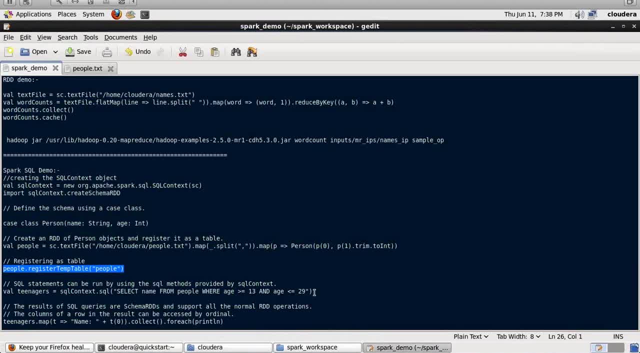 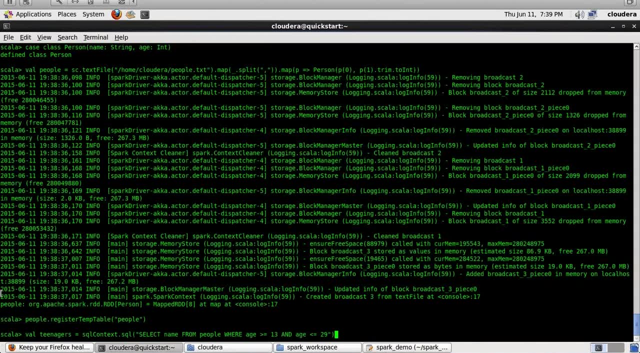 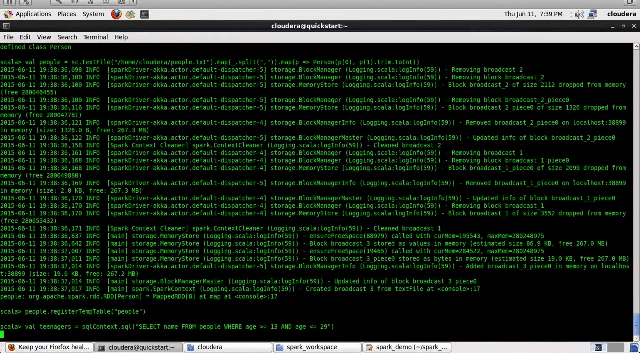 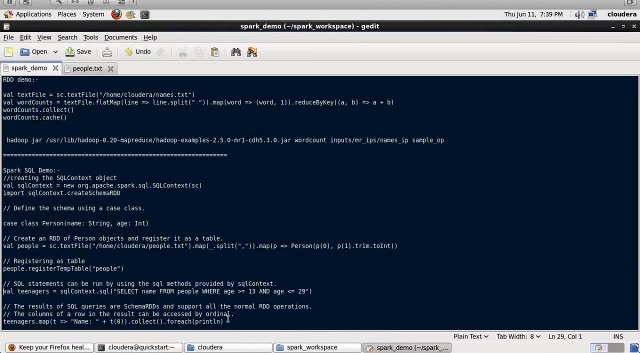 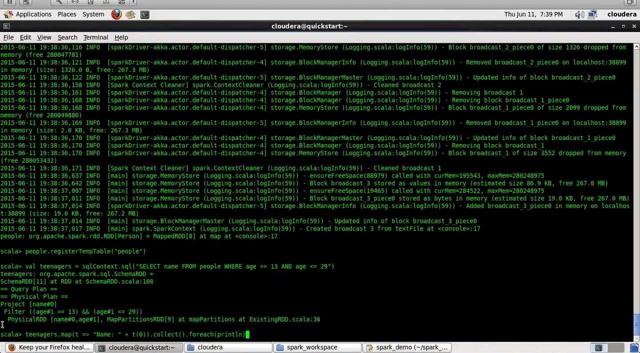 whatever was the actual file has become available as a table and guys just focus on this. what is it? what is it? pure SQL. right now, fire your query. okay, see this. you have not got any result because this was a transformation. remember, I told you until unless you do an action, you will not get any result. now you just fired a. 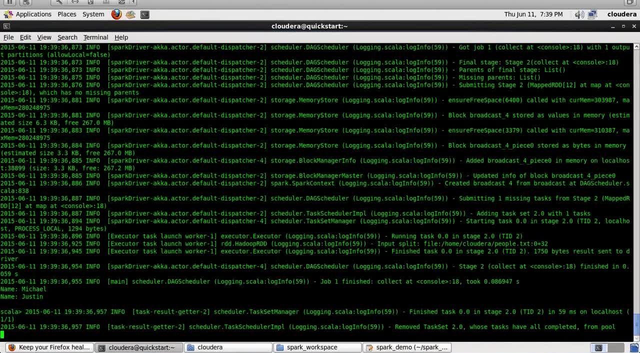 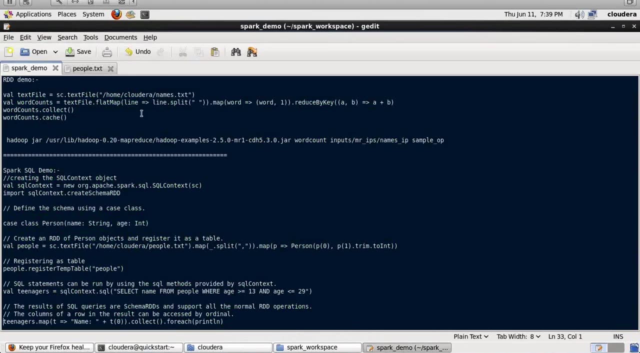 query. I'm just producing the results now. see this, Michael and Justin. let us see is it correct or not. it said: age should be greater than or equal to 13 and age should be less than and less than or equal to 13, and age should be less than or equal to 13. and age should be less. 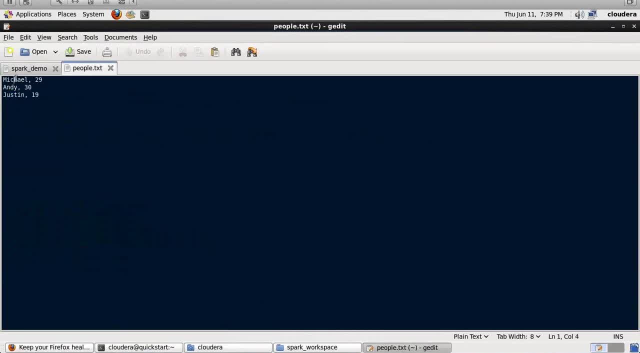 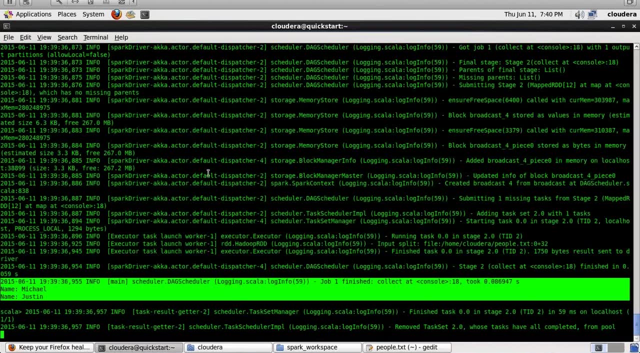 less than or equal to 13 and age. should be less than or equal to 13 and age. should be equal to 29. then Justin and Michael. they are the only ones which should come. Justin and Michael, how was it guys, those people who are coming from SQL background? I hope you are. 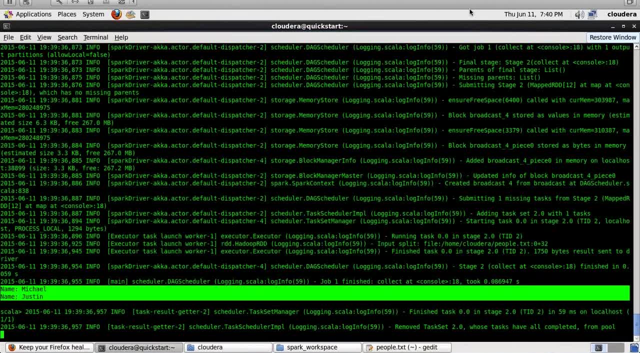 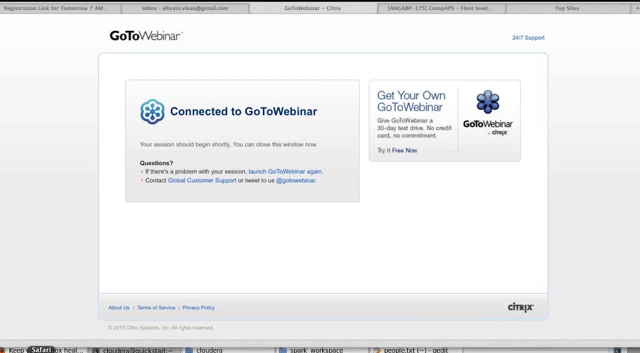 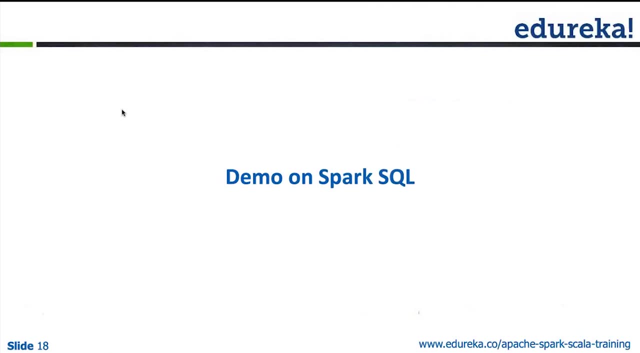 feeling a bit relieved, right? so, guys, I think that's where I would end my- you know this demo part here and would quickly go back. so this is where my demo ends. those guys who have a hurry- probably you can, you know, just continue. only my request is: please do fill. 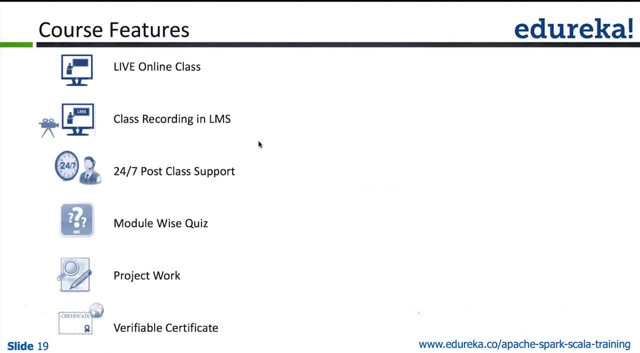 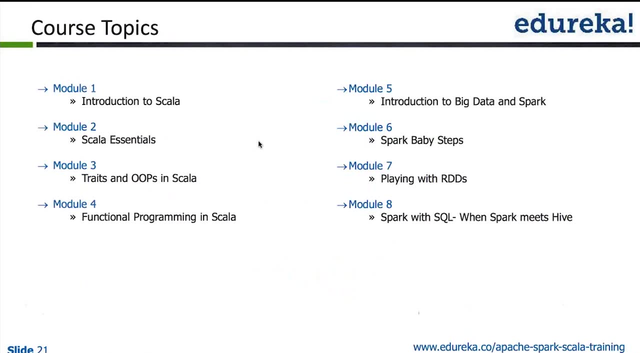 the feedback. however, I just have to tell you a bit more about the coverage of the course, which I would quickly tell you you know here. so we have divided this entire course in 8 modules, guys, and we understand that there are people who are new to Scala. so in the 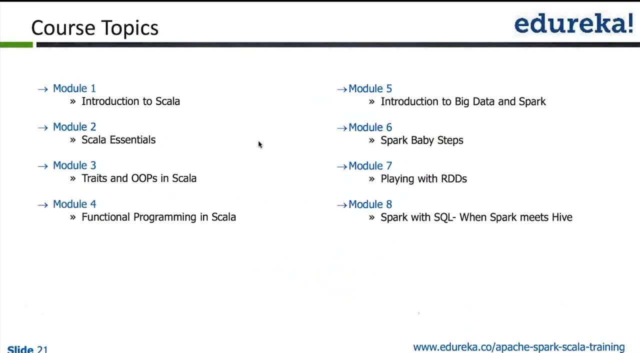 first course. we have divided this entire course in 8 modules and we understand that there are people who are new to Scala. so in the first course, first four modules, we are going to talk about Scala. we are going to cover this entire thing in Scala, for the obvious reasons: because the entire framework itself is written in this. 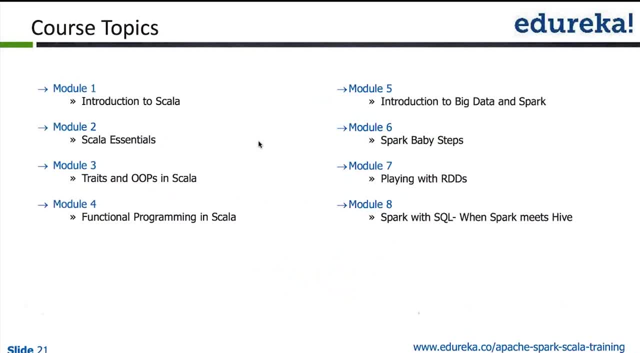 language. so it is always better if you understand this language right. so first four modules will equip you enough to work, to understand the syntax and to work with it. the remaining four modules, five to eight, basically talk about. you know, module five would be a bit overlap, like whatever we do today, but in bit more depth about introduction of Big Data. 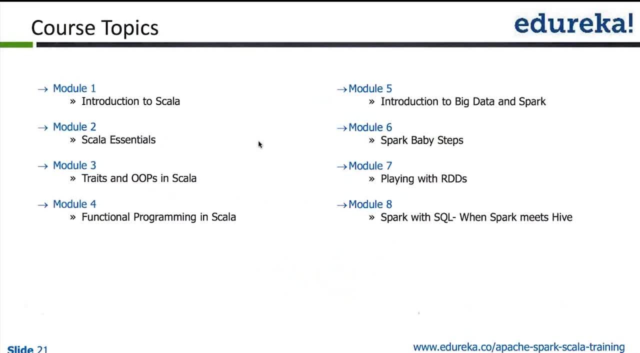 and Spark and its use cases and other stuff. module six, seven and eight basically talk about the baby steps. then developing your understanding of RDDs, creating some sort of you know operations- when I say operations it would be actions, transformations, both- and then modulate, wherein you will be seeing: you know Spark, SQL, and then you know Spark and 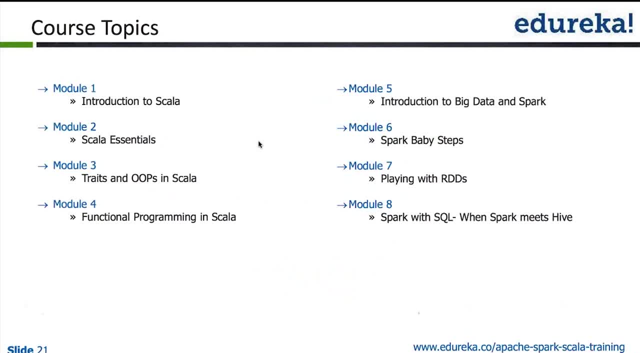 Hadoop integration. there are some more new features which are not yet available in Scala, but you can use them and then you will be able to use them. and then you know Spark and Hadoop integration. there are some more new features which are not yet available in Scala, but you can use them and then you will be able to use them.